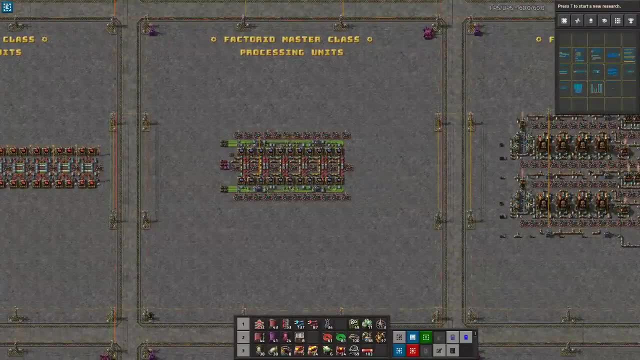 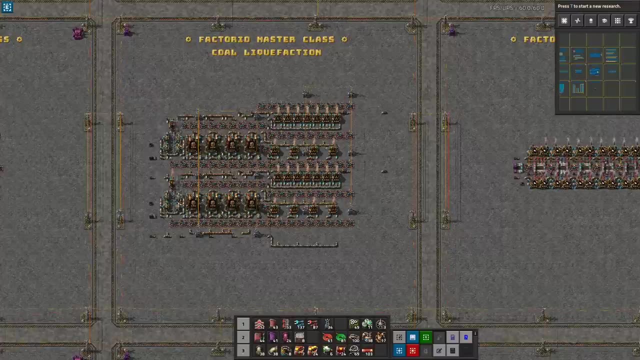 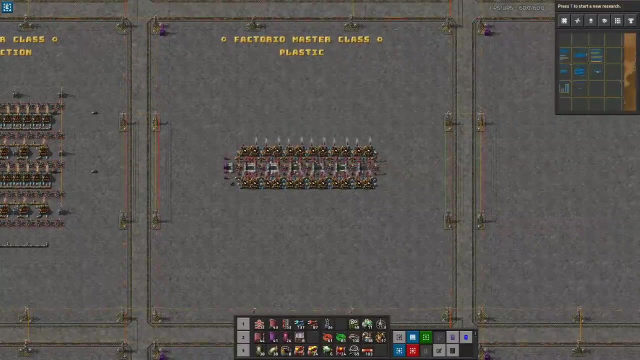 see on the runtime. this is a longer video but I have split it into something that's very basic about introduction to mechanics. So if you are completely unfamiliar with nuclear power, take this first, otherwise skip ahead. Then after we will go into a really nice design. I would call it. 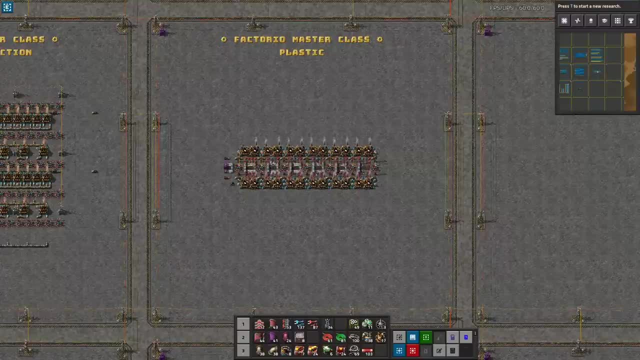 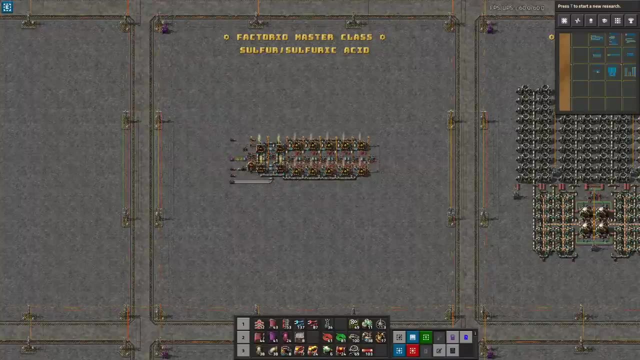 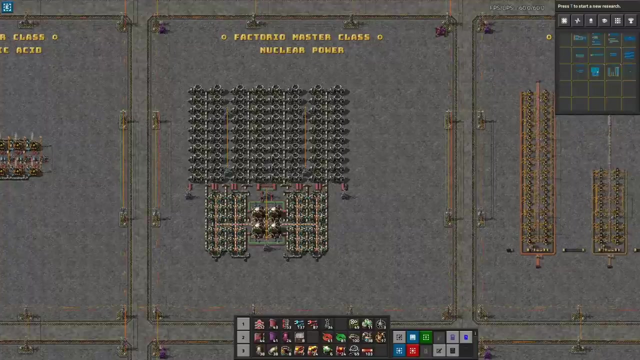 a crisp, modular, tileable design, and then we'll go into more advanced features. I will do some calculations, Prove some interesting points that I wasn't even aware of before. we did the math ourselves. and, lastly, we'll also cover some advanced topics, such as: 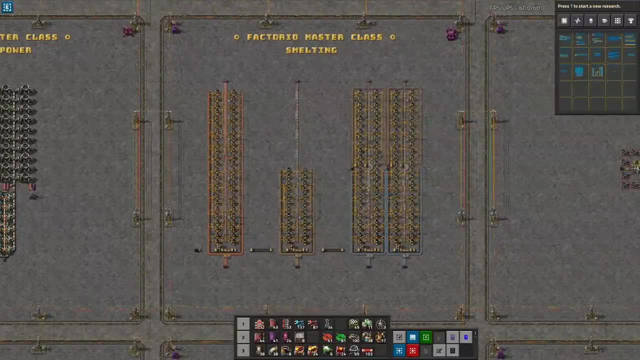 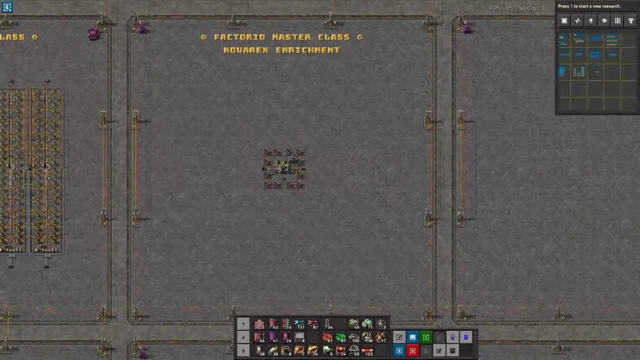 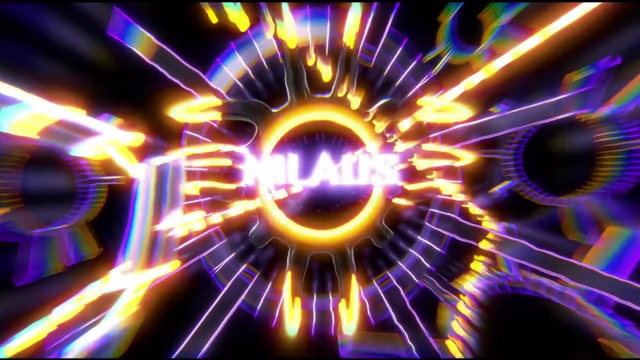 steam storage and optimal size of nuclear power. That's a lot of things in one tutorial, so do feel free to skip ahead if you need to, or come back and watch some parts later. Let's dive in. First thing we are going to do in this tutorial is to take a look at the mechanics of nuclear power. 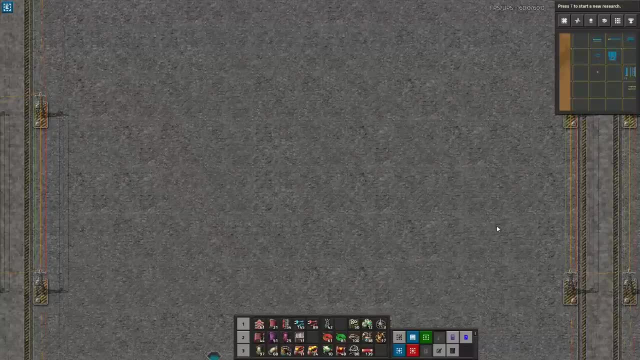 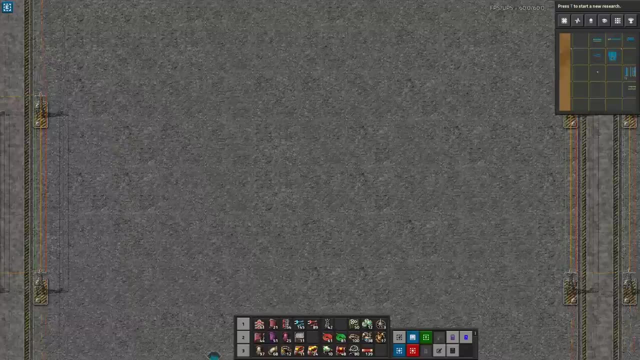 If you are already familiar with the mechanics and are more interested in looking at the design process, then take a look at the video progress bar below and skip to the next chapter. I'll be approaching this part from the perspective of a new player and try to explain the mechanics. 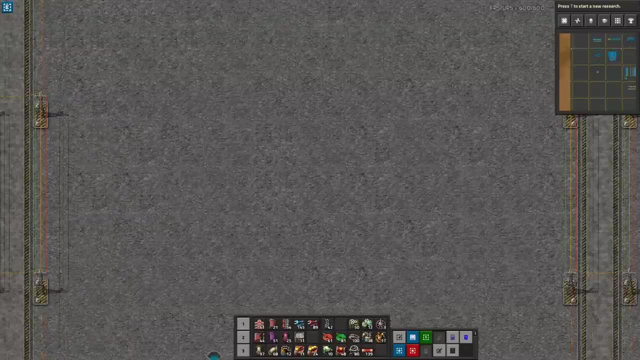 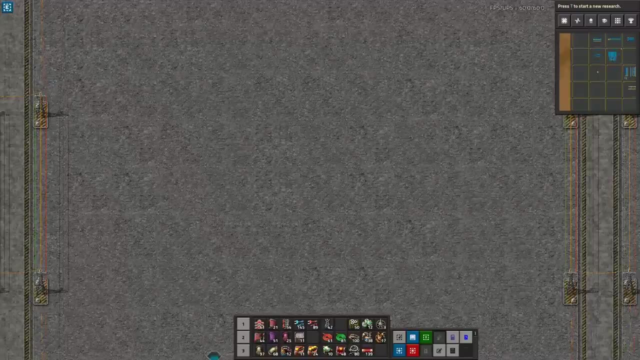 who may be intimidated by the process of converting glowing green ore into power. The first thing you are going to encounter in your game is a glowing green ore patch. I am going to make one of those. I am going to make one of those, and I am going to make one of those, I am going to 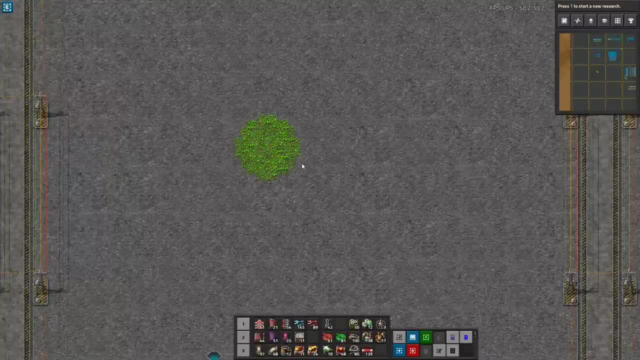 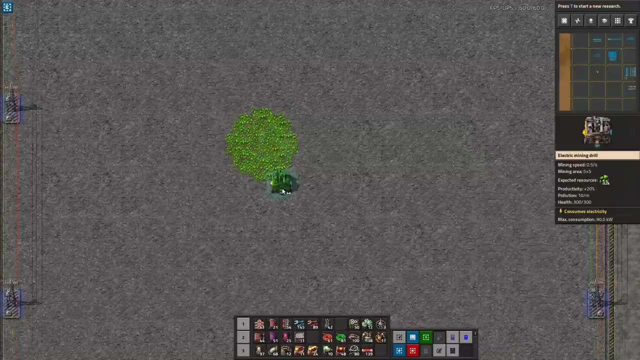 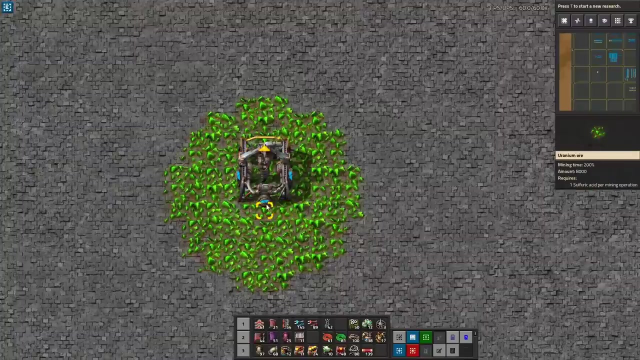 with this mod here. so here we have the glowing green ore patch, and that's where we're going to start the design from, or the explanation from. first thing you're going to need is a miner to go on here now. this miner actually has liquid inputs because it in order for it to work, 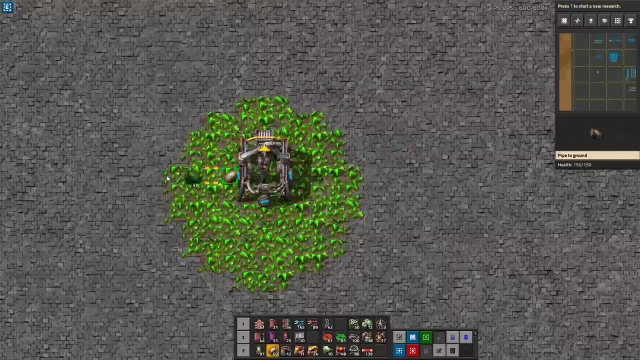 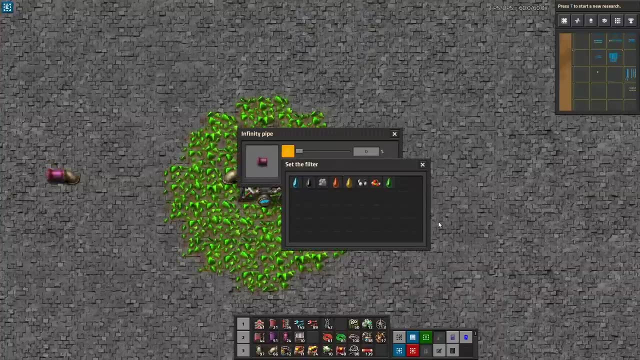 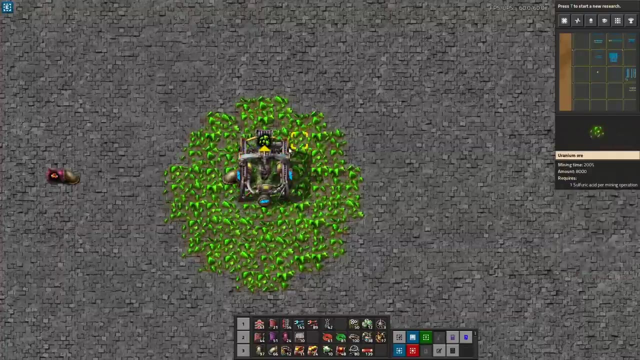 it actually requires sulfur, which is different from all the other processes i'm going to make. i'm going to use some tools here. that's part of the mod. this one is sort of crafting this for free and you can see that it is working. the one and already now there's a couple of things that you 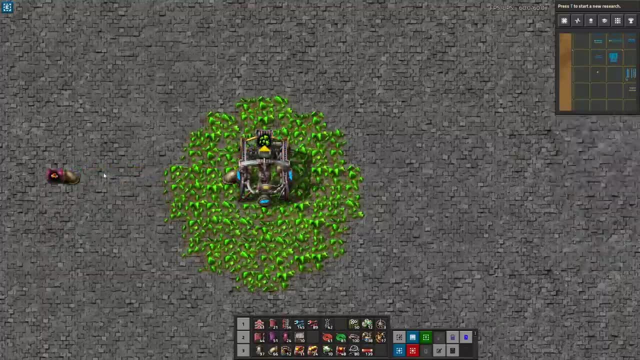 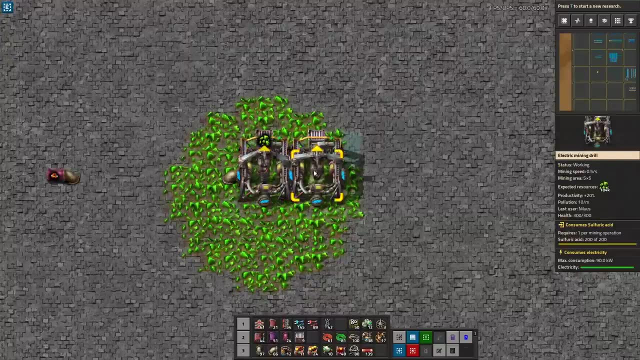 that are different. first of all, you need sulfur getting in, so you need to make a design for how to get sulfur into all of them. if you make them next to each other, the sulfur will process between them. it also goes that way. so as long as they are connected with these inputs, 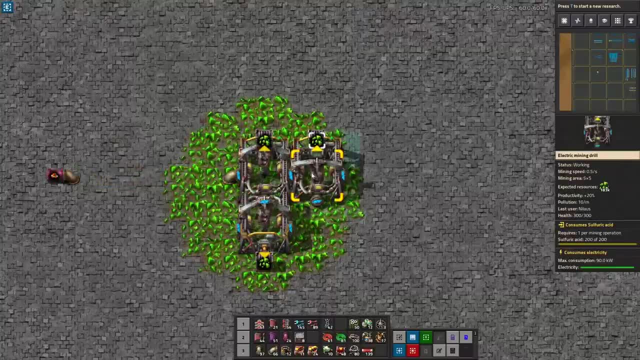 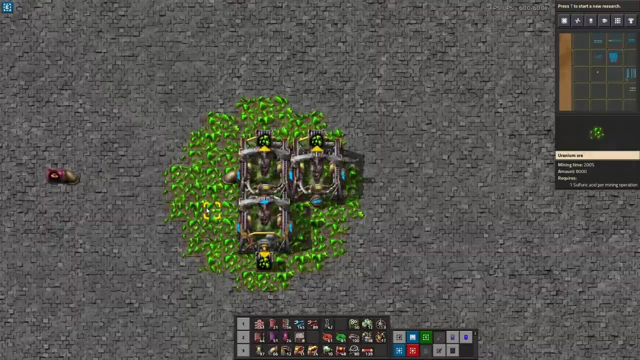 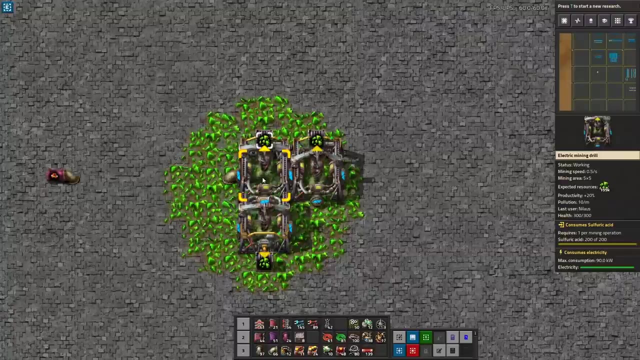 outputs, then the sulfur in one will spread to the other. the next part to keep in mind is that the mining time says 200 over on the right hand side. this means that it takes twice as long to mine this as it does to mine from a copper or iron patch. that is also something that to keep in mind. 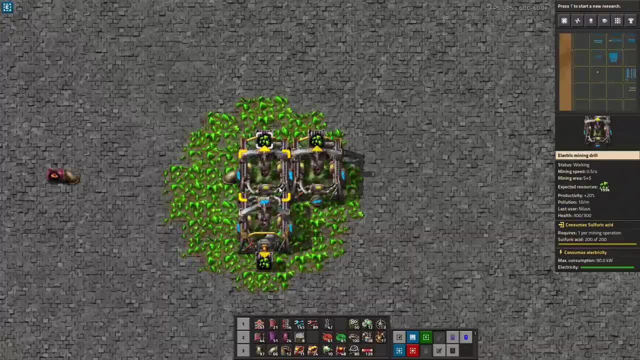 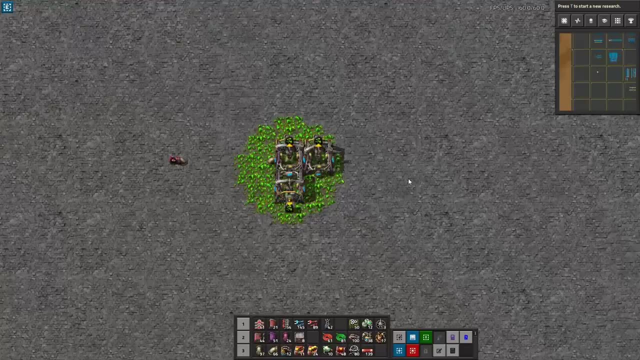 because when you just stamp it down, you will notice that it's actually not getting very much, and that's because you're basically you're getting exactly half of the yield that you would normally get. the next part: you now have some glowing green uranium ore. what are you going to do with it? 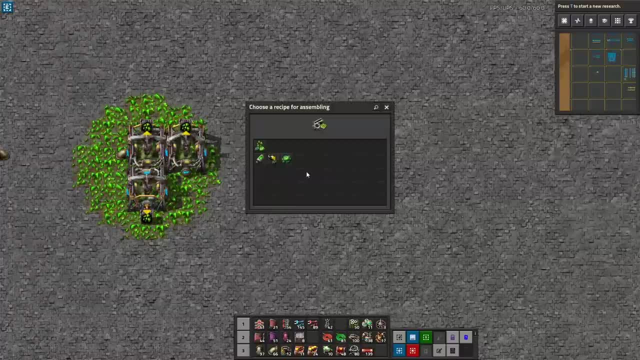 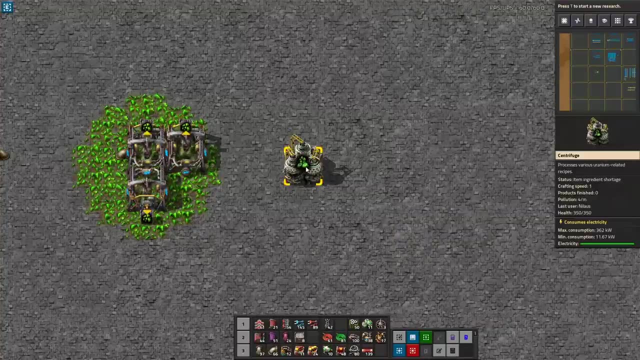 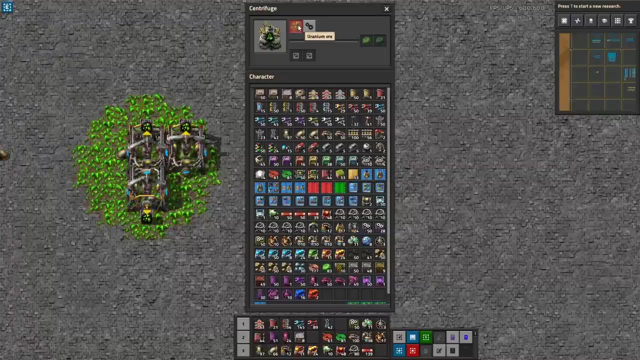 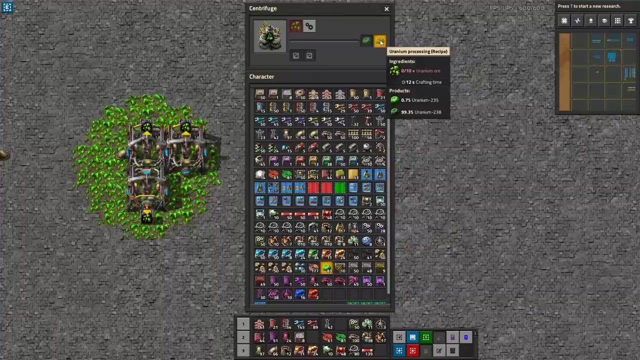 well, there comes the next process. this is in a centrifuge and you go into a uranium processing. this is the recipe that requires blue science, so it is available pretty much in the mid game. this process takes bad. ignore all my junk inventory. the process here is 10 uranium inbound and then you get some really weird. 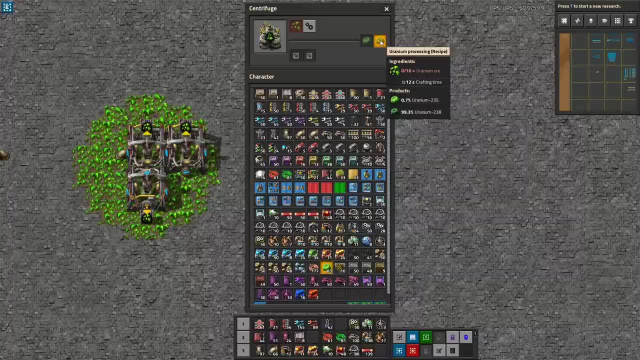 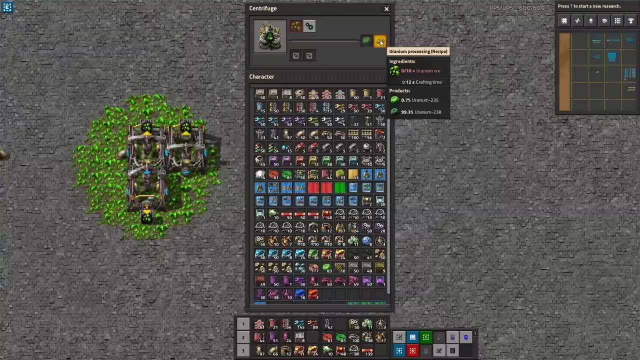 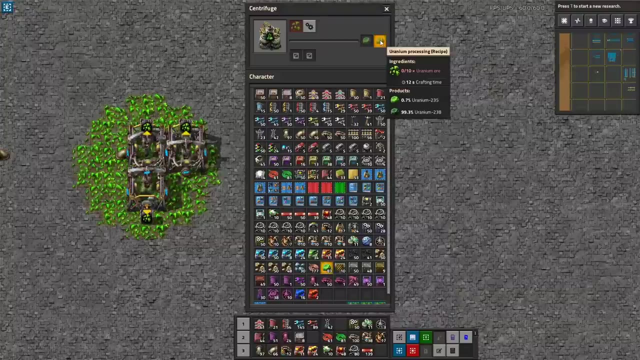 yields here: 0.7 of the uranium 235 and 99.3 uranium 238. this is usually called bright green or light green and or useless and useful green uranium, because the core of what we need is the uranium 235. this is what we used to make the fuel from. the uranium 238 is used for ammunition and 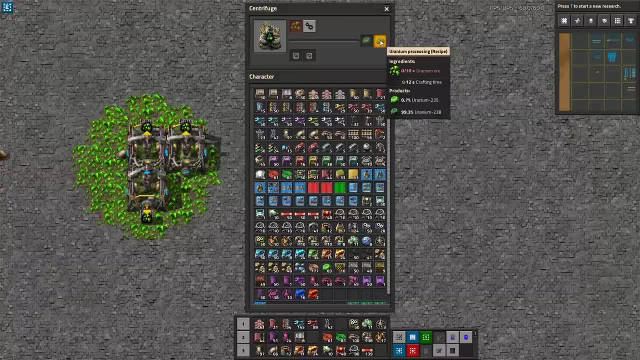 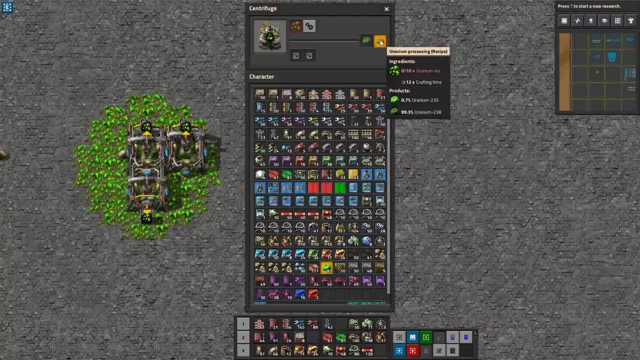 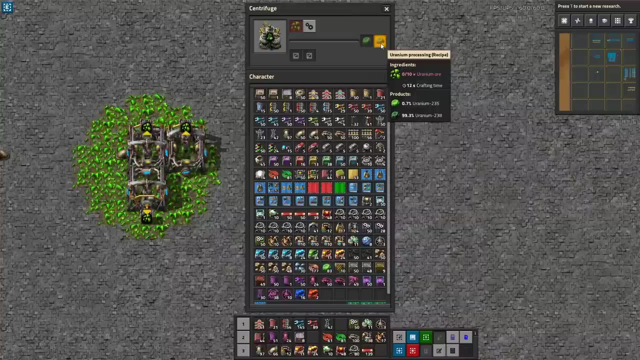 then a few other things as well, but that will. you will have way too much uranium to make the fuel from these- uranium 238- and not enough you uranium 235 in most cases. so what this basically means is that you're going to need a lot of mining to get some uranium 235 and because it is a 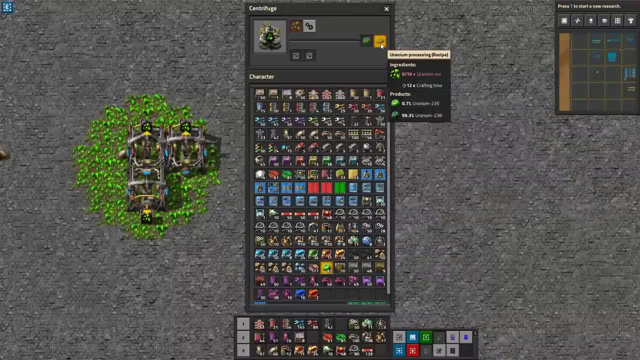 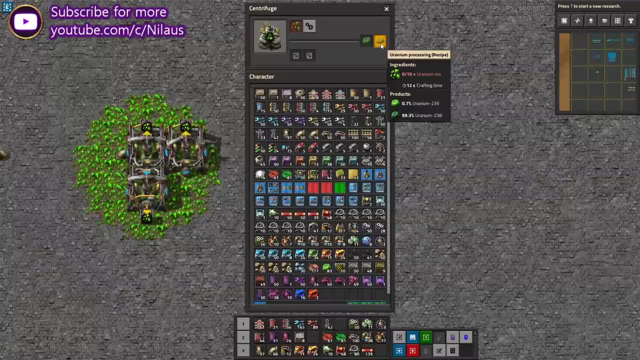 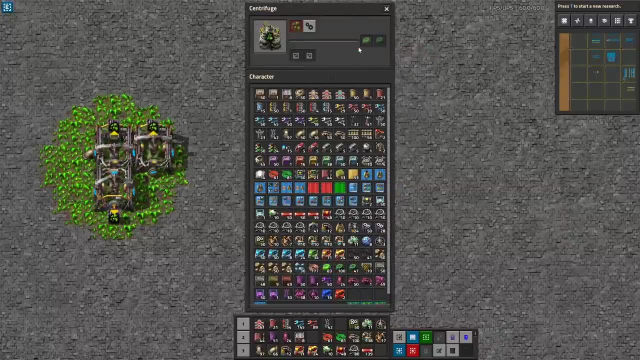 low yield and it's a random process. with a random process, then you can't really rely on exact numbers here. you will just basically, once in a while, get one and stockpile all of the uranium-238. the process now continues. you have generated uranium 235, bright green, and you want to convert this into something useful. 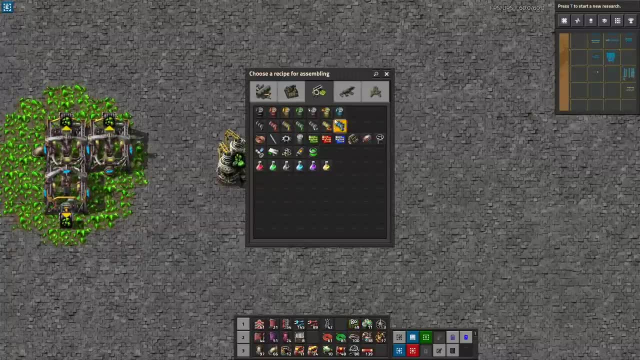 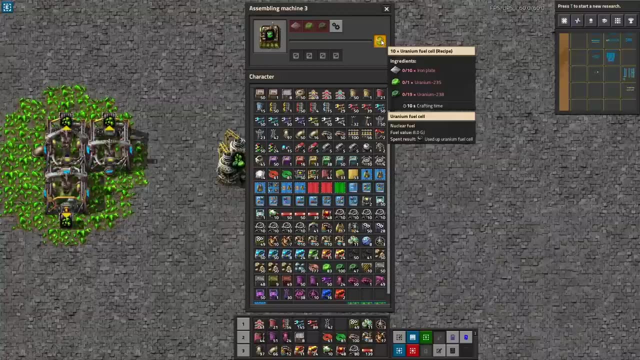 and that useful thing is uranium power or uranium fuel cell. so that's the recipe we need. it takes one uranium 235 and outputs 10 uranium fuel cells and uranium fuel cells. that's what we start burning in the uranium process. so let's switch over and explain the actual uranium process. 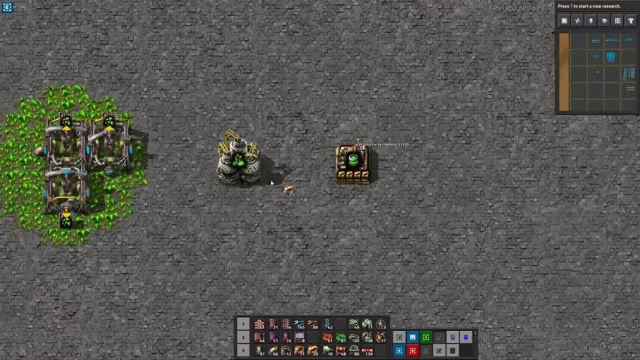 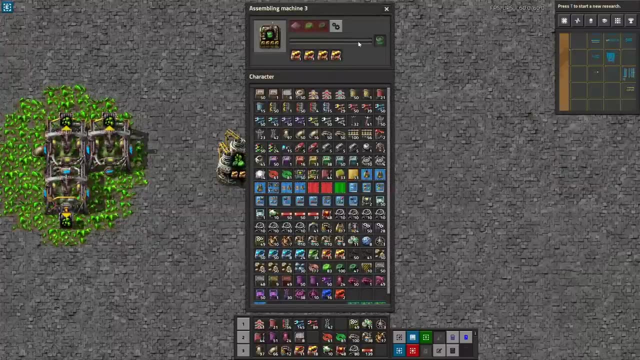 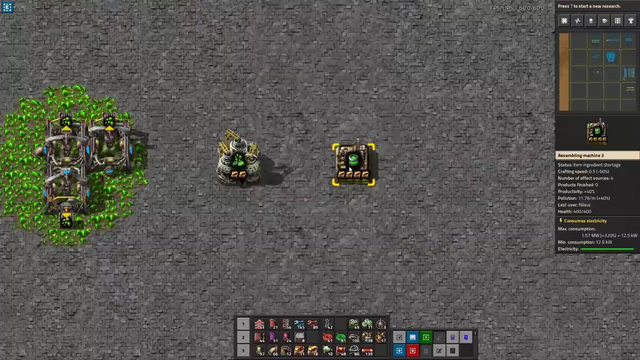 it is worth mentioning that this process and this process can be moduled, and i would highly recommend modulating it, especially especially this one, because you take your very precious rare material, you uranium 238, 235, and why not get an extra 40 or 16, depending on your tech level? 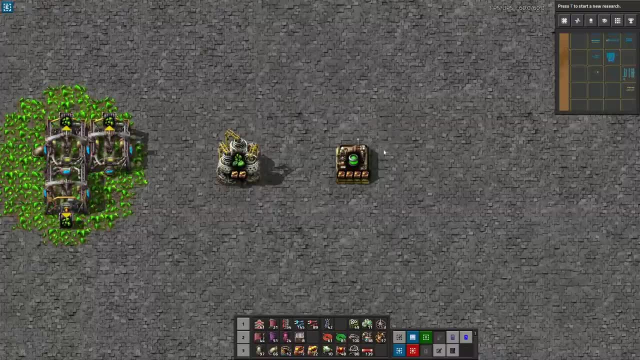 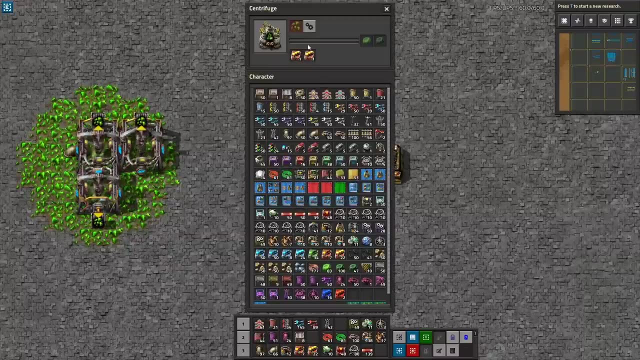 this extra 16 yield if you can. this process well, depends on whether you have a small mining pattern or a small mining pattern, and you can do that by using a small mining pattern or a big mining patch- whether you feel you need this, and power wise as well. so now let's do a 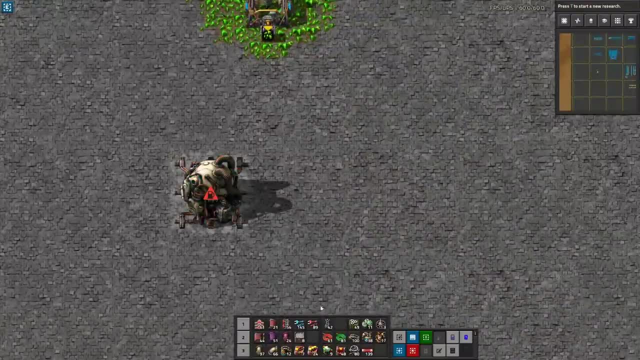 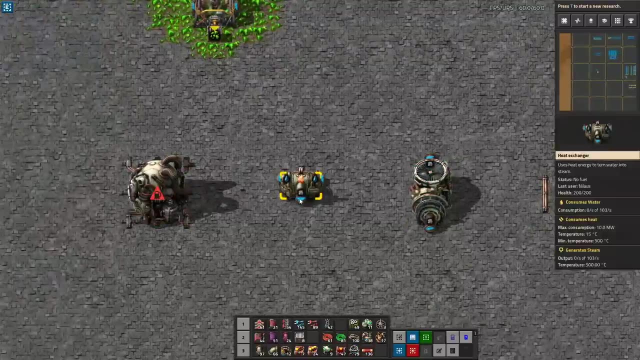 switch and take a look at the nuclear process, because there are several different engines or entities that are part of this process and i will explain how they work and how they're connected. we start with the nuclear reactor. this takes uranium fuel. it can only take one type of fuel. 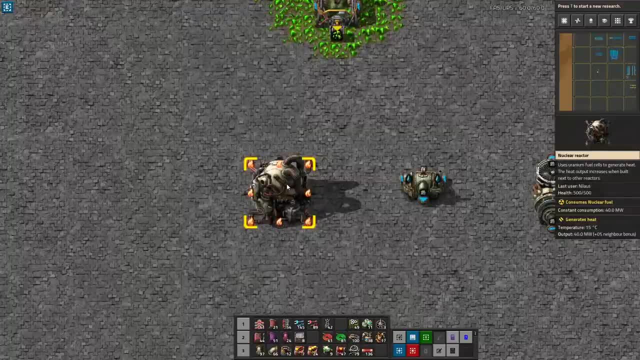 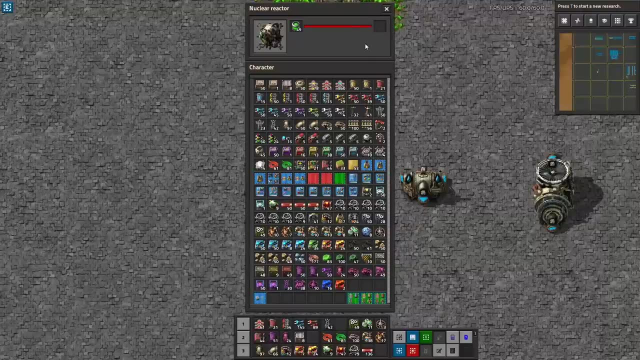 and that's the uranium fuel. it will then generate a lot of heat. let's just start by putting something in here, and we're going to start with the nuclear reactor and we're going to start with the uranium here, just to show what's going on. this one will burn. it'll take 200 seconds to burn one fuel. 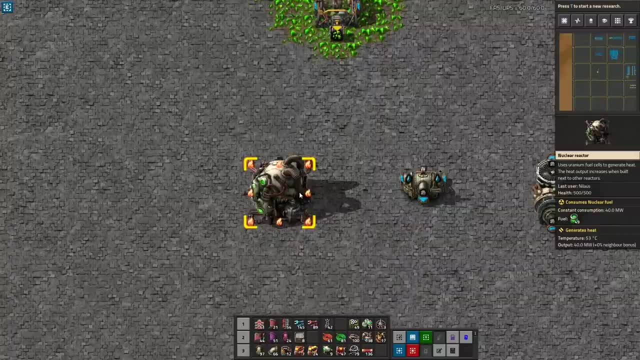 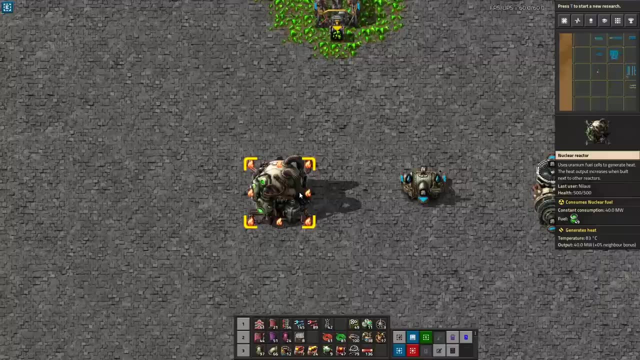 and this is completely independent on whether whether there is a draw from this. so, unlike steam engine, there's steam power where coal is only consumed. when there is a draw of power from the steam turbines, not just dimensions, then in this case the nuclear reactor will always work. so we're going to start with the nuclear reactor and we're going to start with the nuclear reactor. 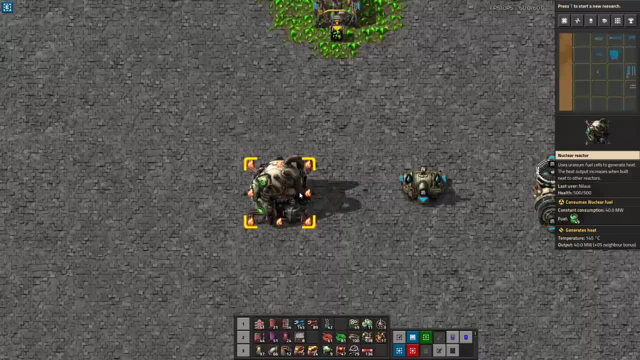 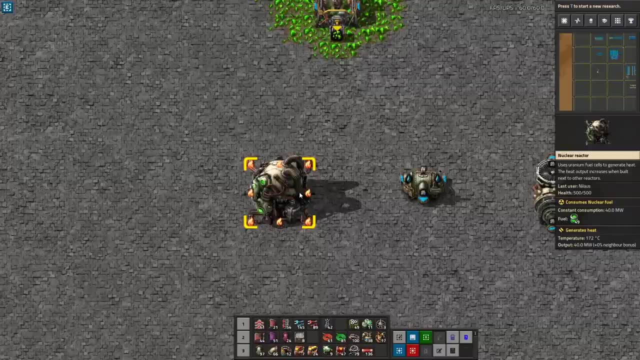 it's always on. so as soon as you start it up, it will consume one fuel cell every 200 seconds, and that's just the way it is. you can do some clever tricks with circuits and trying to insert, export, and, but i'll get back to why i don't think that's a good idea. for now we are going to just 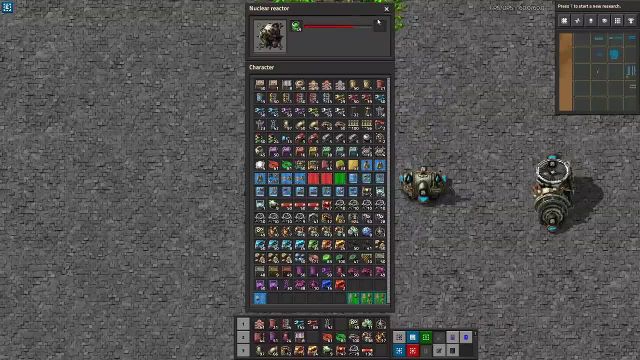 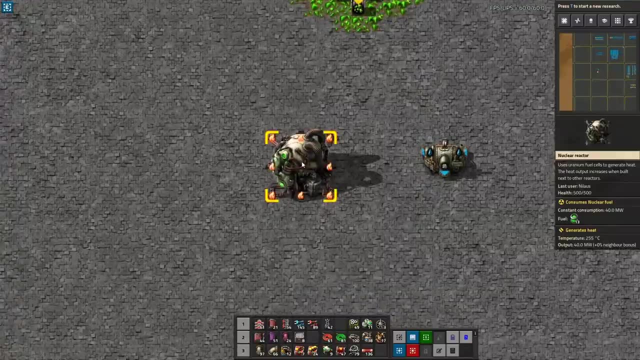 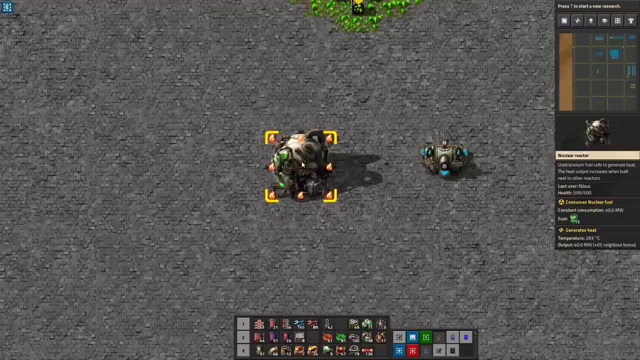 say, every reactor needs 200, or needs one of these fuel cells every 200 seconds. we're not going to have to wait and see this mikä opening the doors all the way up, and let's hopefully we'll see for sure that it will not end up like i'm seeing now. this has a weird, very weird. 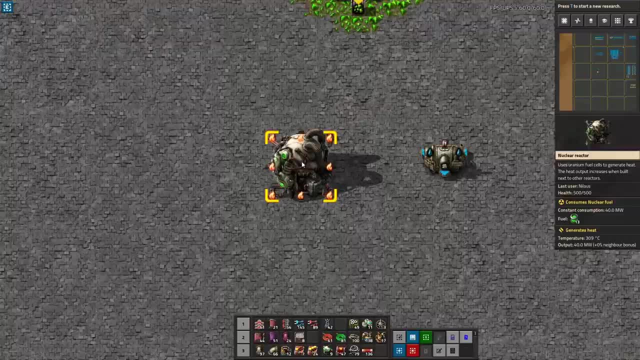 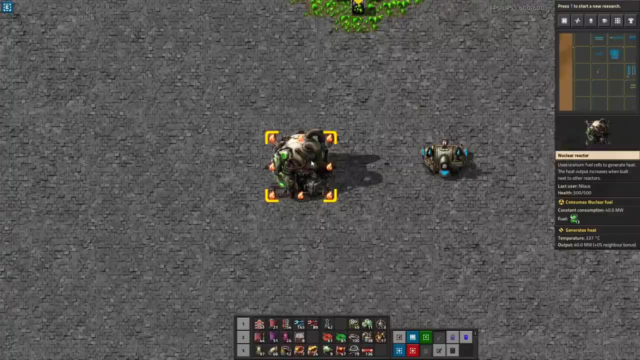 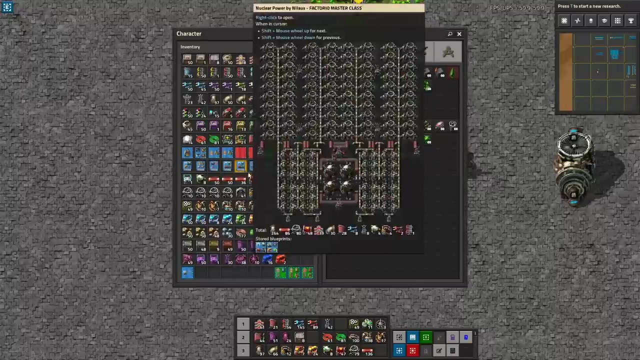 mechanic. you can see this one is producing 440 megawatts, which isn't actually a lot. you can also see a temperature is slowly increasing. it'll only start it outputting heat when it reaches 500, well above 500. so this has an interesting mechanic: that if they are next to each other, 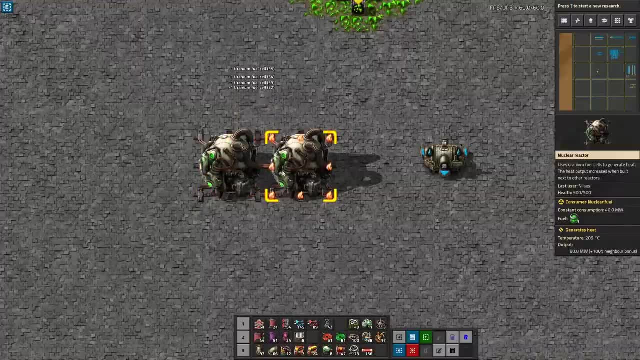 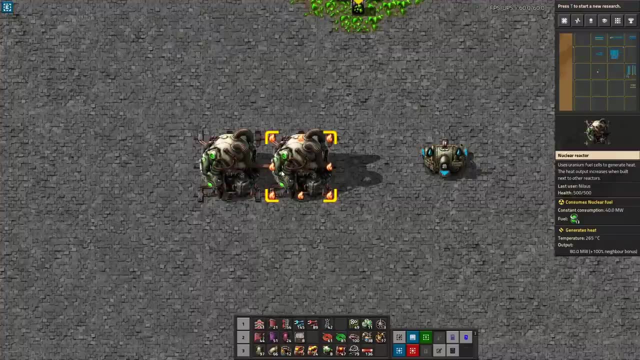 like: so they will get a neighborhood bonus. does it say here: yes, it does it say: output is 80 megawatts, because it gets, it gets 100 neighborhood bonus. so now, when i have two, instead of generating 40 plus 40, they are generating 80 plus 80. so by doubling this, by putting two next to each other, 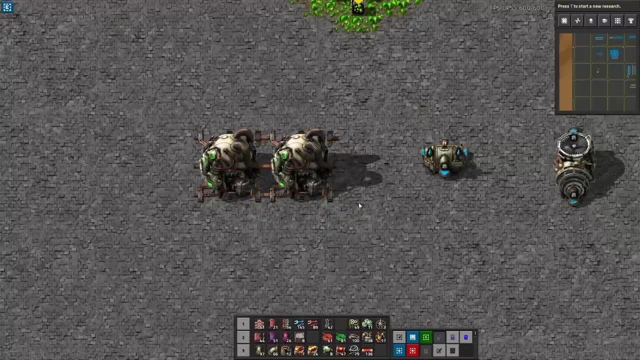 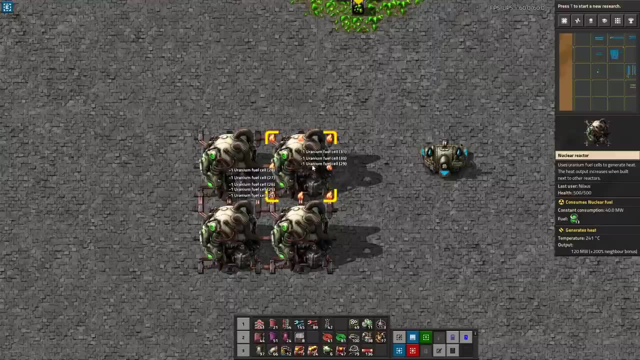 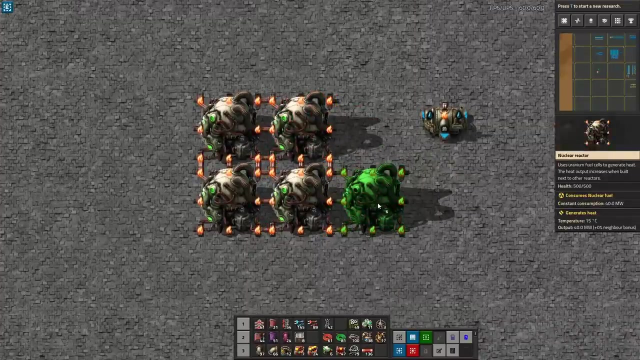 we're actually getting an output of 160 from these and if i go like this, for example, then you can say that they get 200 negative neighborhood bonus. neighborhood bonus only counts if they are evenly aligned. you can't do it like this and do it diagonal. it has to be. 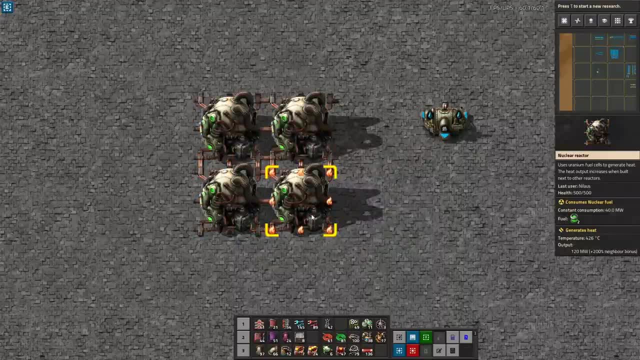 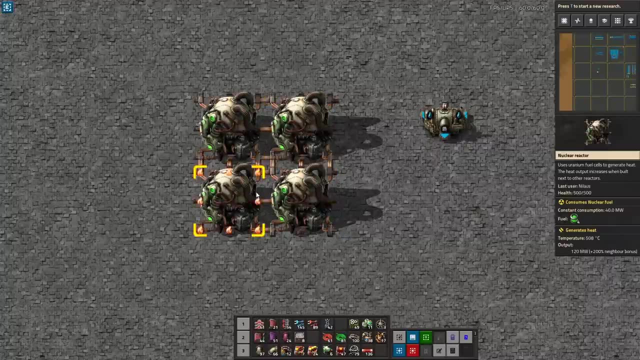 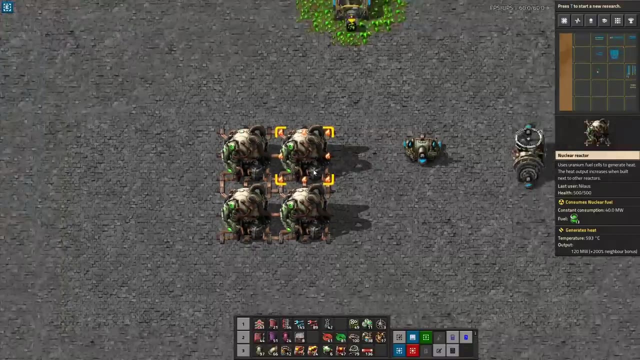 the full face towards the full face, and then it works and as you can see, you can see that. you can see that this one gives us. now each of these is producing 120, so this design here is 480 megawatts of power, and that's going to be the unit i i will use. there is a kink that if this one gets destroyed, it'll 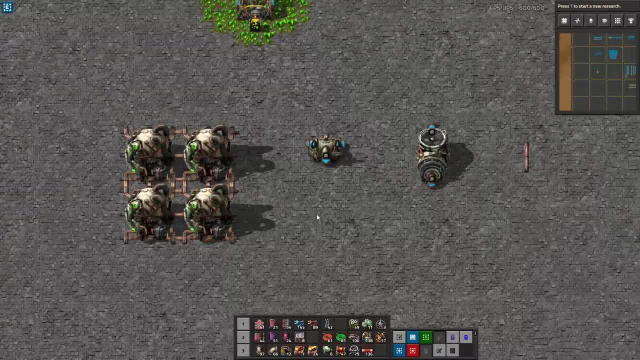 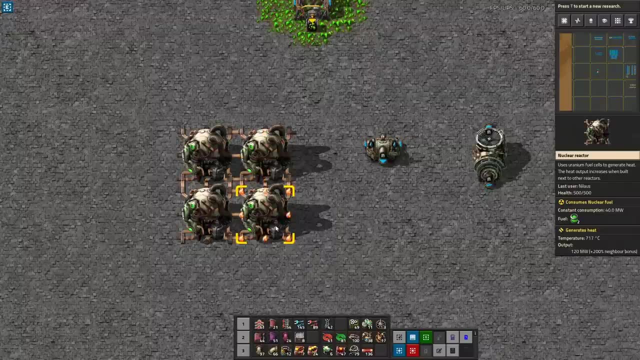 blow up, but it happens so rarely that i don't actually think i've ever seen it. so what happens with the power that is generated? these are now up to about 500 and it'll just output some power. the power that is generated it'll blow up, but it happens so rarely that i don't actually think i've ever seen it. so why are we even talking about one and one? 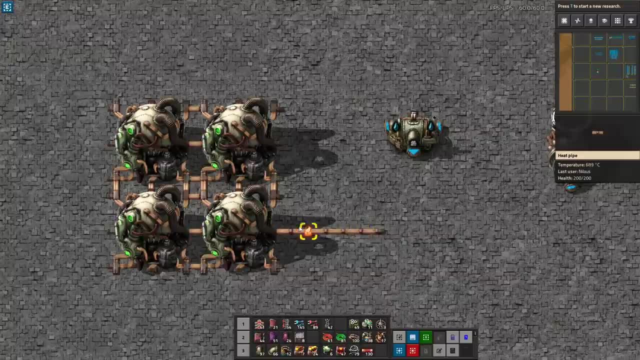 that's not quite a lot of time to do it. the power that's generated determines if the damage will be going to increase, and that's only true if the damage of the iron is reduced or not. you can see here there's a little flame. it outputs through these heat pipes. you can see. 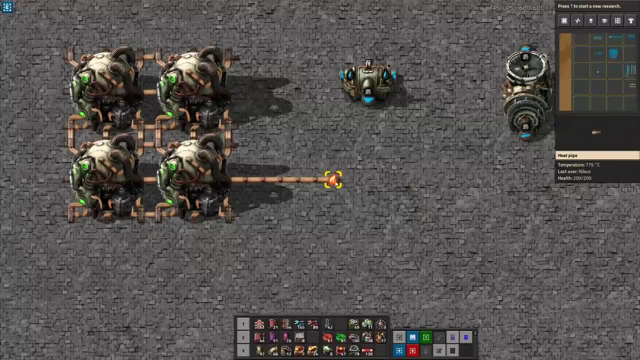 the temperature increases in the heat pipes, and the heat pipes are kind of like belts or pipes. the heat pipes are kind of like belts or pipes, except there is no underground. so once you build this, you have to work around the fact that there ground. so once you build this, you have to work around the fact that there are no underground. 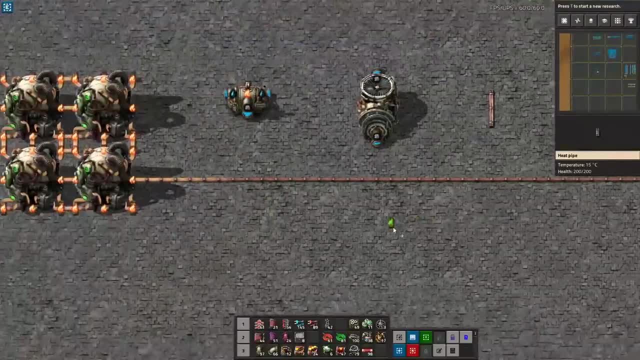 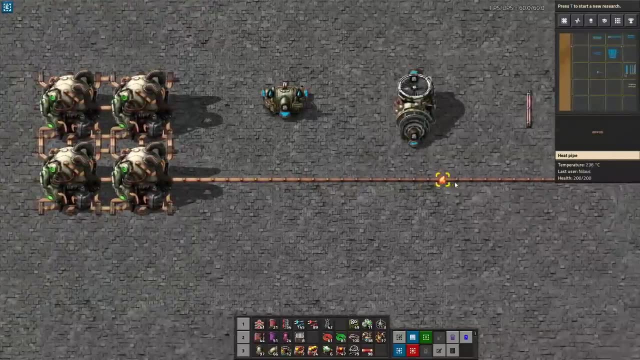 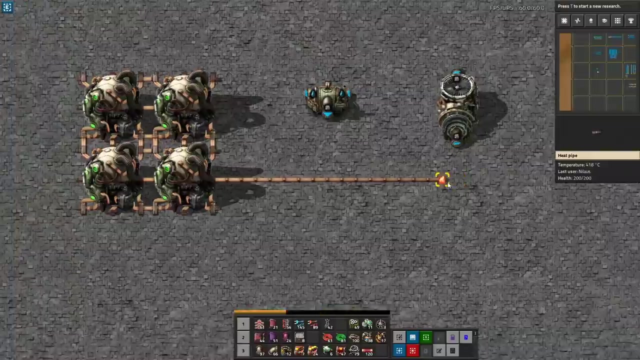 heat pipes and additionally, if you build it very far, heat does not transition very well down the line. it will of course dissipate down the line, but if you also draw heat from it at the end you don't get to so much. so you don't want to make like really long strings of this because you 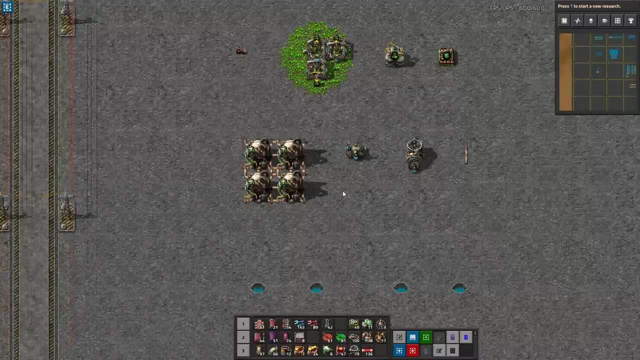 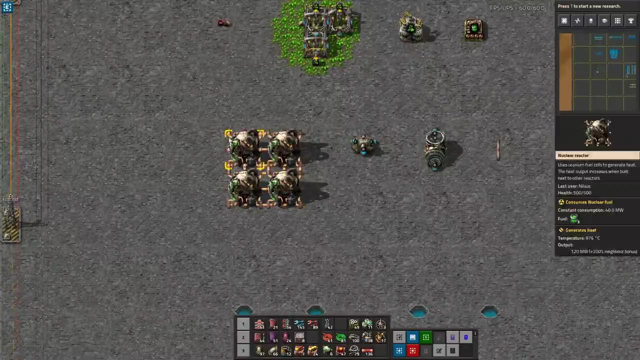 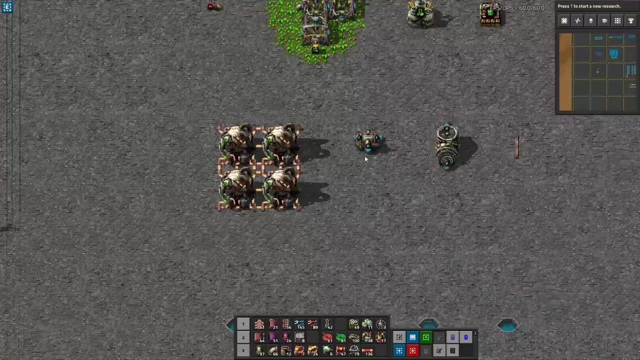 actually end up in a situation where, if you're using all the heat transmitted, you can't transmit the heat far fast enough, far enough away it's. it's mainly an issue if you try to make something like really big designs, which is again and reason why i argue that build more smaller, modular builds. 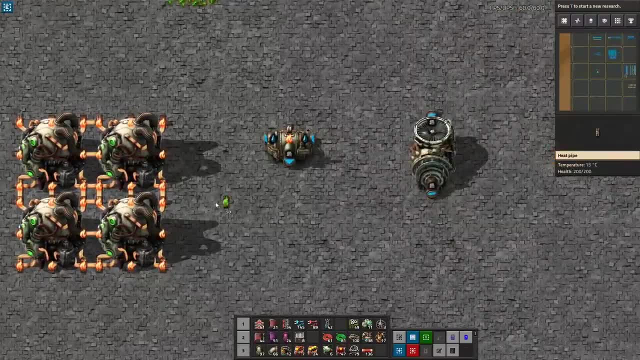 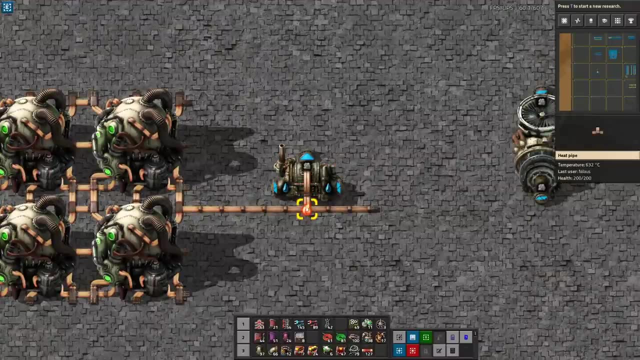 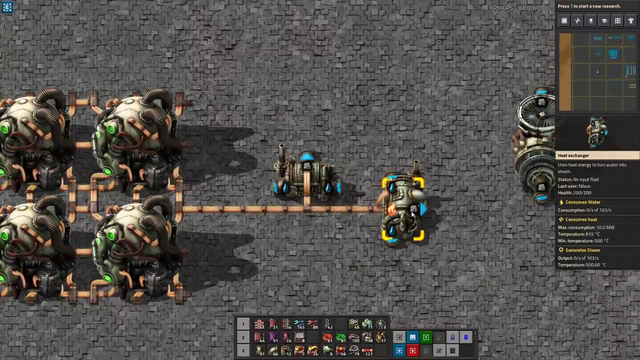 so we have our heat pipes transmitting and that goes into a heat exchanger. a heat exchanger- you can see this- looks like a normal boiler but it has an input here on the side, in the middle of the side, like that the way it gets the heat in. you can see the heat here is. 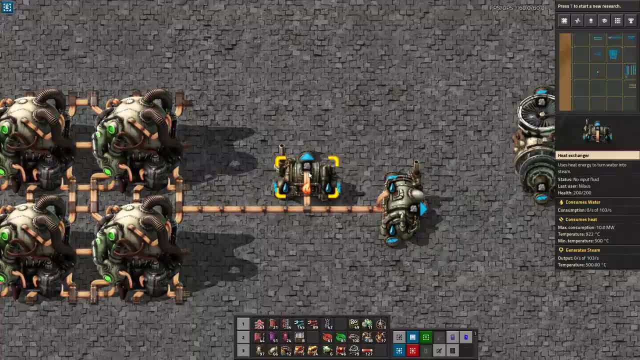 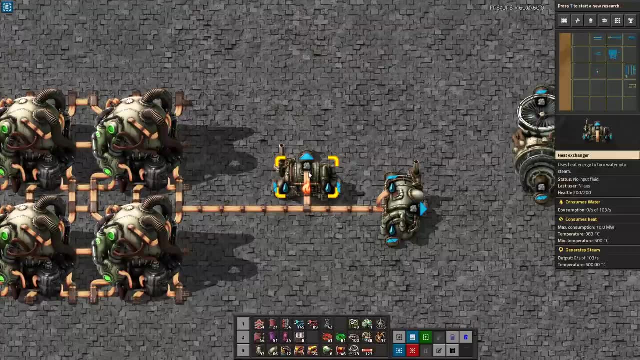 increasing up to 1000. and what it does? it's consuming water and making it into steam, and it only works when the temperature on the heat pipe here- the temperature in here- is above 500. so until it's, it means it has a startup time and that also means that if you 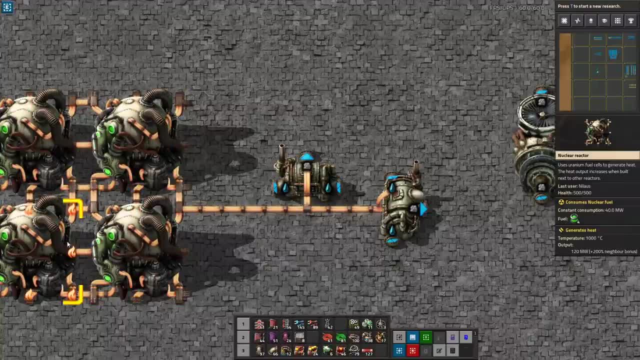 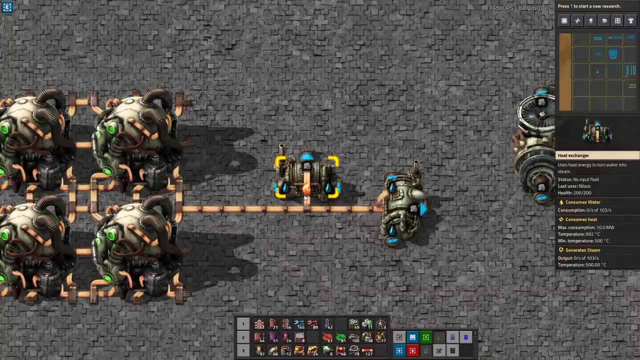 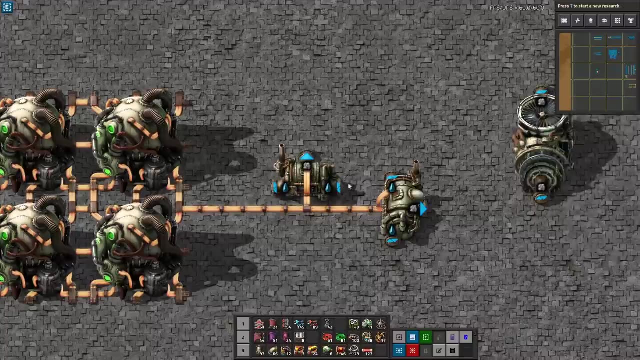 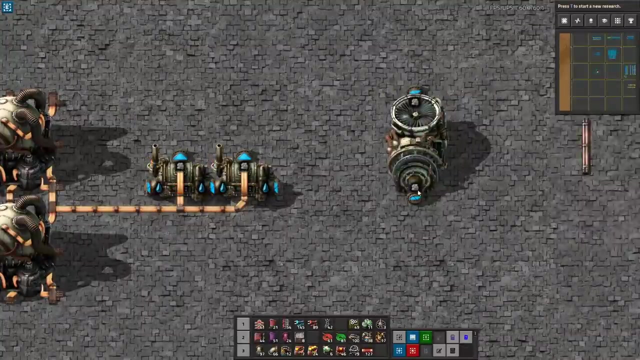 run out of fuel and even if you insert the fuel again, then it's going to take a while for the nuclear reactor to heat up and therefore the power to restart. these ones are consuming 103 water per second and outputting, so the water comes in on the side and the steam goes out. here the steam is what we use for power. 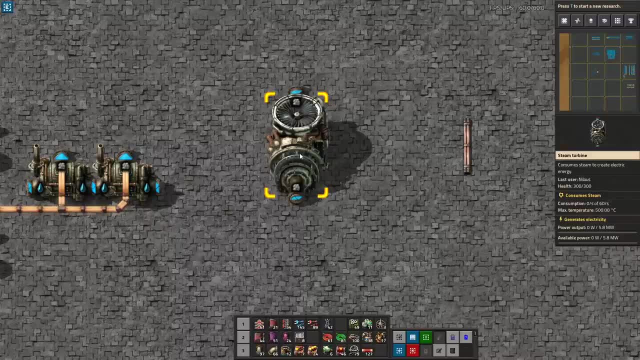 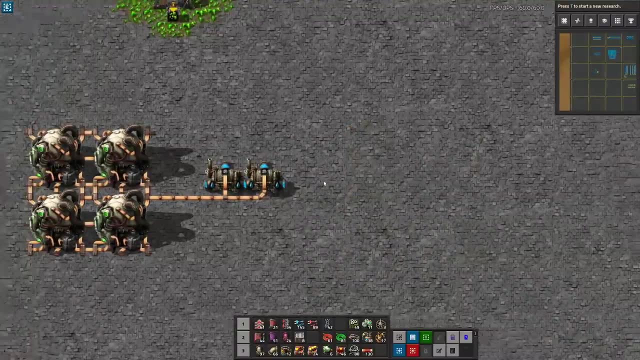 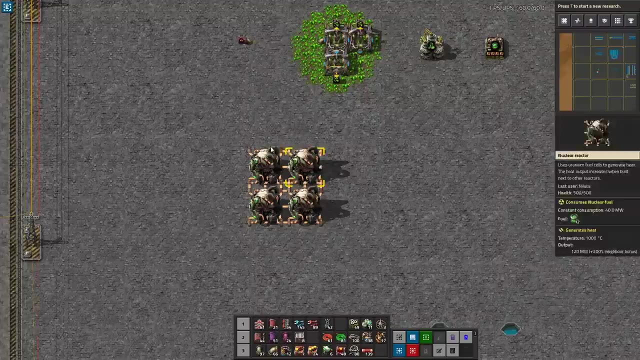 the steam is going into a steam turbine. it consumes 60 steam per second and outputs 5.8 megawatts of power. so with all these things, you can, you can start doing some calculation. if we have this part and i want to fully utilize all the 480 megawatts of power, then we do some. 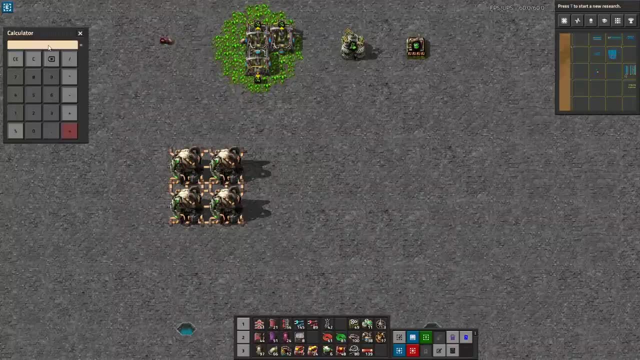 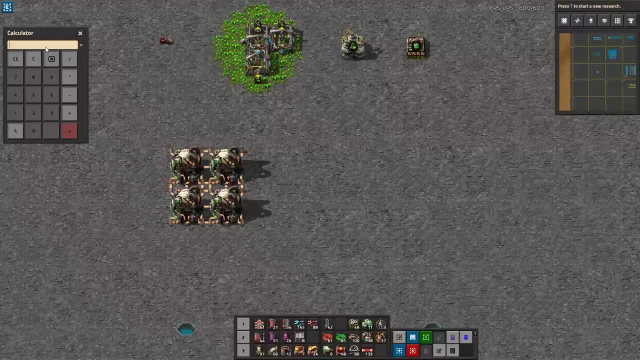 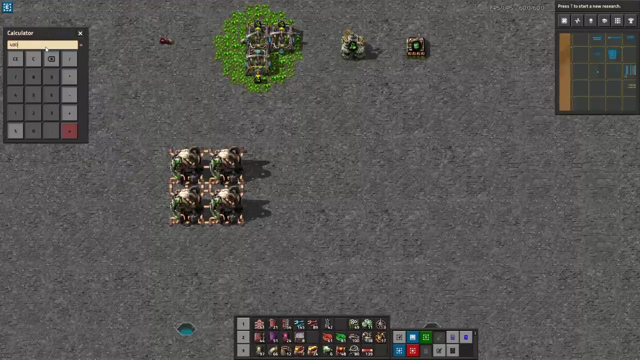 calculations. i can use my in-game calculator. this is a mod called calculator ui. it's really nice, made from my video from the community. and what are we doing? so if i have 480 power created from the nuclear reactors and i want to see how many of the steam? 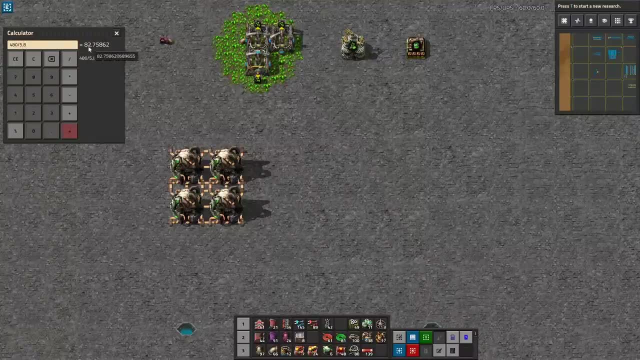 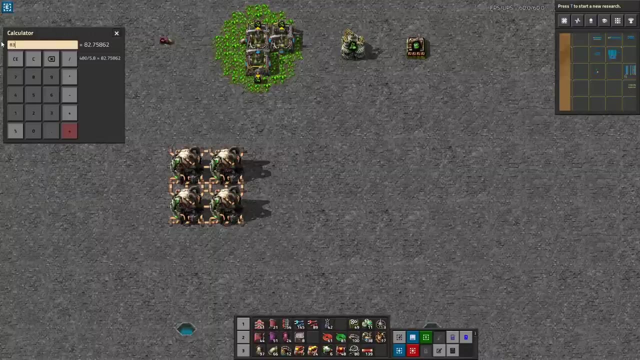 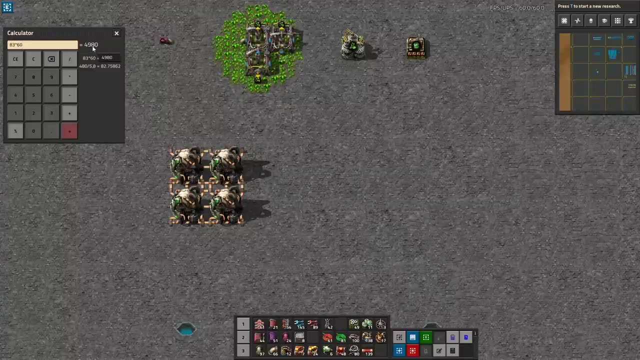 turbines i use. i divide by 5.8 and then i figure out that i need 83.. now, 83 is a really bad number, especially because 83 times the 60 steam is 4980.. each offshore pump can produce. let's take a look at the offshore pump. 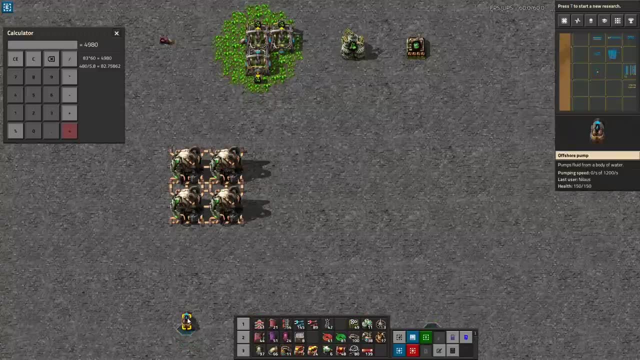 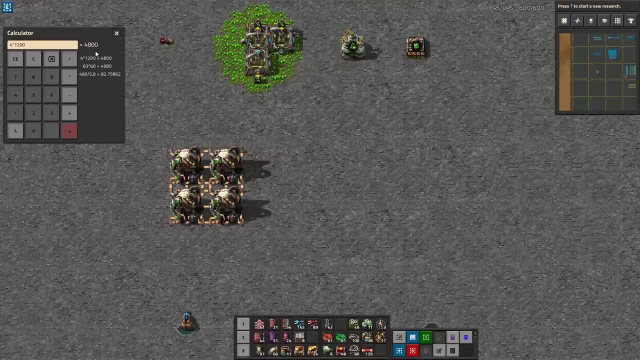 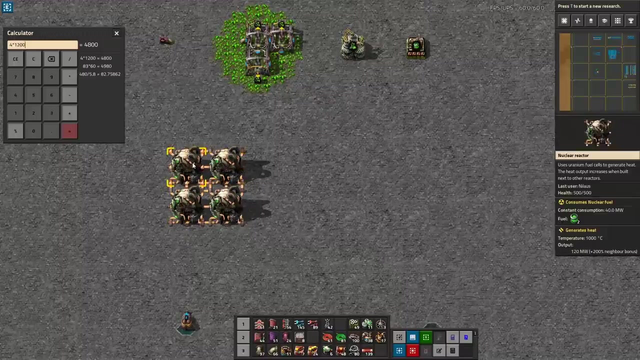 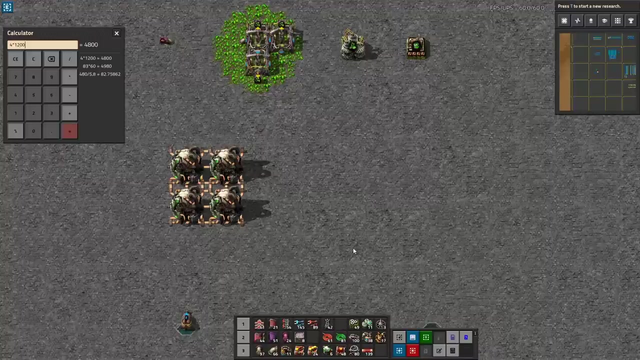 here can output 1200 per second, which would be four times 1200- 4800. so basically, what i'm saying is that, even though this one can produce 480 megawatts of power, it is really impractical to deliver, to utilize all 480 megawatts of power, because you're going to need 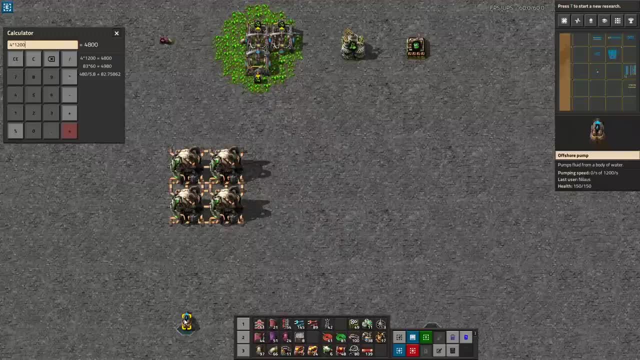 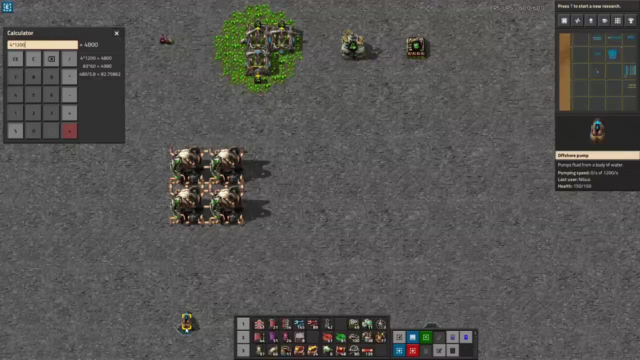 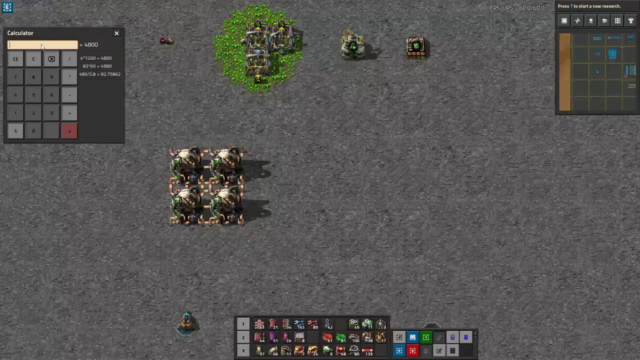 five offshore pumps, and this, the fifth one, is only very barely used, and, on top of that, something that is, uh, that has five inputs, is not really easy to design. therefore, what i'm going to do is i'm going to say i want 80 times the 5.8. 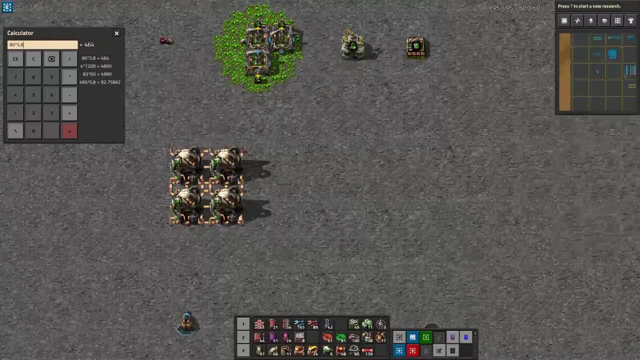 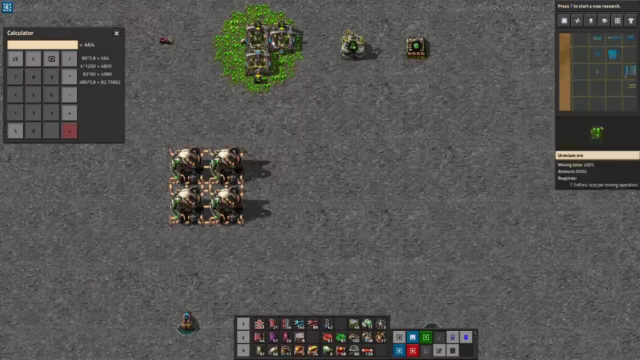 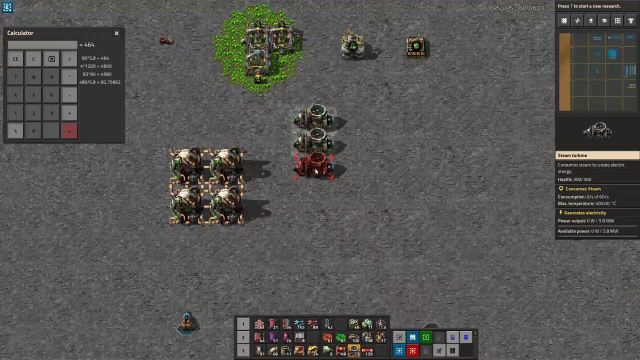 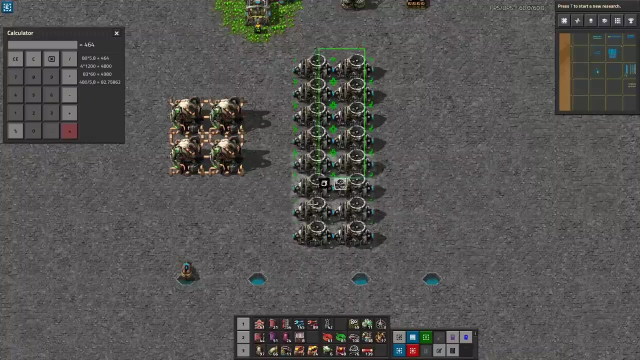 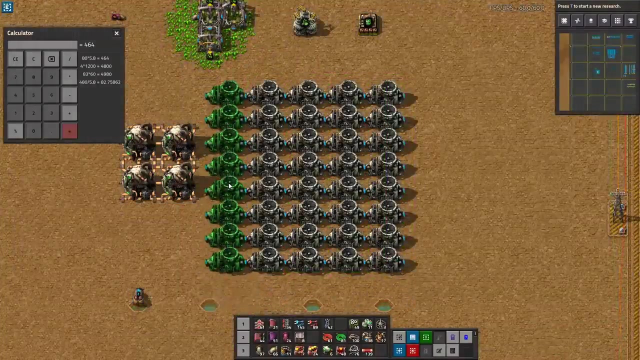 and that's 464 megawatts of power being used from here. i'm perfectly happy with that. if we then look at: now we have 80, 80 of these. one, two, three, four, that's eight, 16. it's actually not particularly practical. 40 and then double it, so that's how many energy we have. and now, if we look at this one, we have: 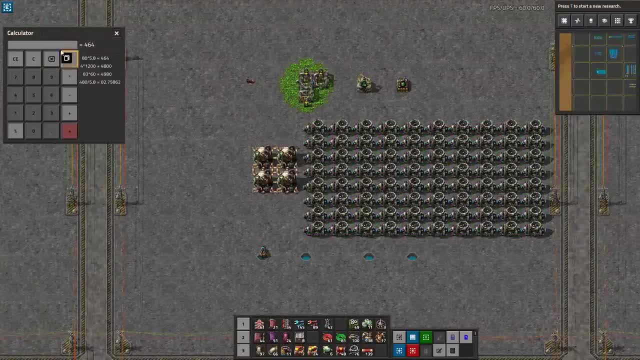 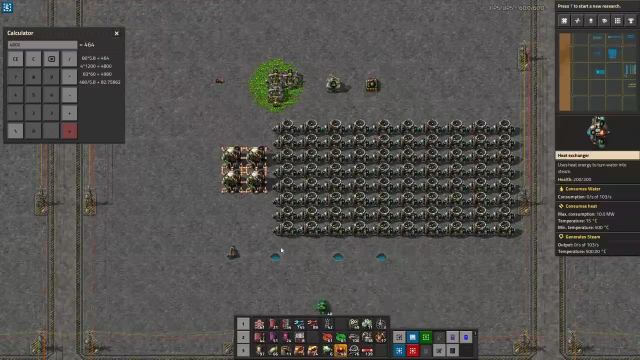 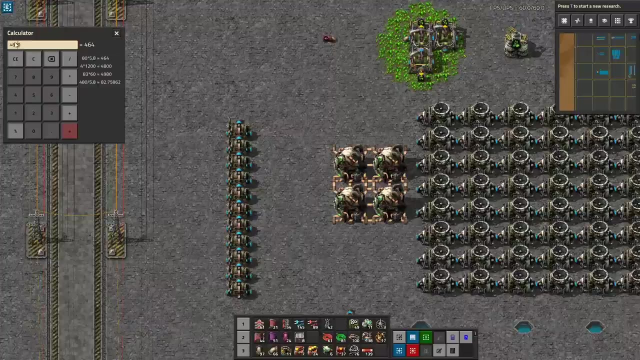 need. If I take a look at all of these, then that would require 4,800 water, and 4,800 water I need to build that in here. Each of these can do 103.. I'm just going to pretend that it's just 100.. 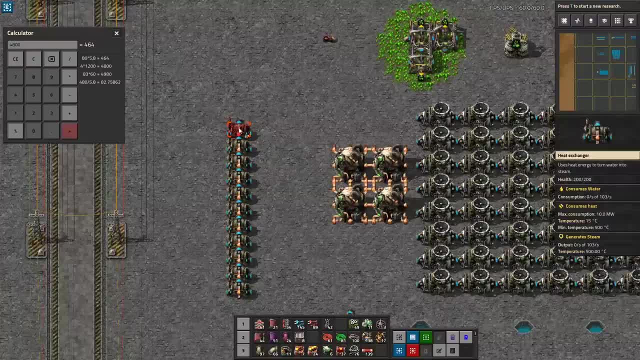 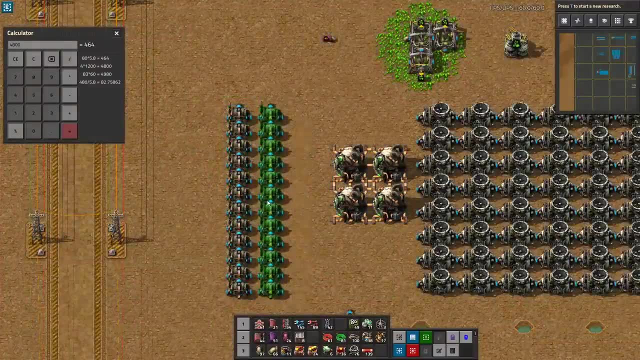 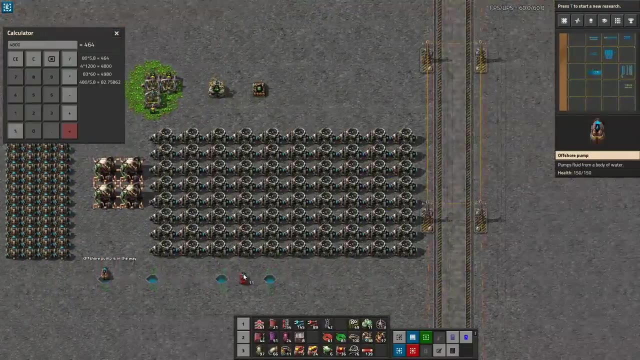 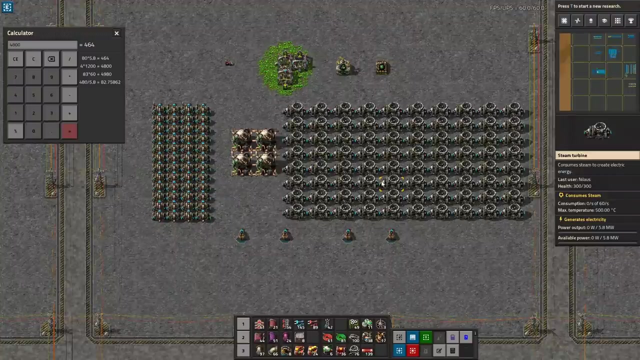 This means I need 48 of these. How many do we have? 11. And there you have it. So, if we want to, and four water here. So those are the ratios that I would propose, and this is the input for our design process. We will have to design something with. 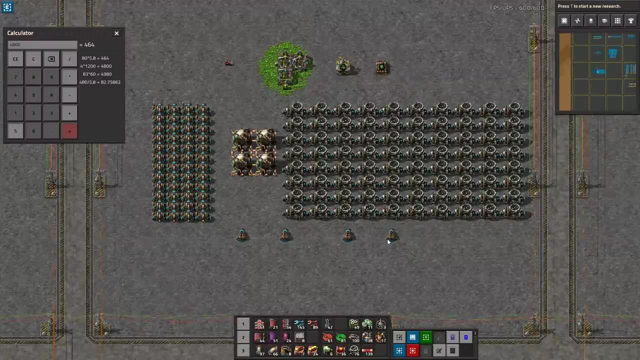 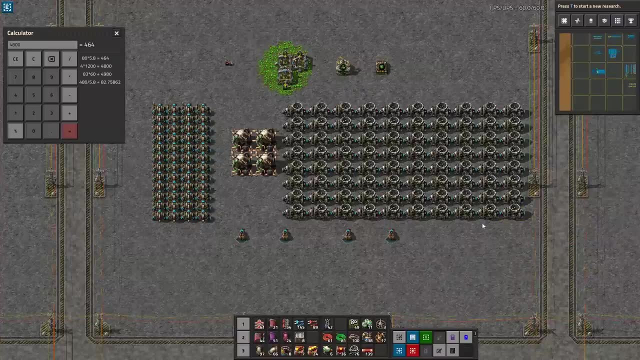 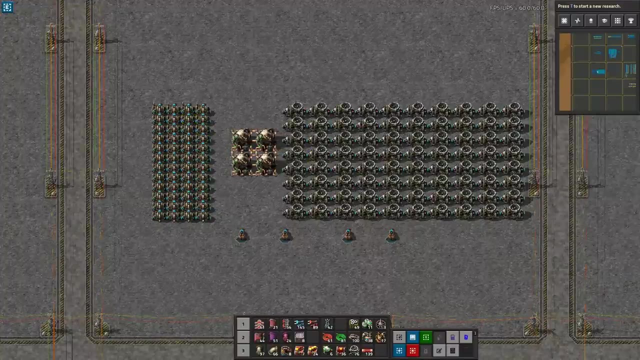 four nuclear reactors, four offshore pumps, 48 heat exchangers and 80 steam turbines. That's going to be the input for our project And that's going to be the object. So if we want to build design process, let's stop the design process, because what we can see here is that things 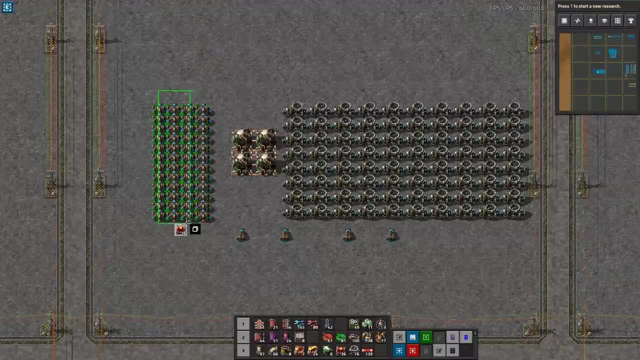 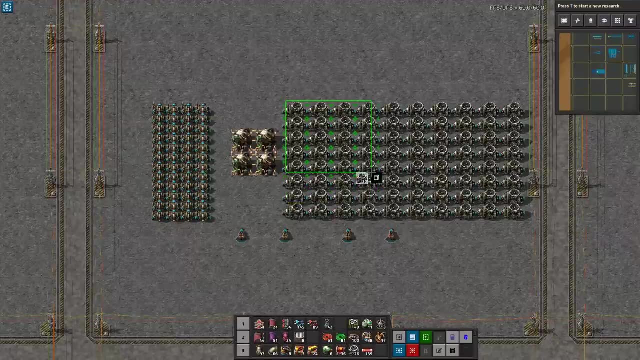 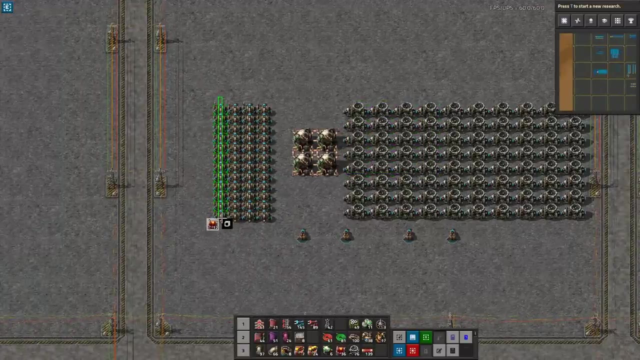 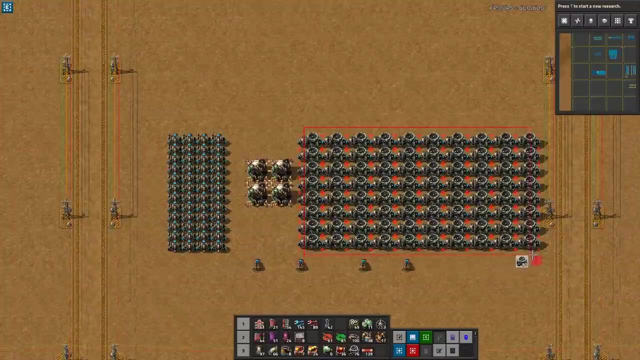 have a tendency here to be divisible by four. i have 48, so i have something with 12. i have 80, so i have something with 20.. so maybe i could build a design that takes 20 steam turbines and 12 heat exchangers, and that would be a good premise for our build. that's going to be our 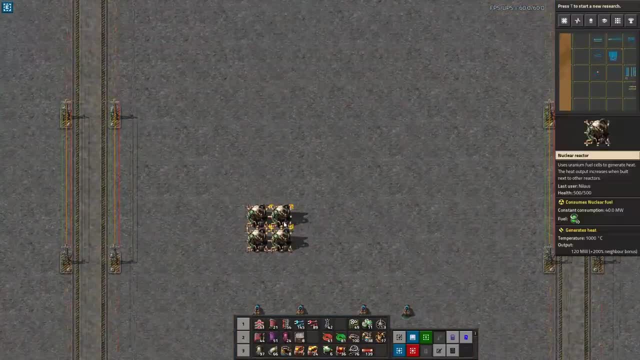 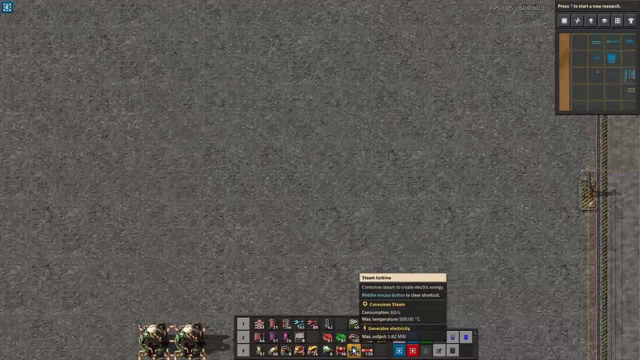 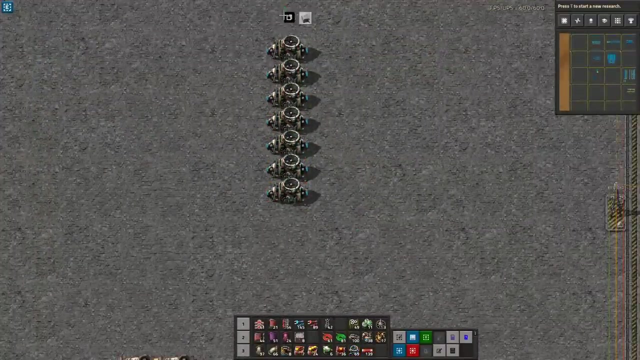 objective. what i also want to do is i want to make sure that i build something that is tileable, and by that i mean, if i bit stamp one down, one, i wanted to be able to feed into the other. we're gonna start by just making some random things here. this is seven, then. 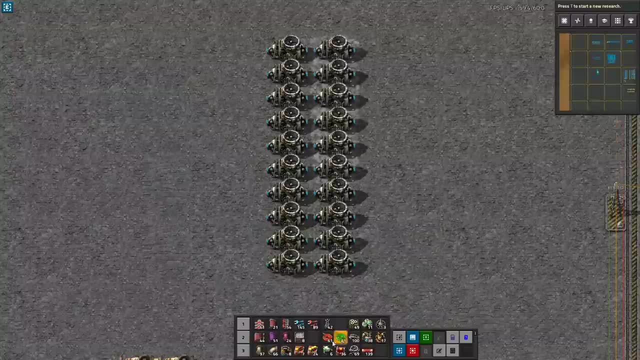 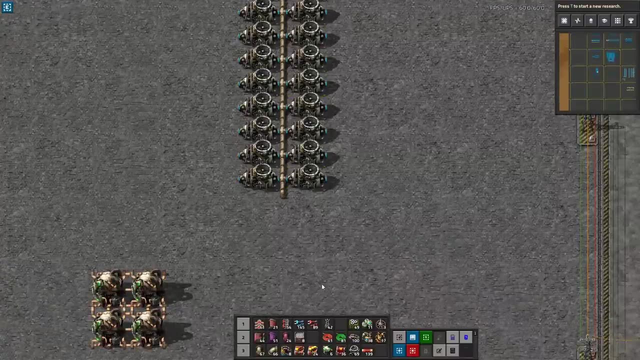 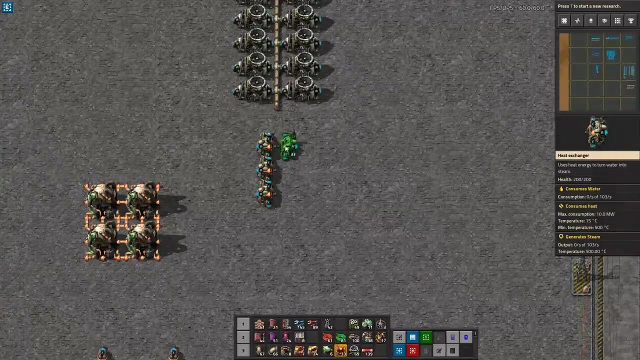 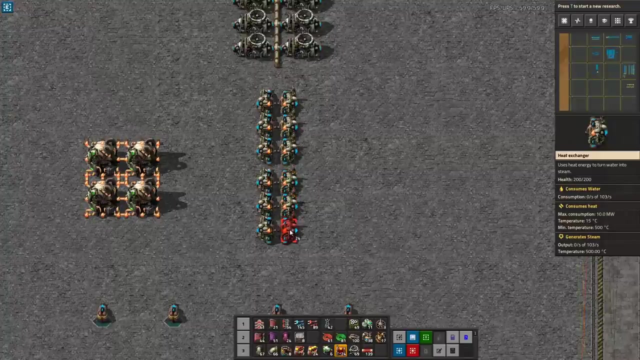 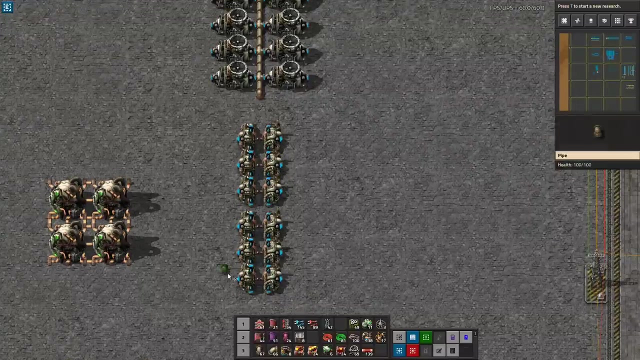 the. this seems good. it seems very reasonable to do something like this. we have 20 of these and in order to support it, i am going to have need one, two, three, four, five, six. here this is where things get tricky, because i'm gonna need to manage the inputs and outputs. 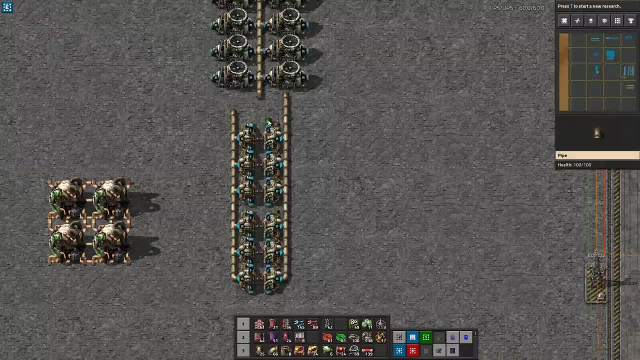 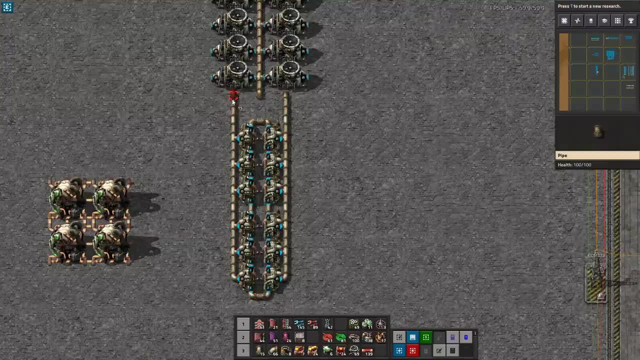 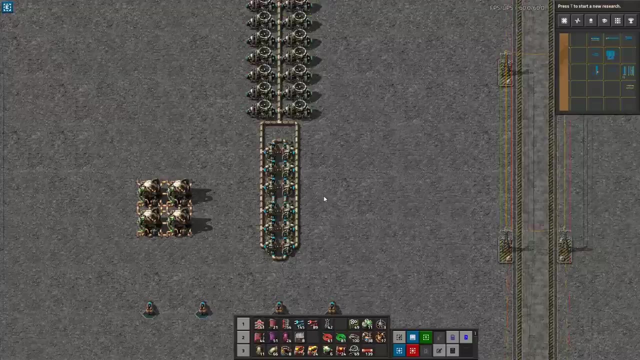 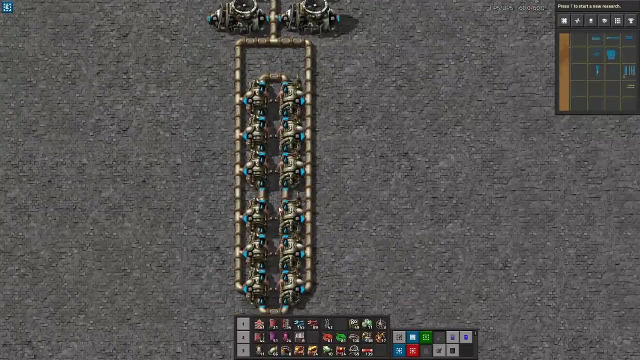 and i can do something like this, and if i do this one, that's pretty much. it's pretty okay, i would say. however, there are glaring issues here, the first one being how am i going to power this? because there's no underground, so let's punch a hole here. 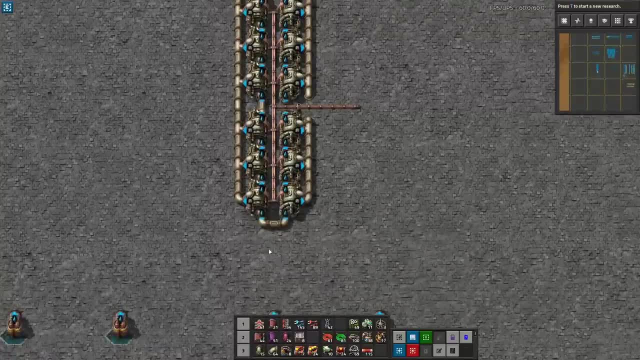 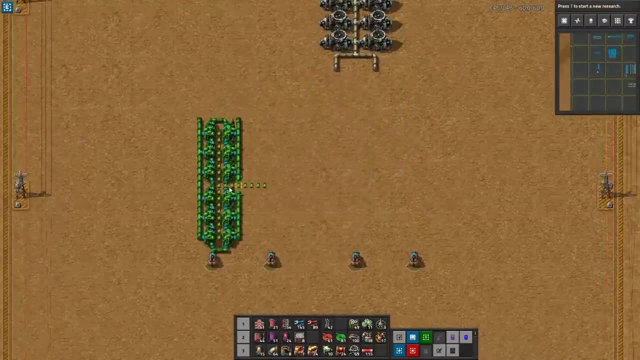 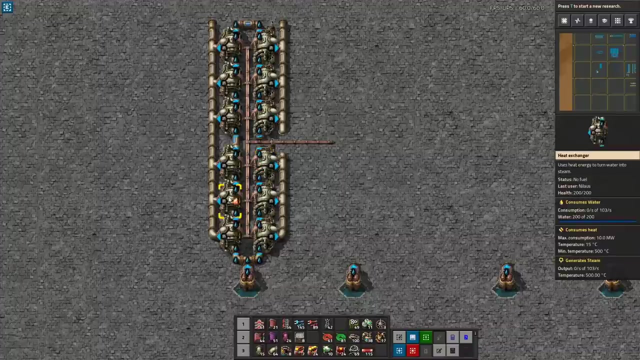 right. so what we have at this point is water is coming in here. we can take this out and move it towards the water, just to make it simpler there. so water comes in here, it comes in here, it goes up to these, it goes over here and then over there, and then over there. 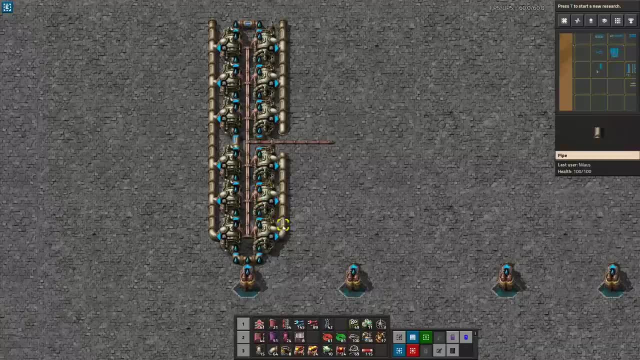 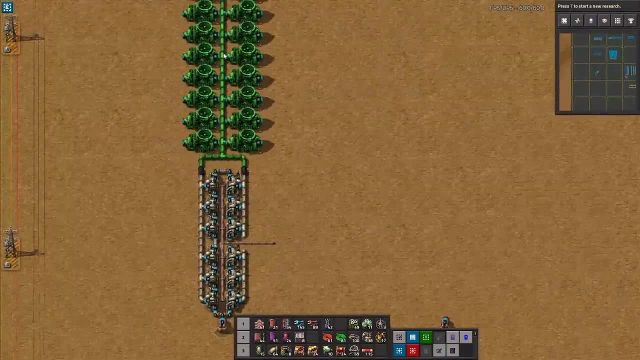 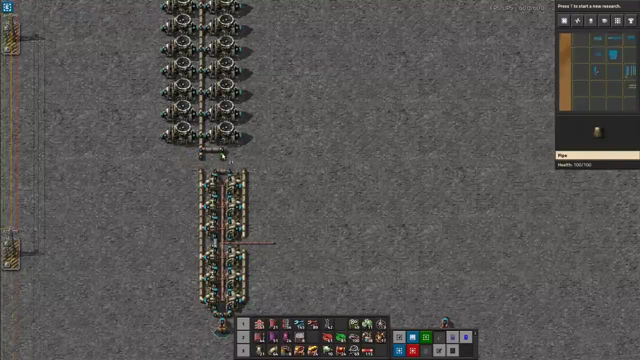 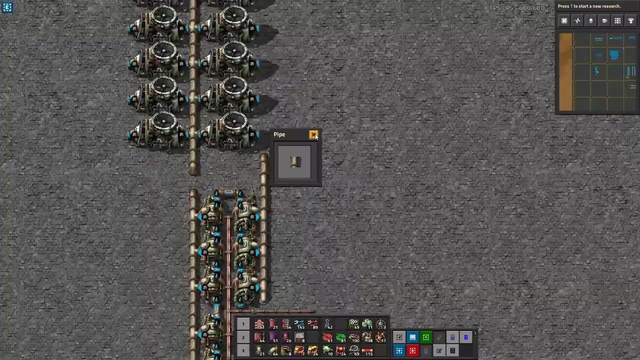 around and down looking good, the steam goes this way, this way, and i'm gonna have to find a way to get it up here. i'm just gonna build it like this, just for no apparent reason, and what i just did was actually i messed up. now we use the new function here in point 18, 35, i guess, with the 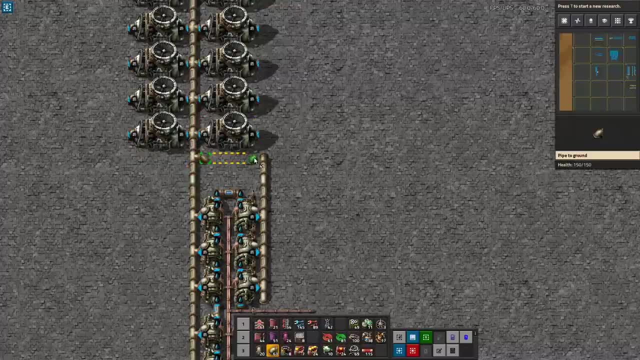 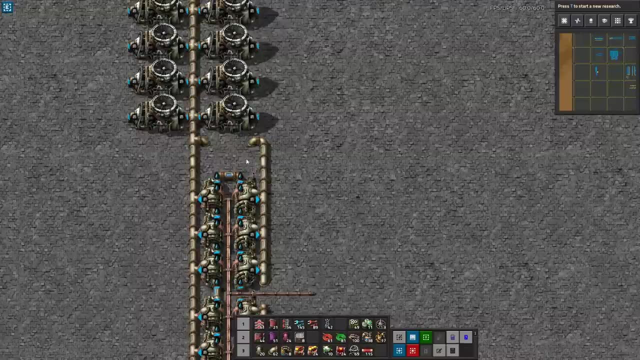 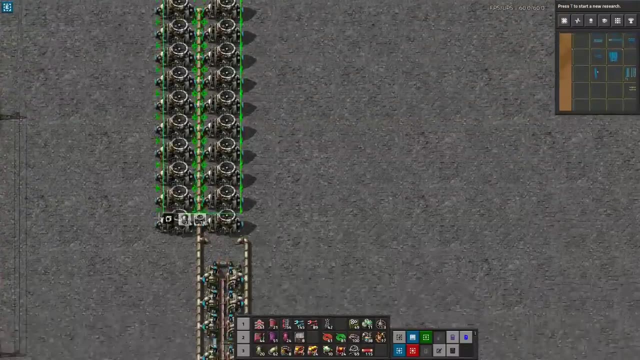 cleaning out of the pipes. i've honestly, perfectly, i've actually preferred being it blocking me from doing it because it's the wrong inputs, rather than having to clean out the pumps, the pipes. so we've built one and we need to build four of these. so what i'm gonna do is 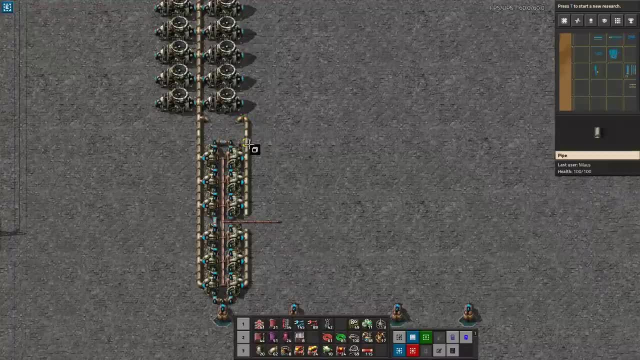 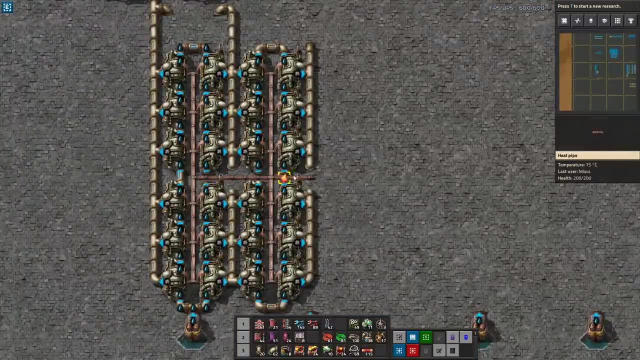 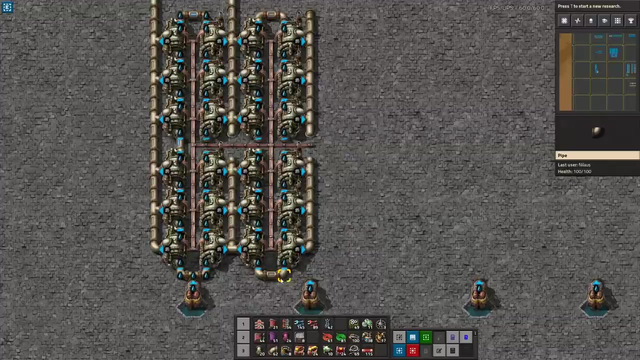 i'm going to say, yeah, can i just get this one built next to it, like, like that, maybe this one goes through looking good. but we do have an issue that this part up here is not getting the water, and i want to make be very strict about this. water goes only into these, these 12. 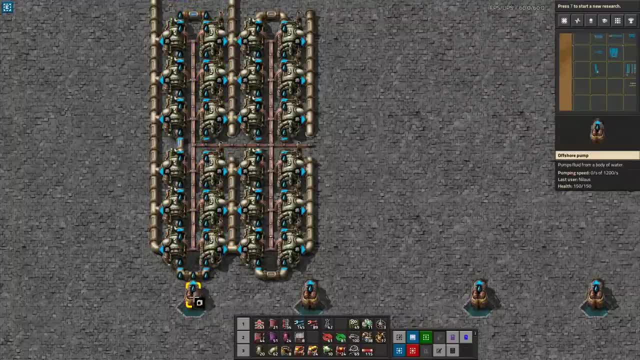 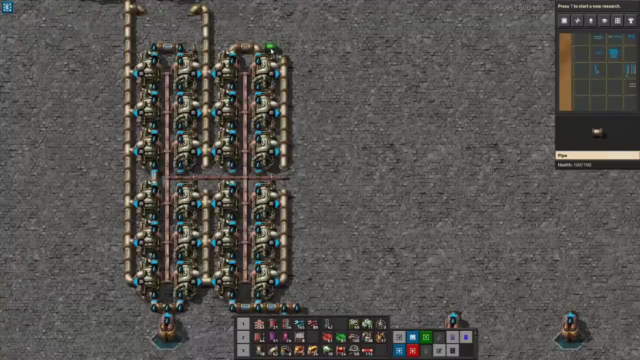 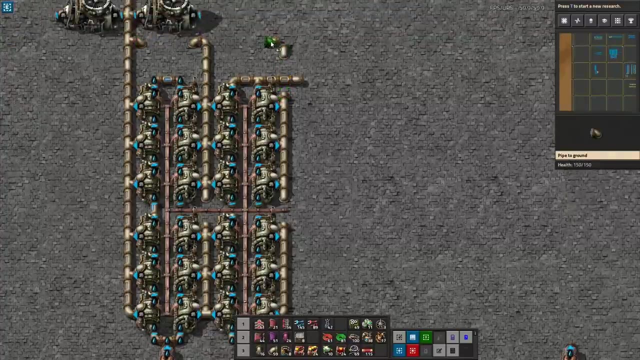 are consuming exactly, oh well, not exactly. they're slightly over consuming what this one can provide, so i don't want to start mixing it. there's no point in mixing it, so let's actually go this way. the steam, though i want to mix, the steam will be out here, and 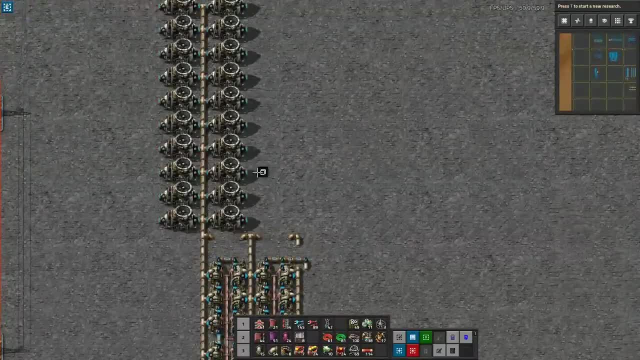 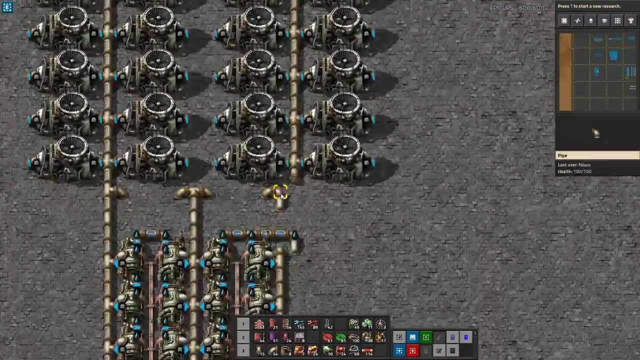 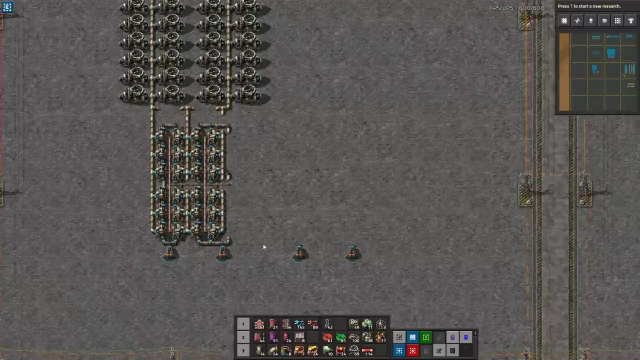 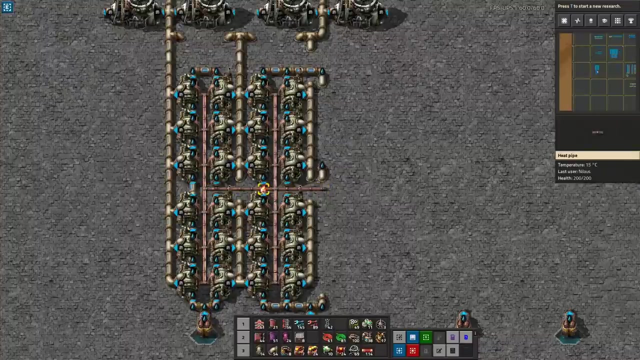 here. so now we build something. i am going to take this part here and right. so what we've done now is take half of it and i'm actually just gonna mirror it, because we now have an ability here for the heat pipes to go in to all of these and the distance is pretty much as short as possible. 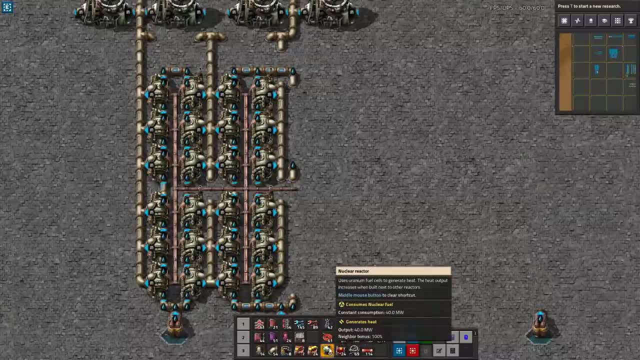 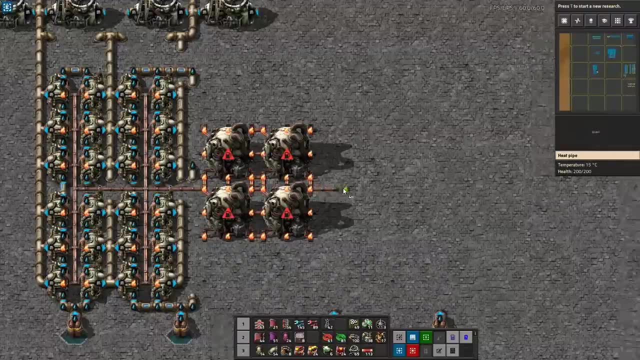 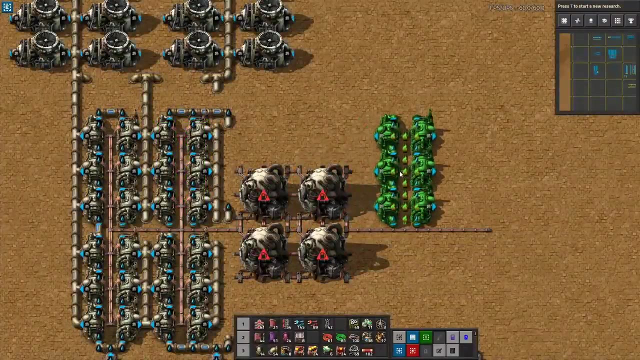 i think that's an important aspect, that it is as short as possible. let's put our nuclear reactors in. we need the four nuclear reactors and then you start seeing that there is a repeatable pattern, which is good. we like repeatable patterns. two there, if i can rebuild it correctly. 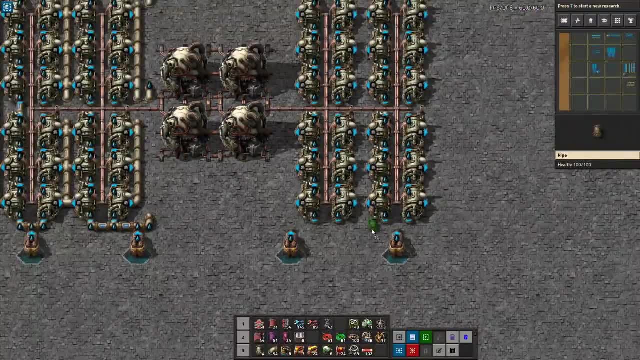 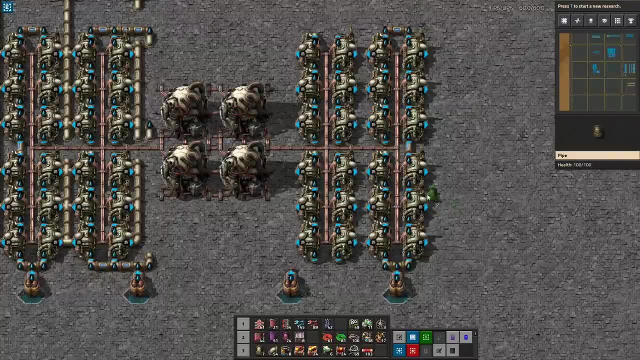 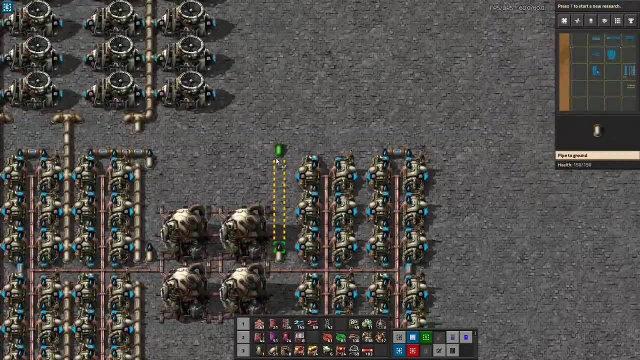 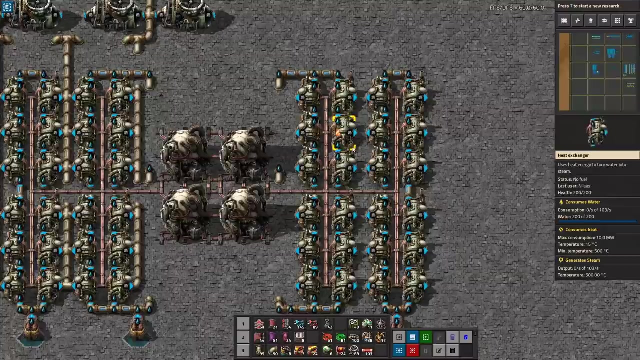 without too many issues. that one and that one are idle, this one here going up around, so this is now fully watered. i'm going to fully water the other one. yeah, and now all of this is fully watered. now we're going to deal with this. theme goes up here. 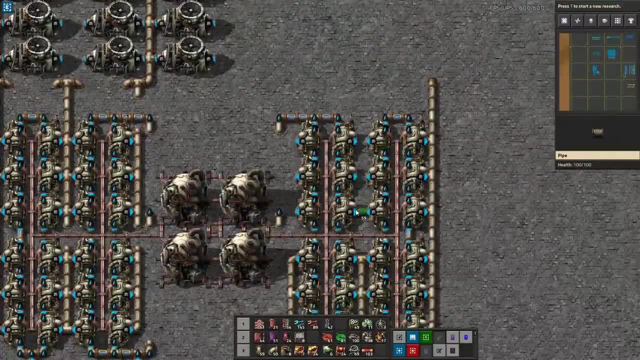 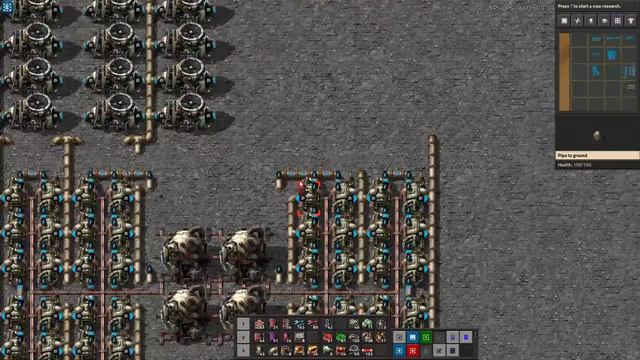 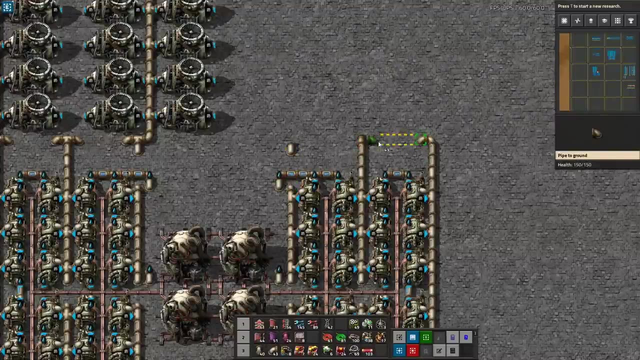 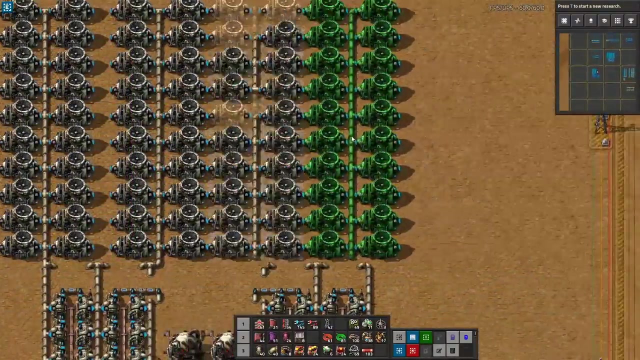 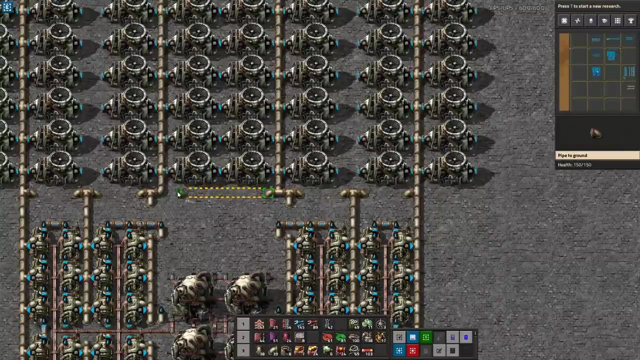 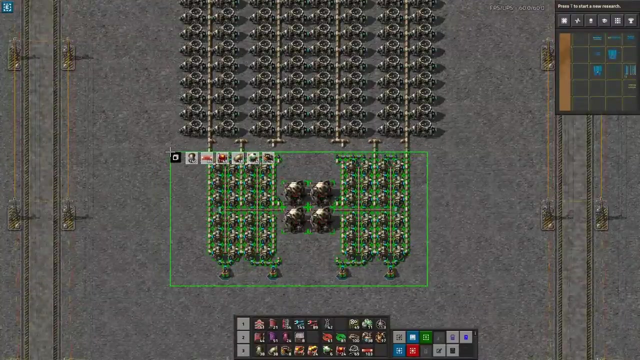 here. this one goes straight up, jumping over this one, technically jumping under who's counting, and again doing this, and i want to now do this as well. this is going to mirror here and here, here and these. so what we've now built is four reactors, four reactors, 48 heat exchangers. 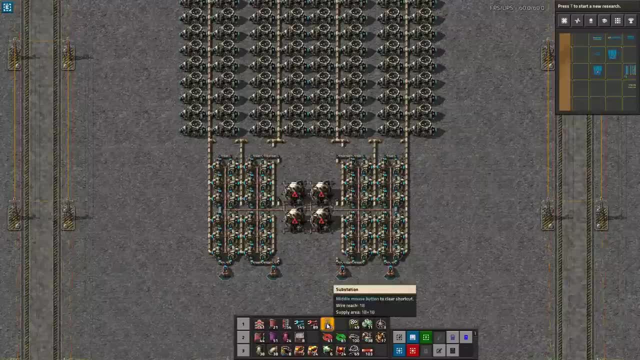 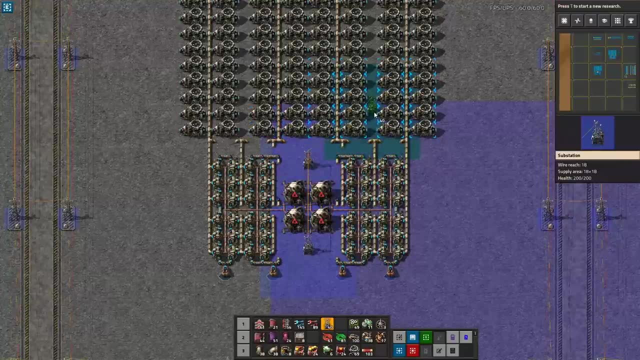 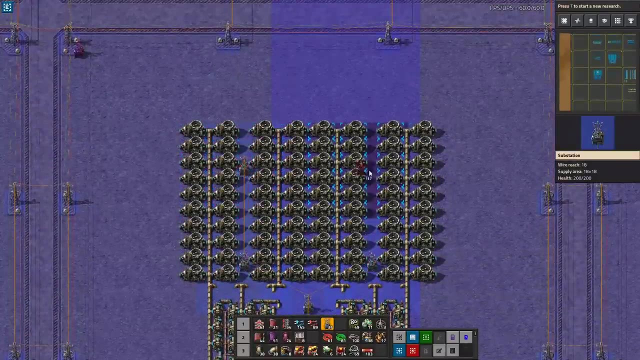 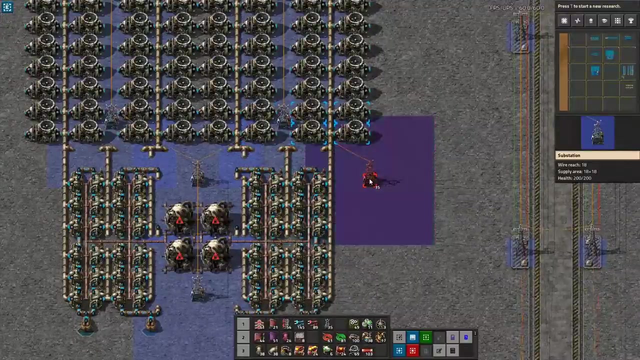 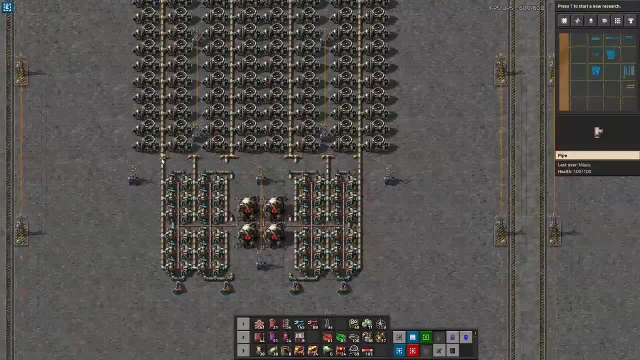 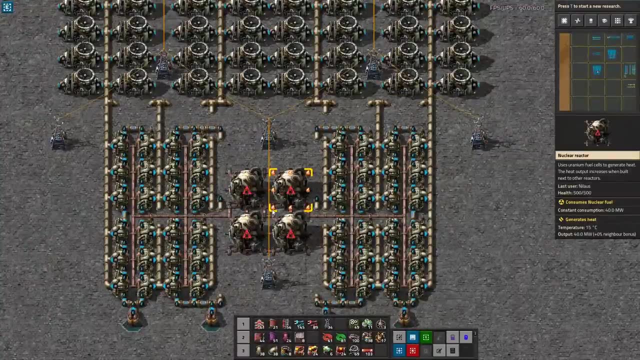 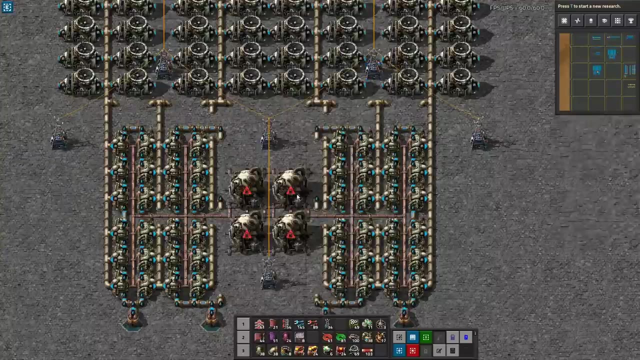 because i'm testing but we need to make the power, so we still have some things to sort. for example, these are blinking because we don't have any any nuclear fuel coming in and also- i forgot to mention this- nuclear fuel is actually outputting some waste nuclear fuel when it's done. 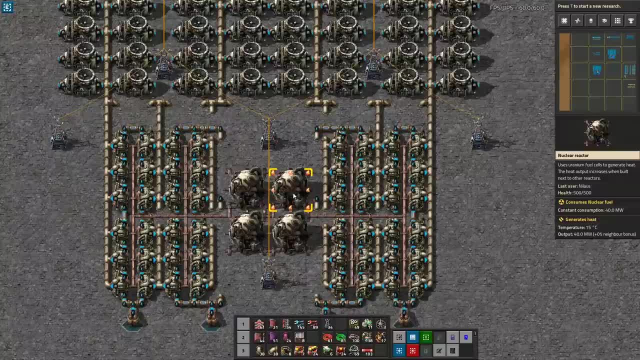 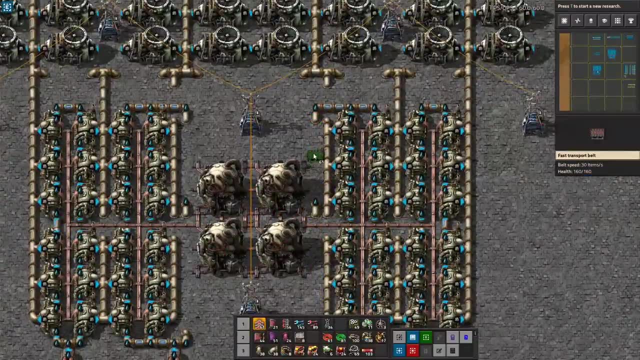 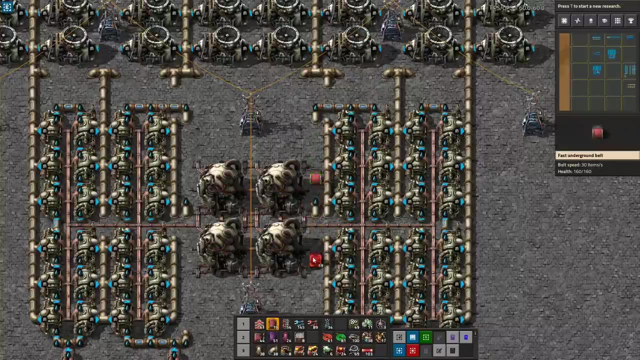 and that one that waste nuclear fuel can be reprocessed. it's not a big deal, but it it's, it's kind of important to collect. so what i want to do is i want to make- and this is some people find this strange, but i really like this, i really like this, uh, this design concept. what? 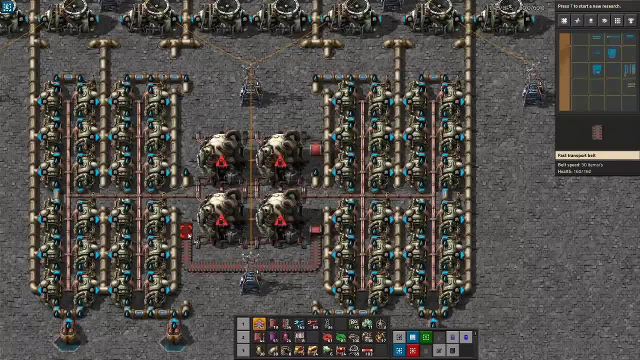 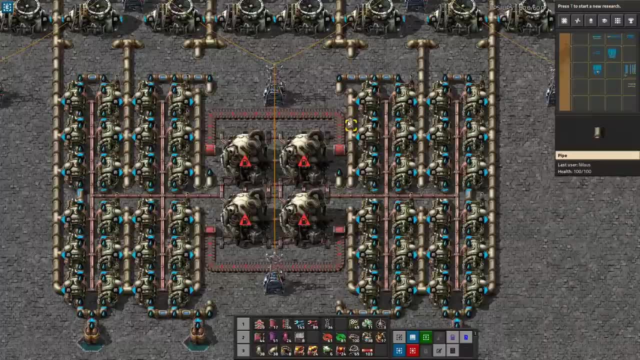 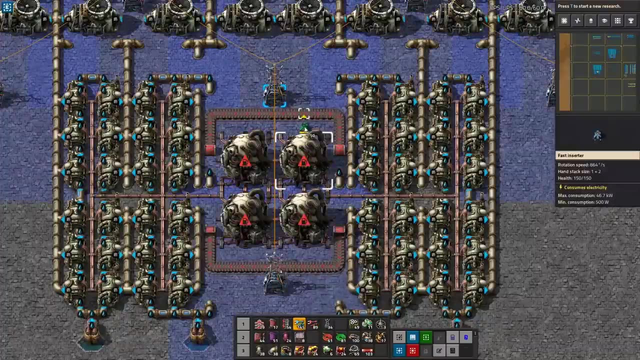 i'm gonna do is i'm gonna make a little roundabout around this one here, so i will have both here. so i will have both the uranium fuel and the uranium waste fuel on this belt. the way i'm going to do it is: i am going. 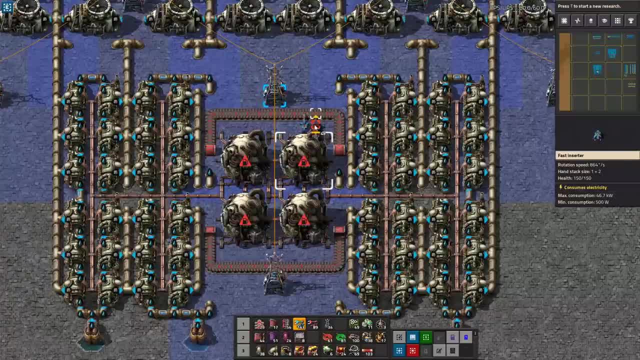 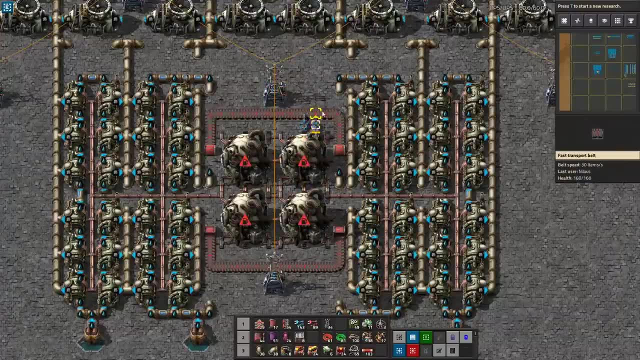 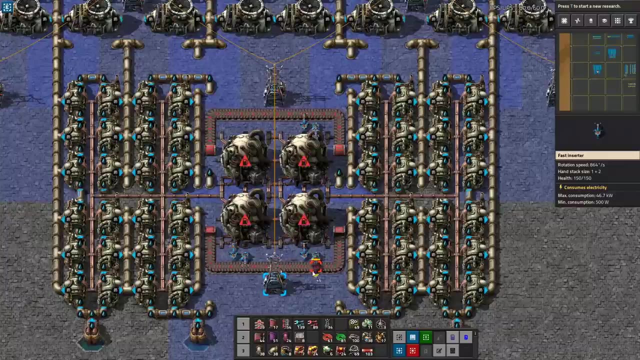 to say this: one goes in and then it takes whatever inputs out. this will only take the valid fuel in and it'll only take the used fuel out and, more than that, it'll guarantee that, if i put it on the inside belt, the fuel, the used fuel, 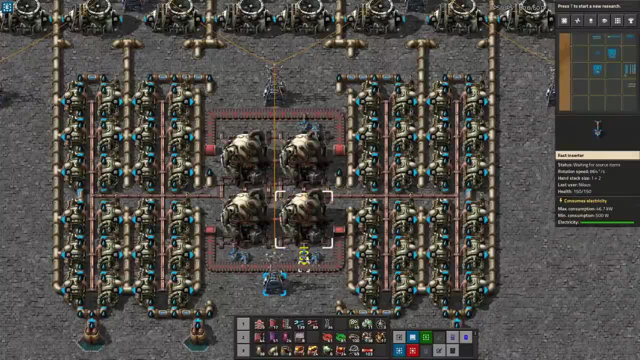 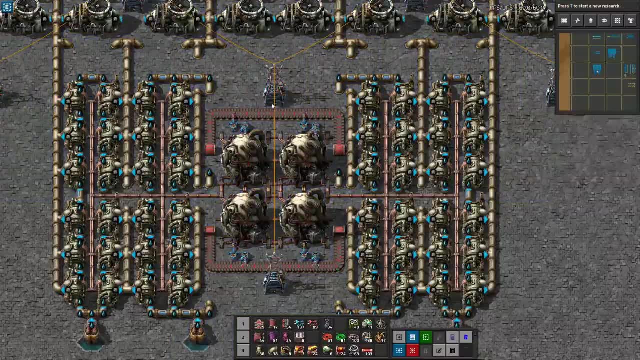 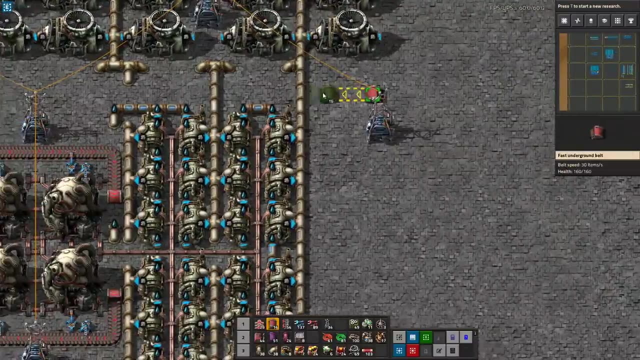 the used fuel, no, the useful fuel, and then this inserter will output on the outside, which will always be room here, and what i then do is i will make sure that i can, from this side, bring in and, lo and behold, someone actually made room for this. 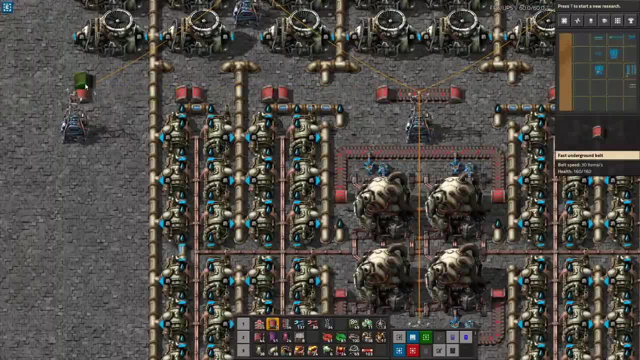 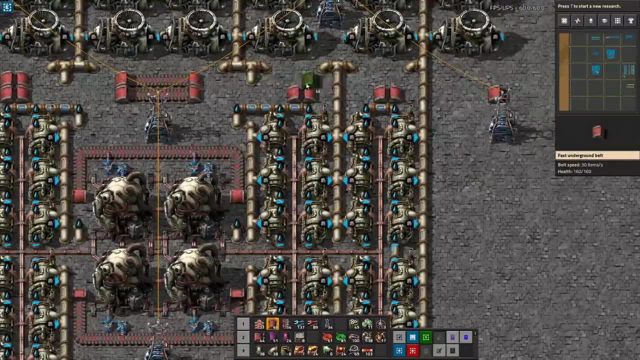 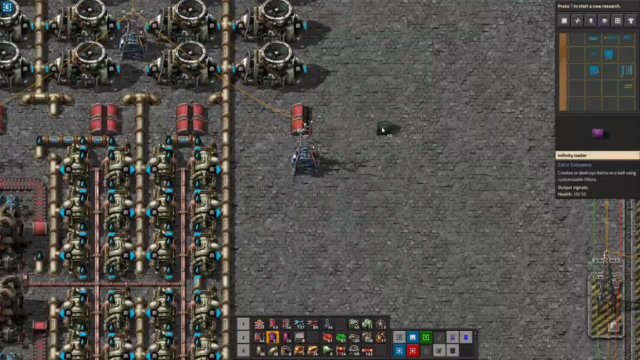 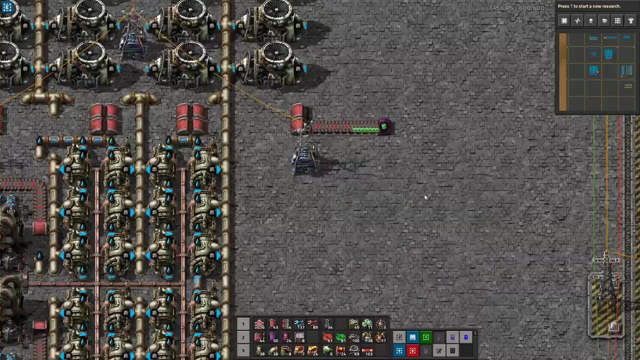 and all the way over and so on this belt. i will simulate that we have inbound some fuel and it comes there. the other one will be a waste one and i will simply put one of these in here, and then i will simulate that we have inbound some fuel. 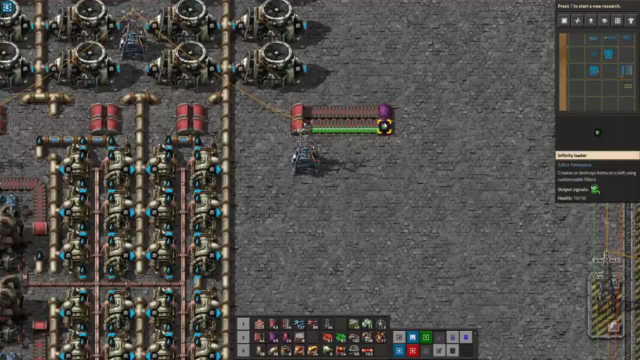 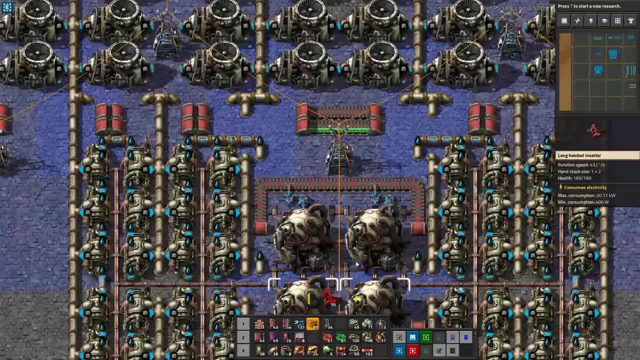 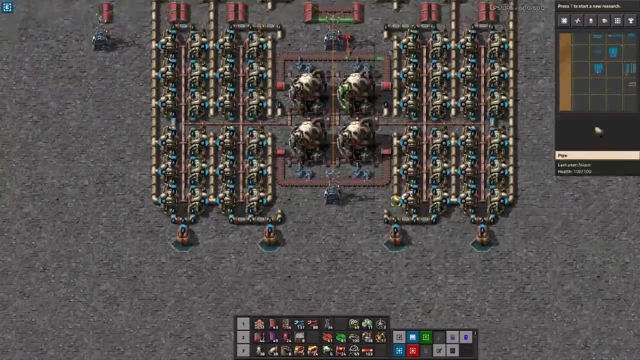 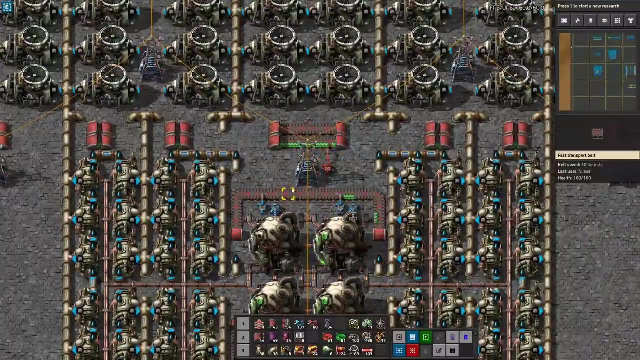 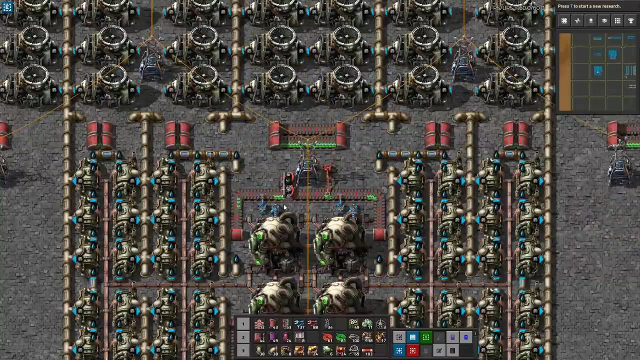 and it comes there automatically. we can see the fuel is filled now. so let me c turn it on. i can see if it does, for example, a very power up this, then this. so this is a boiler out, which is what we do here. you can see, when it passes through, nothing goes out on the top side. 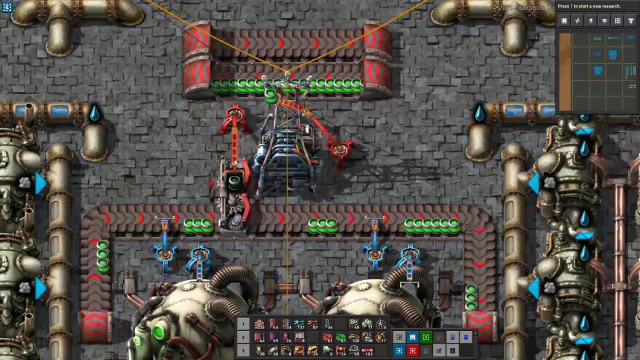 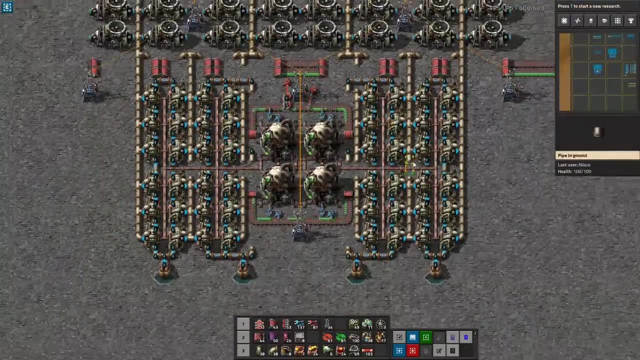 but if something goes on the top side, a long-handled inserter can actually pick it up, and i'll put it here. i'm actually not going to take this one, but because i want to see something i like. so let's have a look at what happens during this process. as it fires up, you can see. 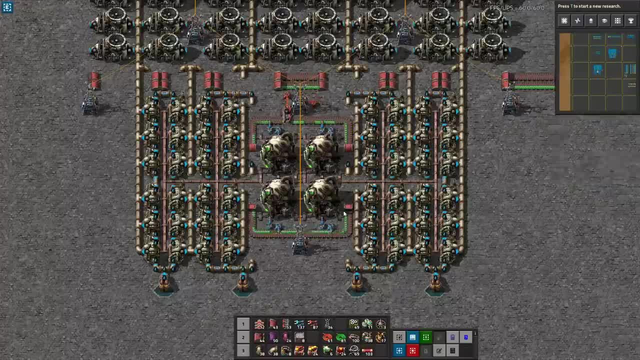 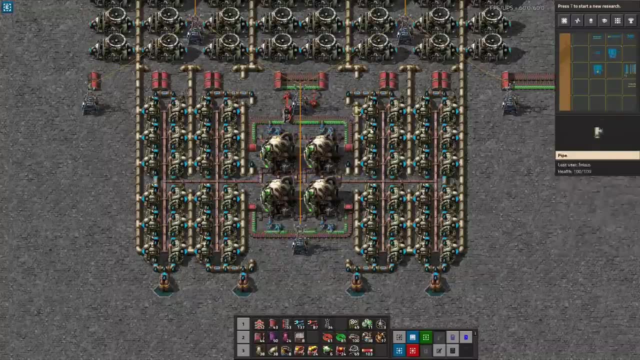 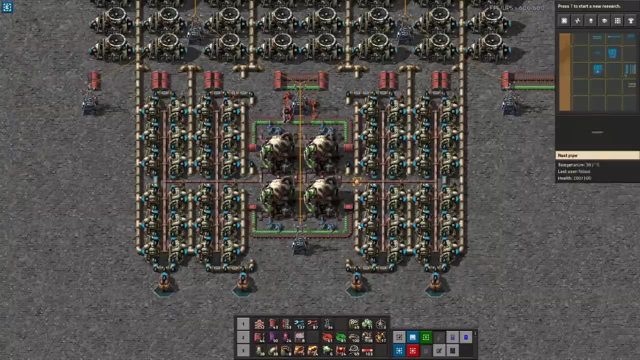 and some people might not like this because it actually wastes a lot of materials going around. i don't really mind that so much. if it's not saturated, it'll just be the same few things running around. when it is saturated, it's okay. it's not going to consume more, it's simply going. 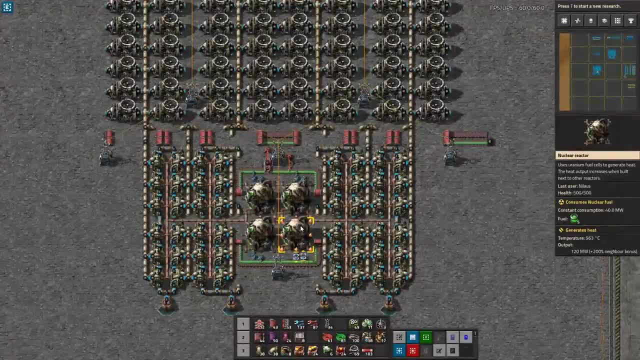 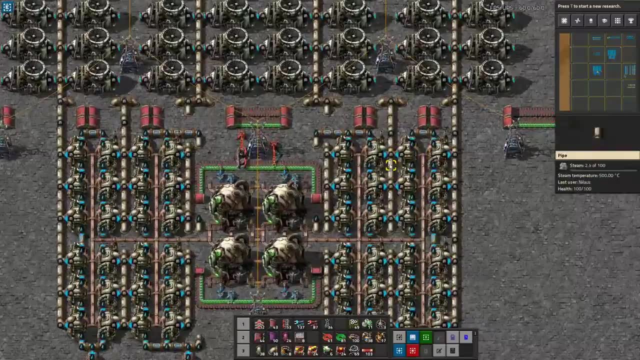 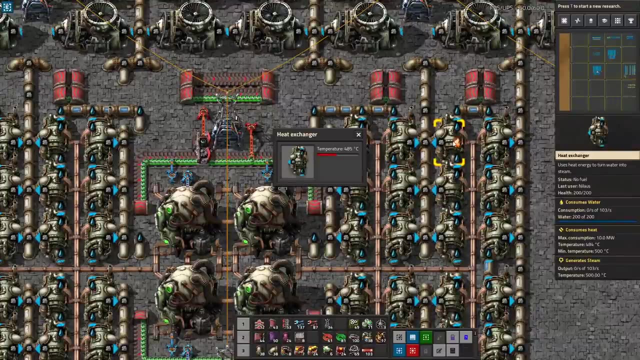 to set this up. let's have a look. we can see stuff is going on. you can see stuff is flowing. eating is going in. eating is not all the way up here, so this one isn't working yet. only when this one hits hits 500 degrees will it start producing steam. you can see no outputs on the left hand side generate steam. 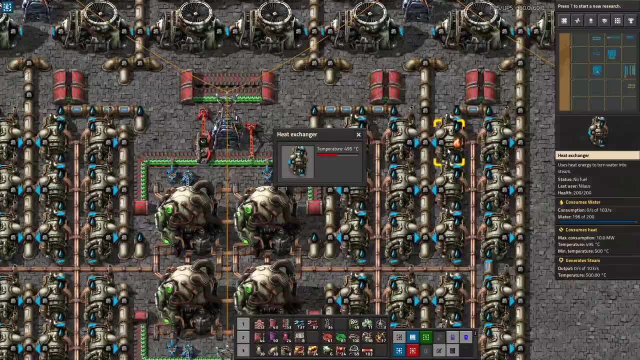 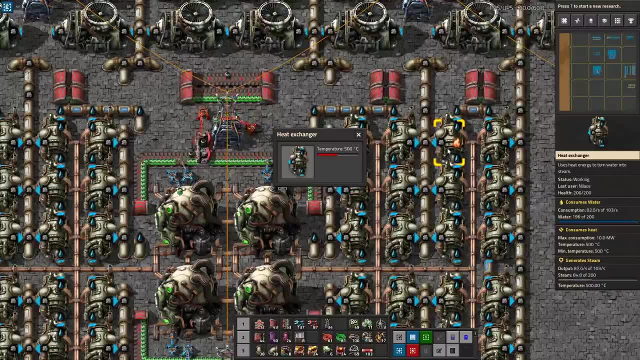 zero. we're just going to look at this one while waiting. also, we can see some fuel coming out, waste fuel coming out. there's some waste fuel being picked up and they are, and they are working perfectly fine. and now it's generating and the steam output is now full. the steam buffer is full. 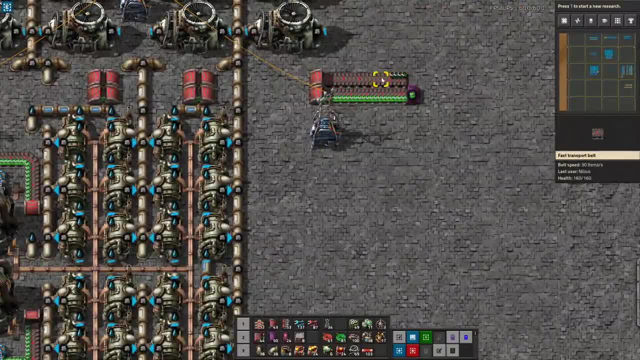 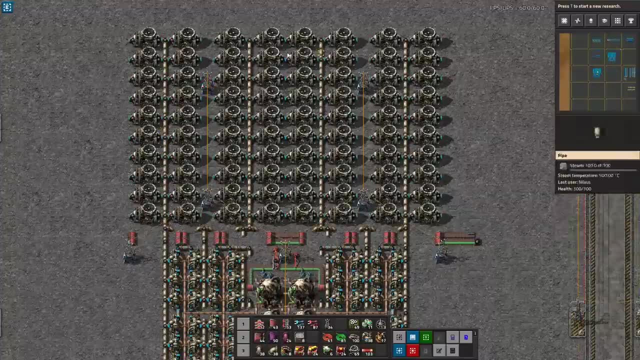 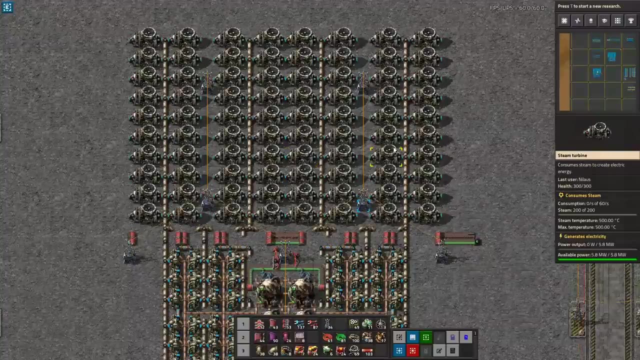 and we have the first four fuel being consumed and it just keeps working on the next one, next fuel. this is now in a steady state. all of this is working if there, at this point, was anything drawing power from it, but i don't have anything that's drawing power suits at zero right now. 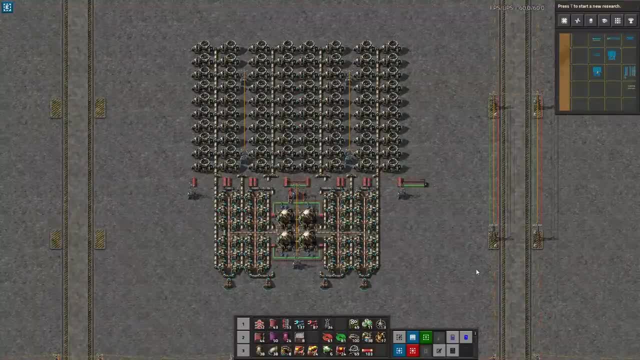 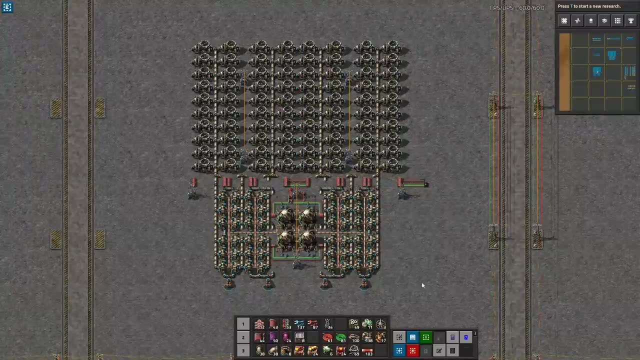 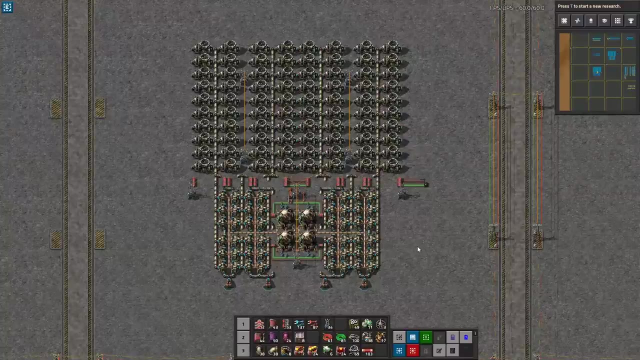 so there you have it. this is a very simple, very robust, modular, tileable design of a nuclear power plant with four reactors generating a max production of 464 megawatts of power and using four uranium fuel- nuclear fuel per 200 seconds. now, that covers the design process. 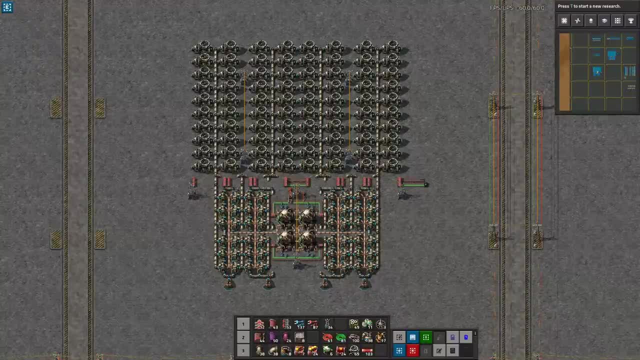 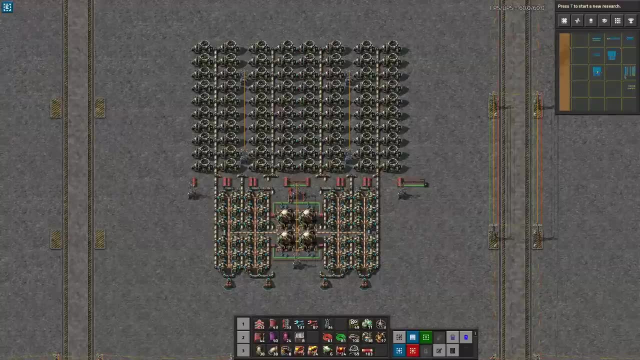 of the uranium fuel or the nuclear fuel plant. however, there are a number of things that i want to draw attention to. these are more advanced topics that we'll just dive into in a second, but i wanted to make this incremental. first, explain the mechanics, explain the ratios, build. 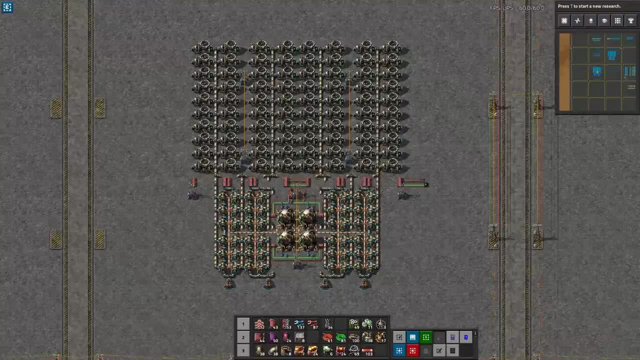 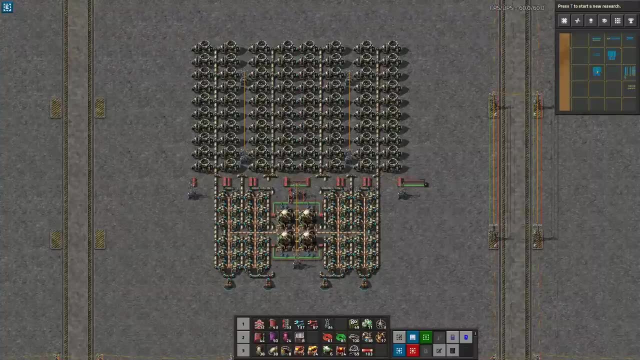 a robust design and then from here on, we can go in and discuss some of the more advanced features and- and i will show you what i think most people are not realizing when it comes to euringian power. but before we do that, i'd like to take a second just to thank all the patreon supporters who are 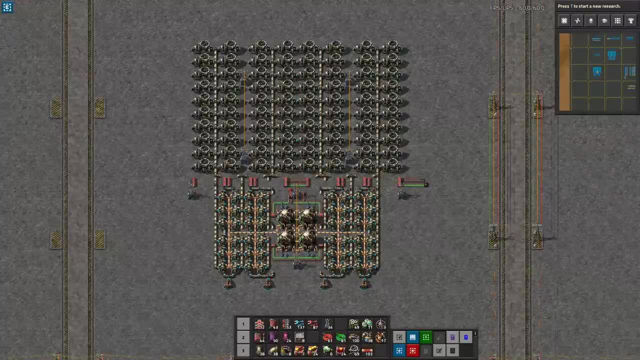 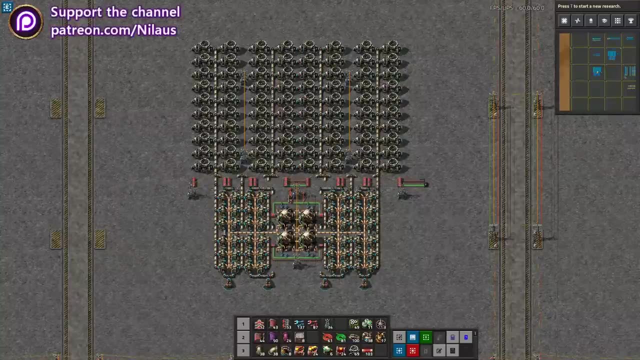 supporting and helping me make videos like this every day. if you like what's going on here and you want to support the channel and the work i do, then pledging on patreon is the best way to do that. there should be a link on the screen and in the description below. thank you very much for. 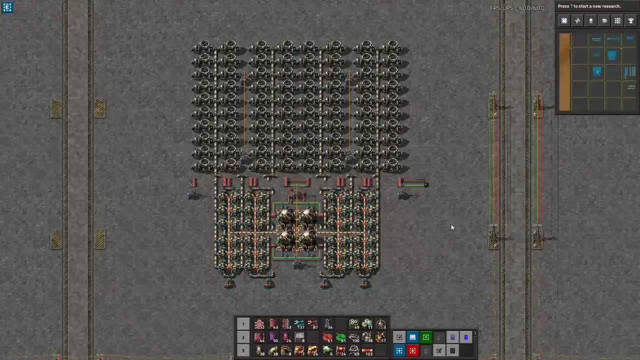 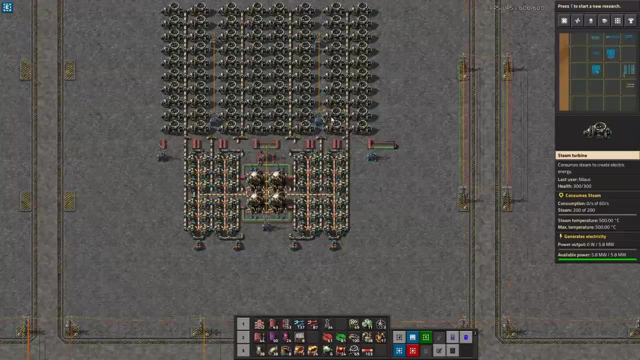 all the patrons supporting the channel. if you enjoyed this video, please leave a like and subscribe to my channel for future videos. Thanks a lot. Now there are two important topics that I want to discuss. One is steam storage. You can store the steam being produced so that it is available when needed. 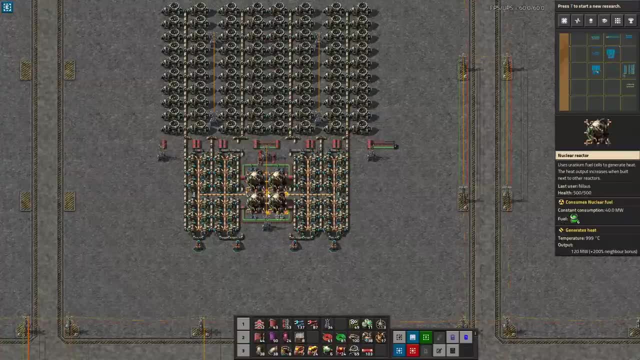 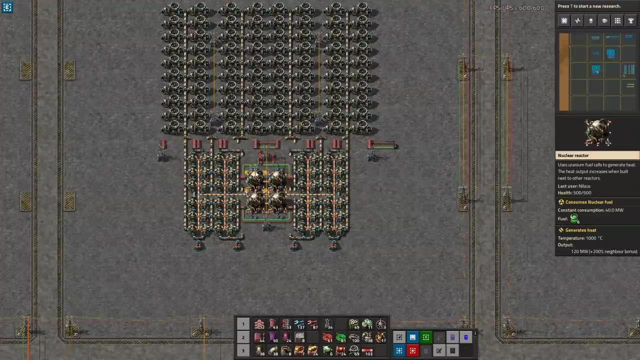 and therefore stop actually feeding the uranium power some uranium fuel and thereby save uranium fuel. That is one topic I want to talk about, And the other topic is scalability beyond a 2x2 reactor into a 2x3 reactor, 2x4, 2x5. 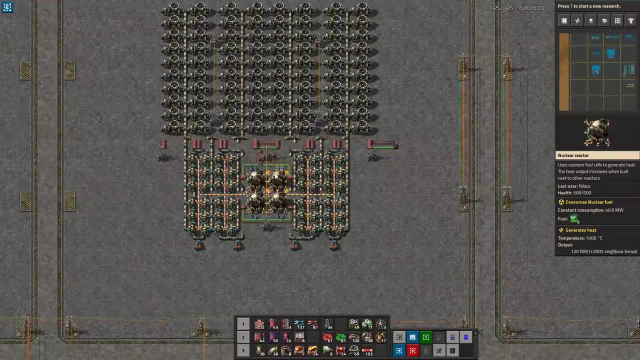 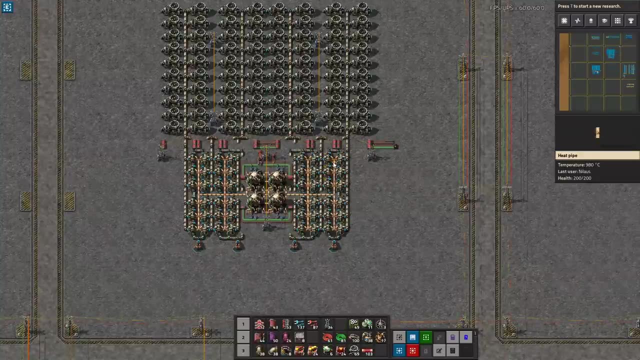 I see a lot of designs with multiple larger reactors, as if that was better, And that's what we're going to dive into. But before we do that, or as input for that, I think it's actually time for us to do some math. 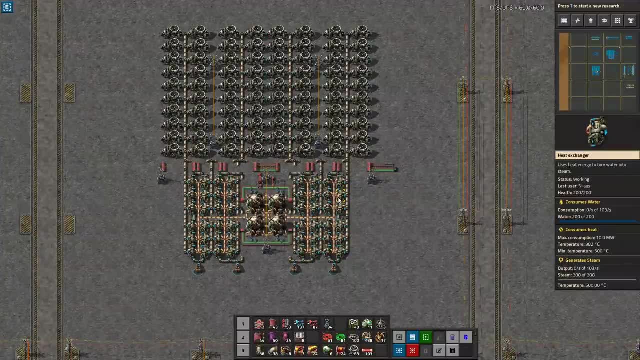 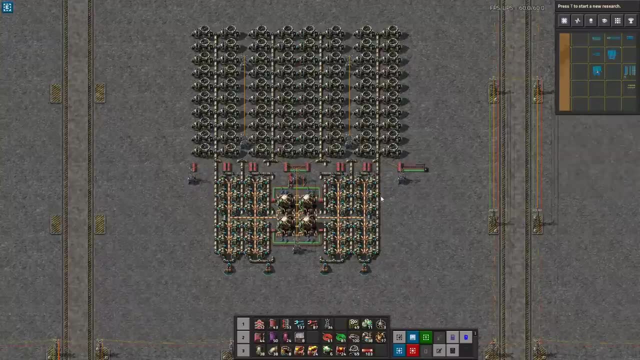 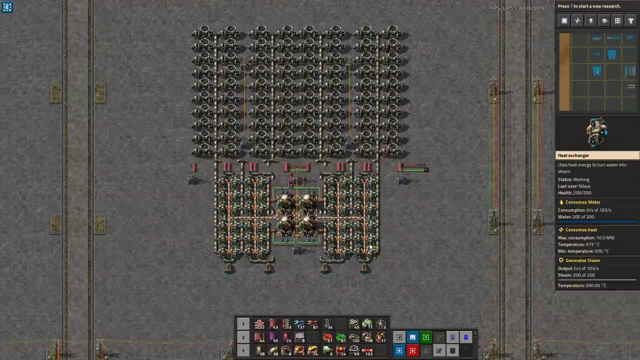 And right at this moment, everyone disappeared from the channel. The reason I believe that we need to stop doing some math is because it will reveal something that I don't think you are aware of, And that is basically how extremely above abundant uranium is, even under very conservative considerations. 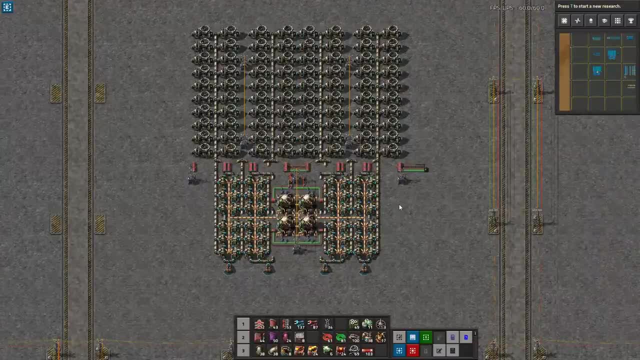 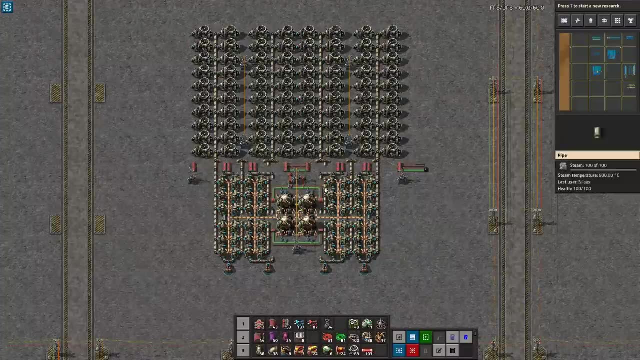 And because of that it will completely invalidate any need for steam storage. It will completely invalidate any point of building it larger than this. Let's take a look at the math. I have prepared things here We're going to do. I'm going to walk you through the process. 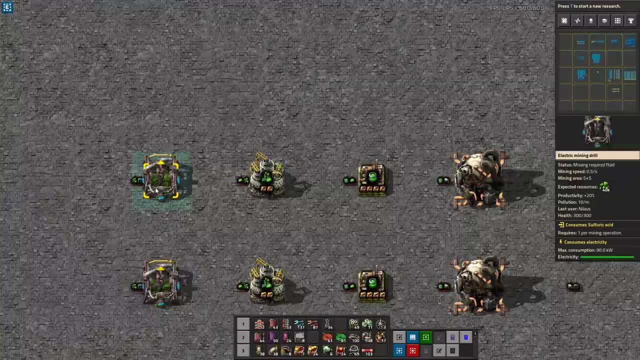 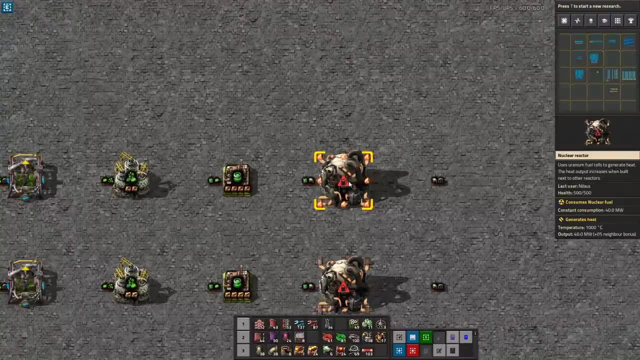 We're not going to do very extensive math, but my objective is: I want to know how many electric drills I need to have in order to support One uranium nuclear reactor. That's the calculation. I could give you the calculation, but then you wouldn't believe me. 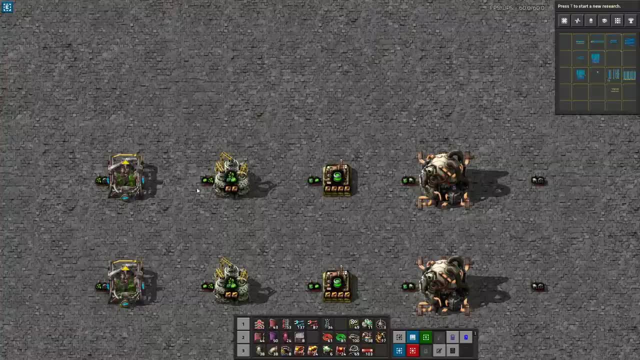 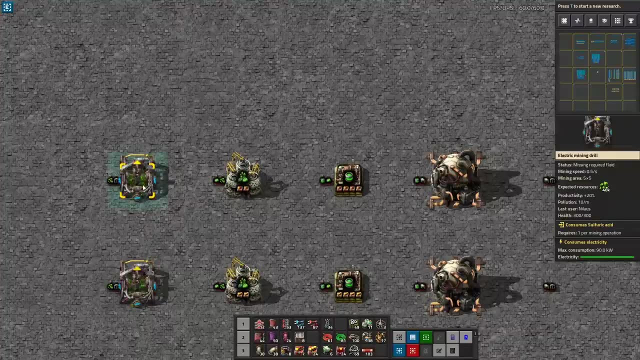 So we're just going to walk through it slowly here. I'm going to do this, this calculation at the onset. This is when you've just unlocked uranium. That means you can see here, the productivity over on the right-hand side is 20% productivity. 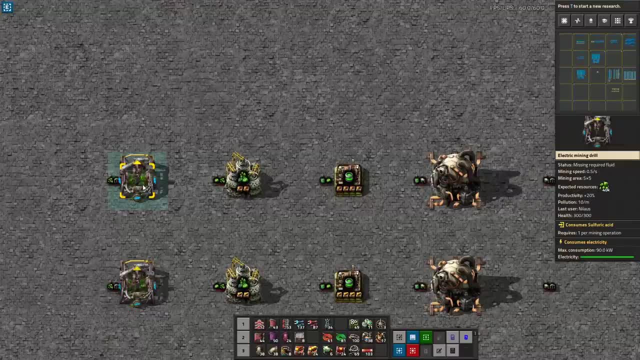 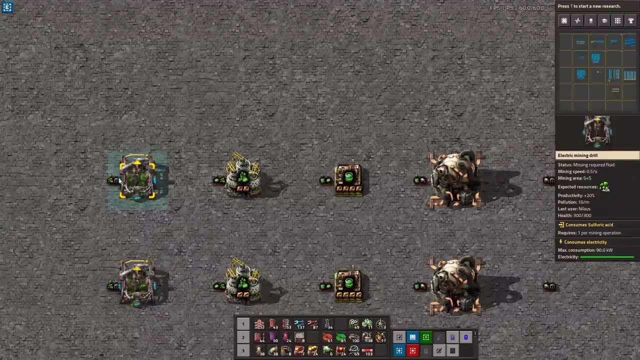 This comes from two researchers of mining productivity. I'm not assuming any end game mining productivity here, just 20%, which is what you can do at BlueStacks. We'll talk about that when we're done here, But I just wanted to show you two signs. 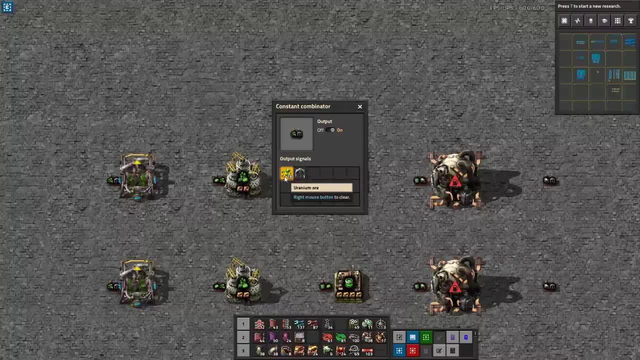 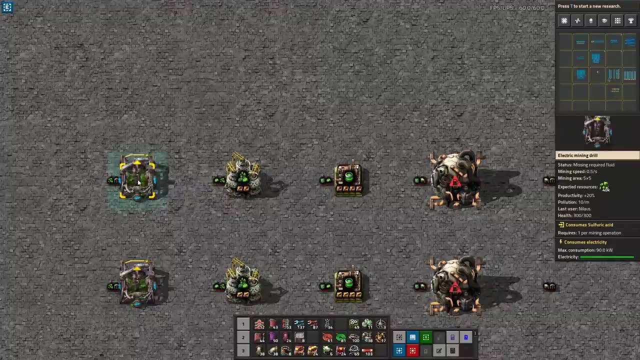 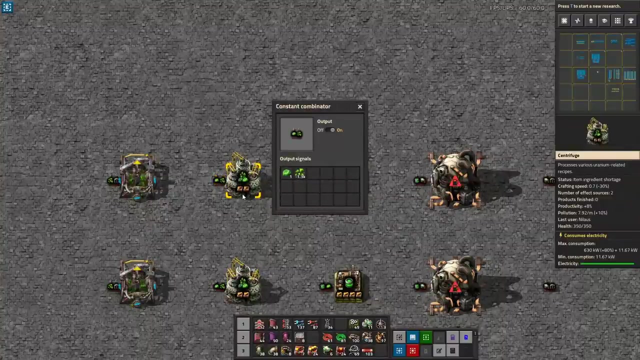 The thing is here. I have set that one miner is generating 18 fuel or NT uranium every minute. You can check each of these considerations and that is with the 20% productivity. Now we take this as I described in the beginning. 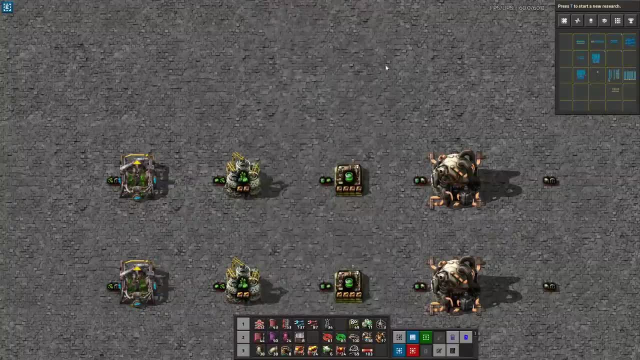 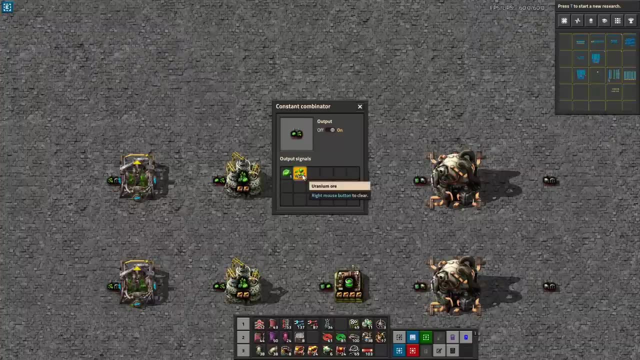 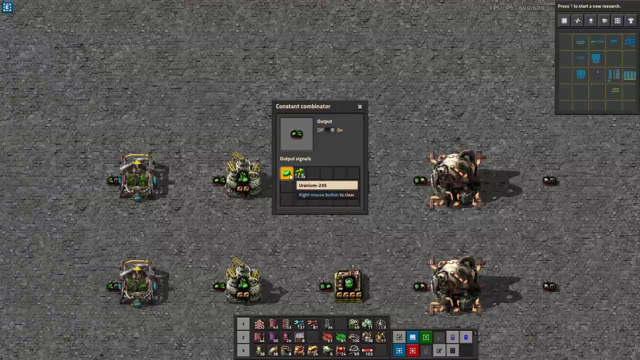 I'm basically saying if this process, this process, has uranium, if that's the case, then i need 1323 raw uranium to, on average, produce one uranium 235. of course, this is on average and since it has a yield of 0.7, it's not going to be exact, but 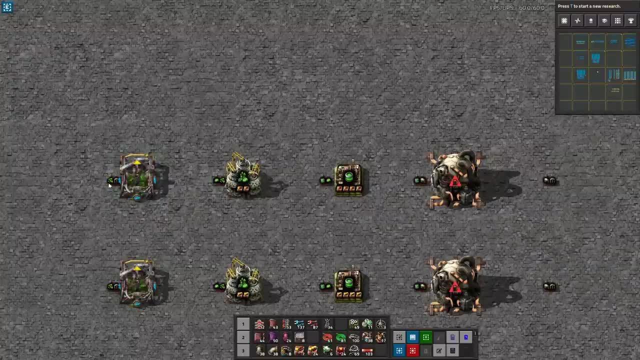 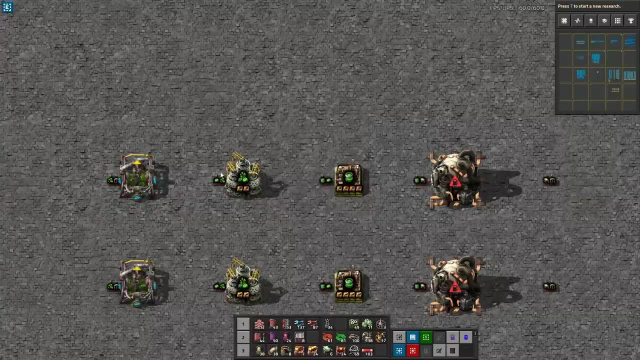 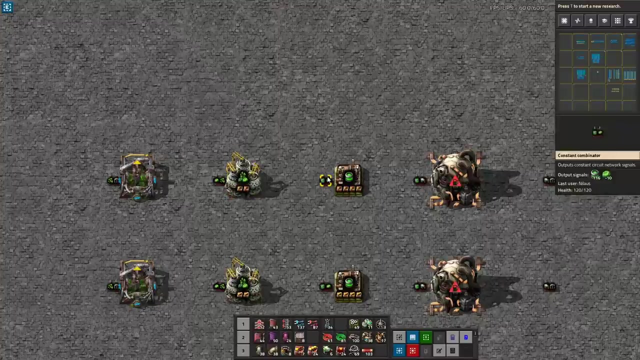 it just gives us an idea that the relationship between that. this is a very large number and this is only producing 18 per second, so that doesn't look good. that's starting to go like: oh, i need a lot of miners in order to feed this. however, the thing is this: one has now 16 productivity. 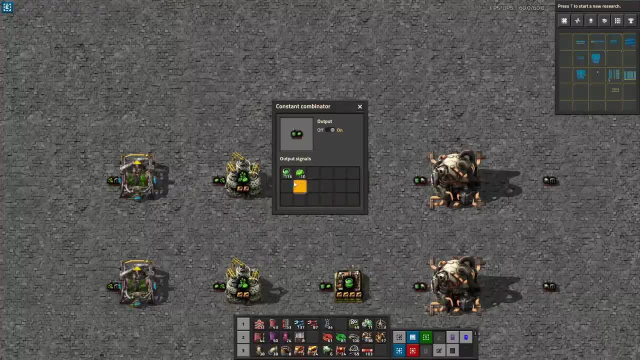 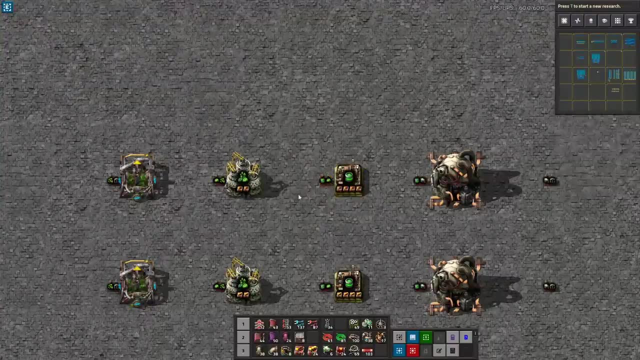 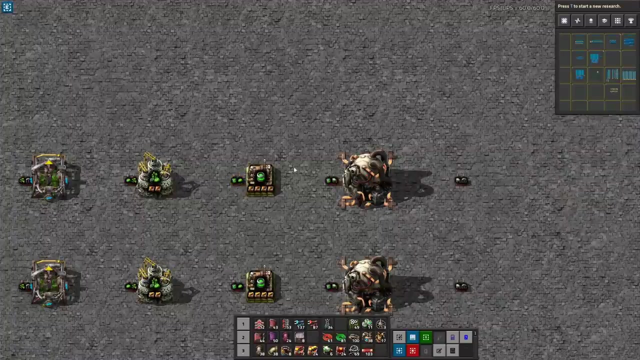 that means for every 10 we put in, we get 116. it's more than a factor 10 output. it's a factor 10 plus productivity output. so even though we only get one from every 1300, then you're actually getting a more. and this is the kicker if you look at it from a per second perspective. 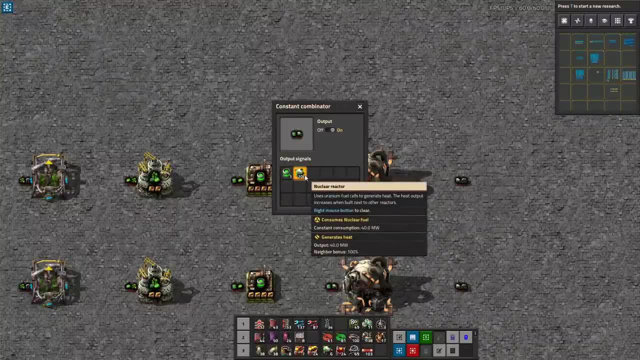 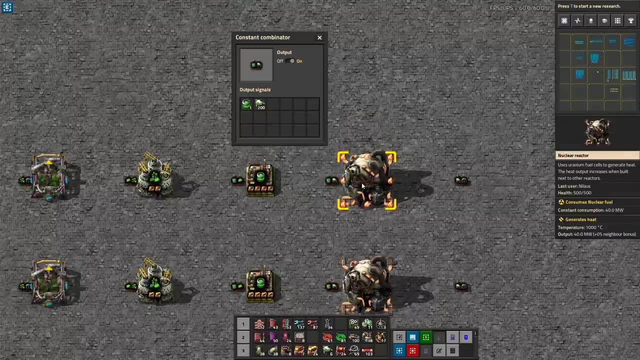 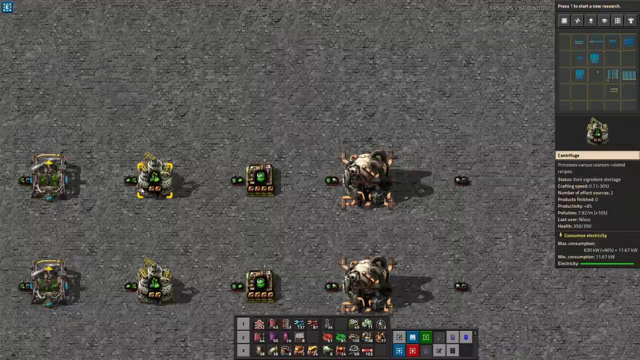 one uranium fuel can support 200 reactors. one uranium fuel can support 200 reactors because this one only consumes it once every 200 seconds. so this is a very large ratio in one direction. this is a very large ratio in the other direction. when we then start combining it and saying: how many mines do we need in order for? 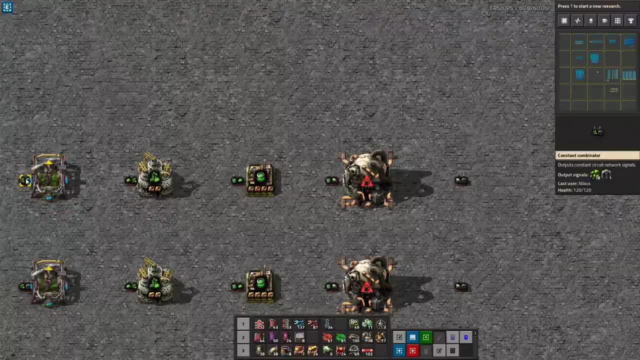 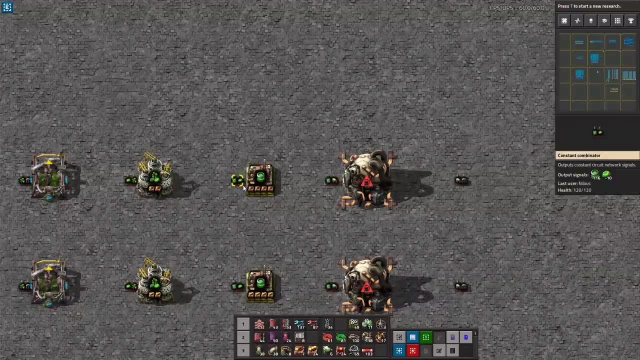 when we then start combining it and saying: how many mines do we need in order for to generate enough? if i put these 18 per minute in here and reprocess it, then it's going to be a very low number of uranium. it's going to be a slightly higher number here, but then this one isn't really. 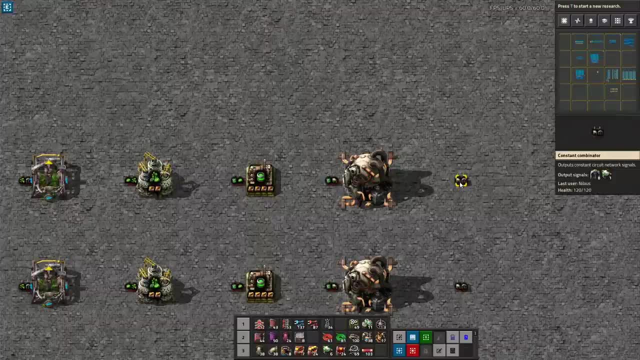 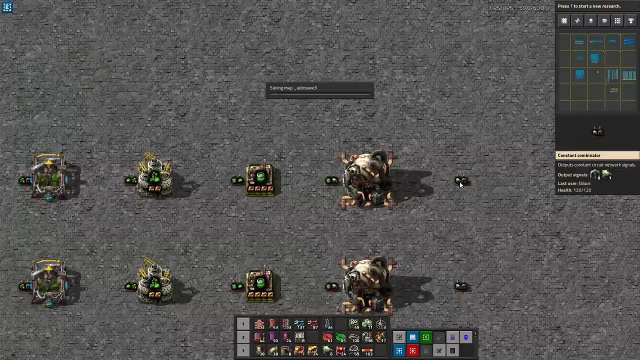 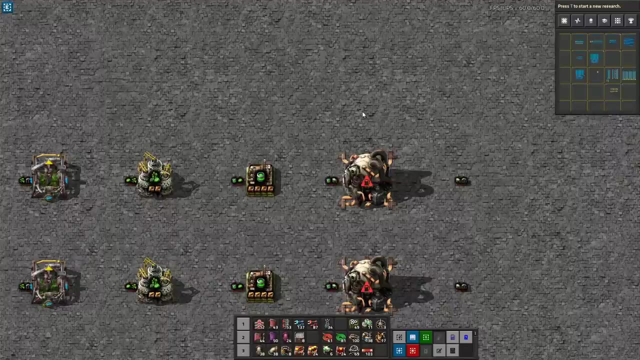 consuming a lot, and the answer is, surprisingly, eight, eight miners. technically even it's 7.6 miners and support one nuclear reactor. i guarantee you, you, unless you were in a nuclear reactor, you weren't to our workshop. you did not see that coming. so when you tap your first uranium, uranium or 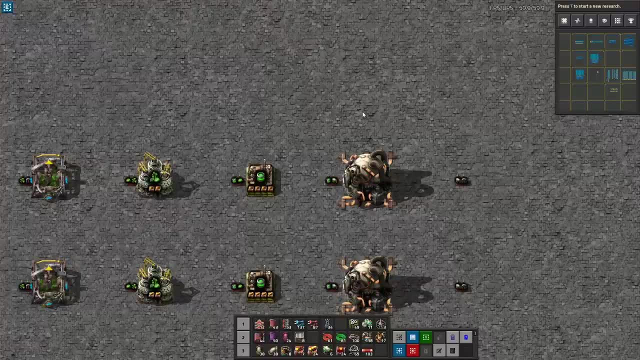 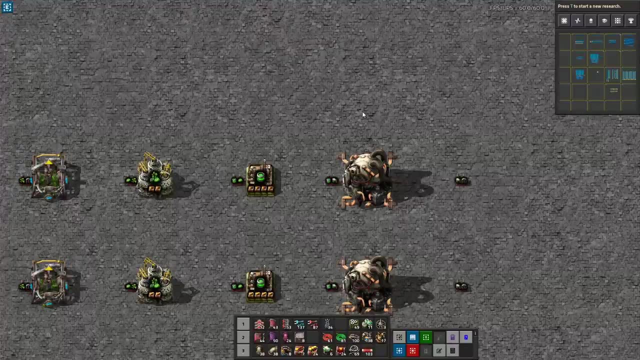 patch and you put 50 miners there even without having the cover x refinement process, you can easily support, you can just go. okay, if you put 50 miners down, you can support eight nuclear reactors indefinitely without a cover x refinement process, just from the random chance of getting these. 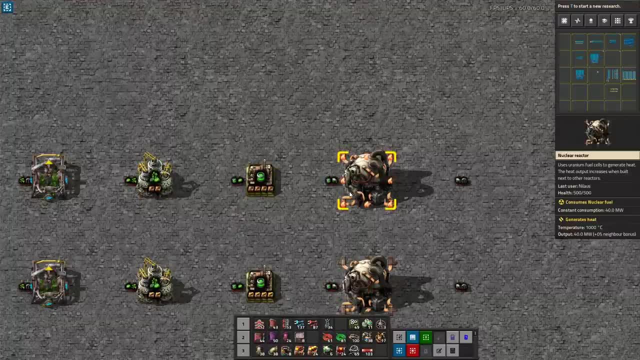 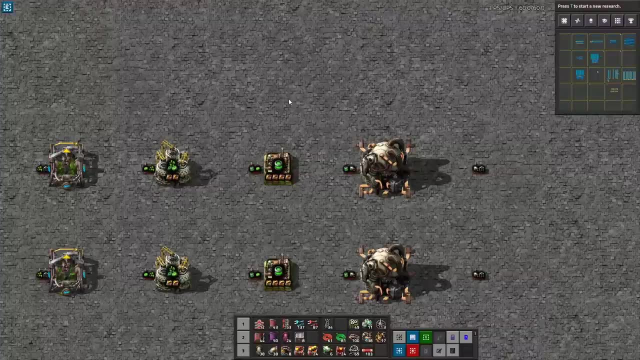 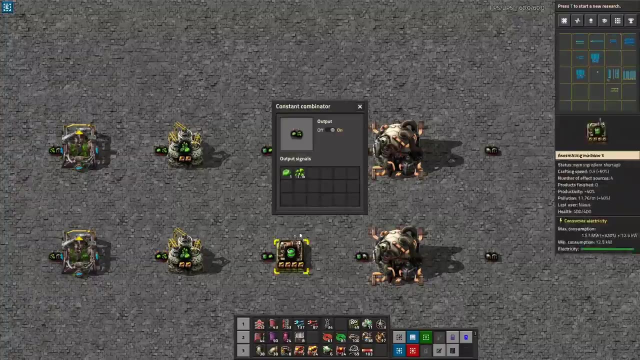 with productivity in these two locations and i think that is absolutely amazing, absolutely amazing to to be able to do that and i will. i've even done sort of a second calculation where we assume that higher productivity it changes the numbers slightly. this is now less we need because we get. 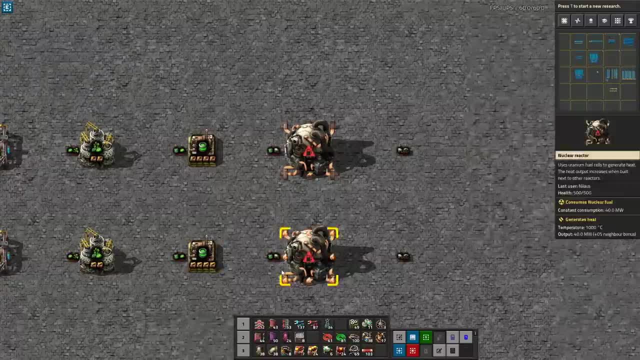 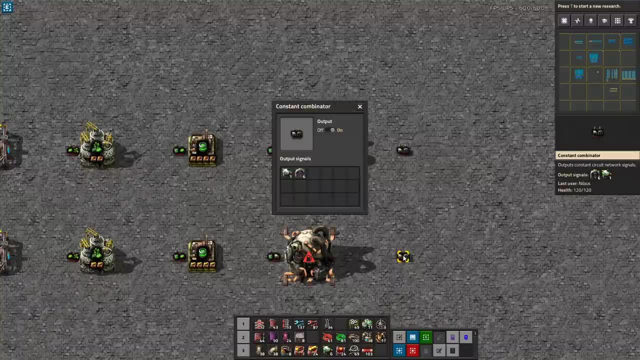 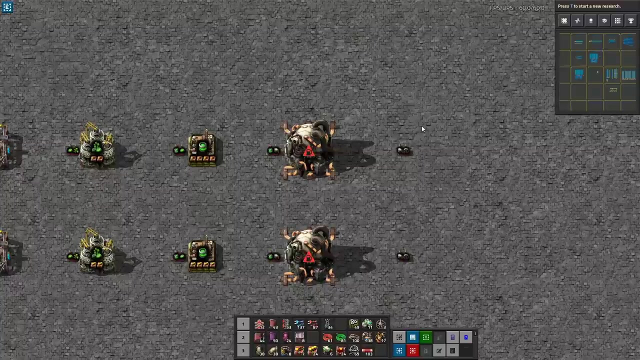 more productivity. this is, we're getting higher yield because more productivity, and in this case it's six, or it's actually five point six, six or six, seven miners to feed one nuclear reactor. of course you can then argue that, yeah, but i also want my nuclear fuel, nuclear fuel for trains, and i also want my to drop nukes on the biters. perfectly fine, 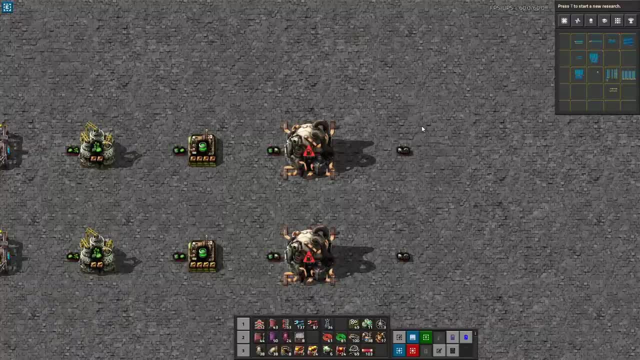 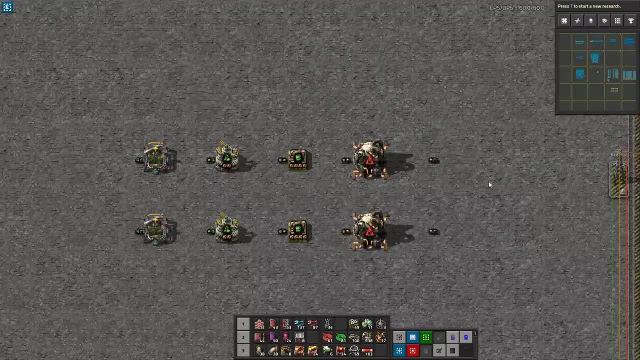 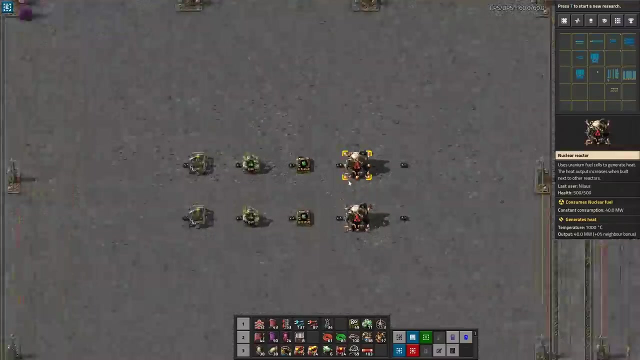 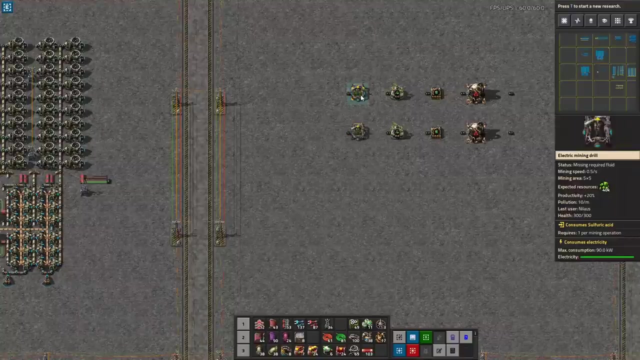 but don't do that until you have over x up and running, because that's basically infinite uranium. so what this means is that it is incredibly easy to support your first nuclear reactor off. you can, just if you built your first nuclear reactor or your first nuclear setup like this. you just need when it reaches a steady state, of course. 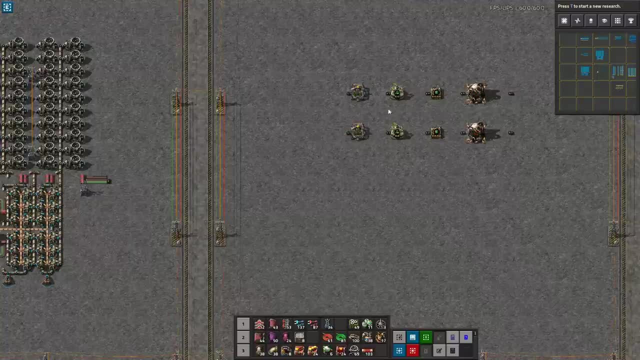 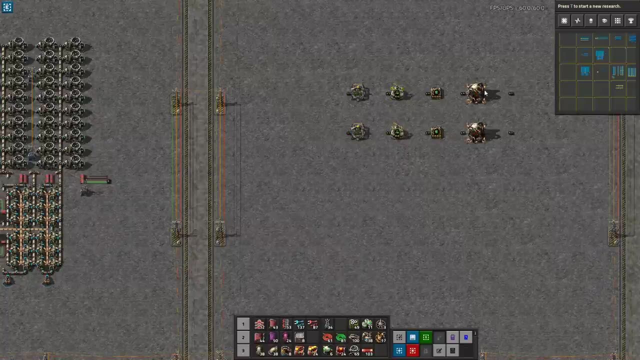 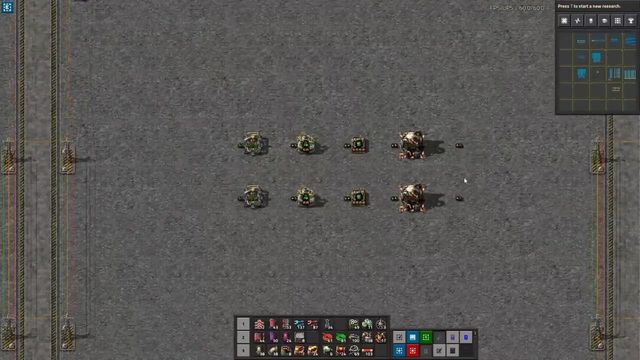 24 miners to support the full thing, which is very, very low. so keep that in mind when you look at a uranium patch and consider whether you with, whether you can support it, whether you should wait for nuclear until you have coverage. i see a lot of people who kind of wait until. 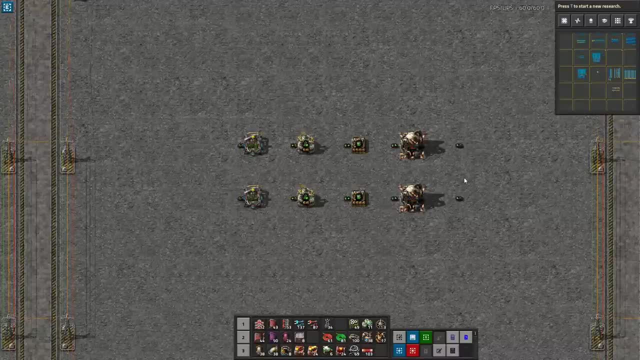 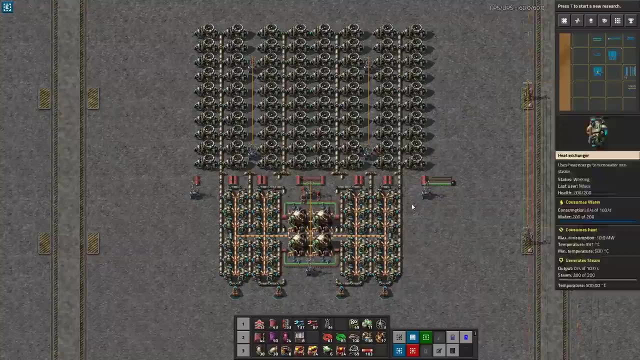 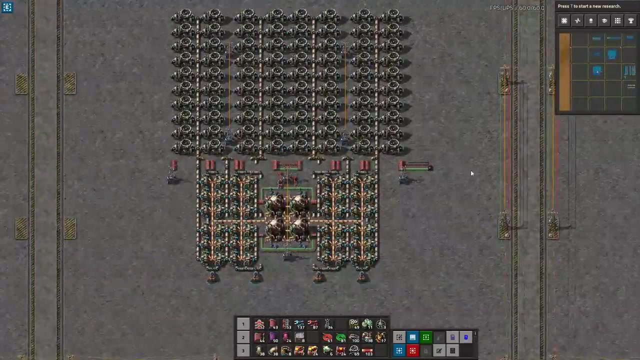 you have cover x or rush the cover x process in order to get the nuclear up and running. that is not necessary, and i hope that this little calculation proves it to you- means that this one can be built at blue science instead of waiting until purple science and even then a very expensive purple signs. this also means that- and this is now, this is 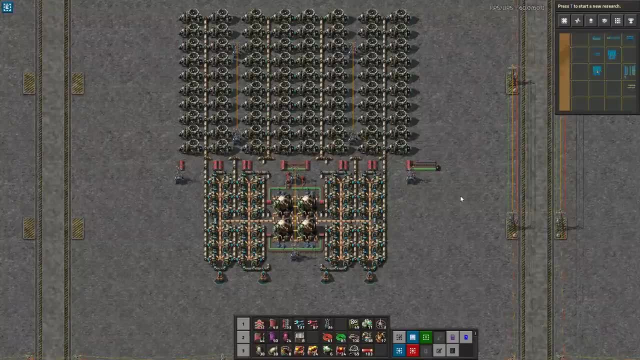 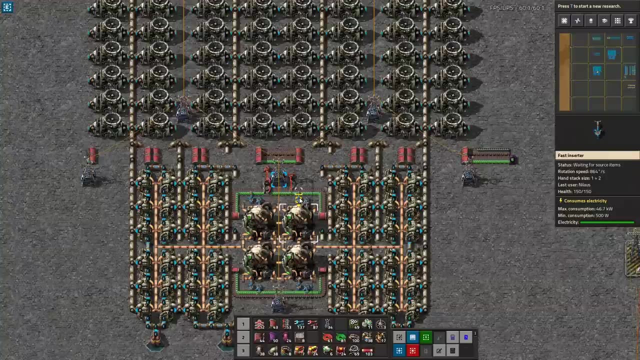 the calculation i'm going to use as my argument for why you shouldn't do steam storage. you can build steam storage which makes this build larger, and then you can put wire conditions here that don't put it in on when their steam storage is, until it's less than. 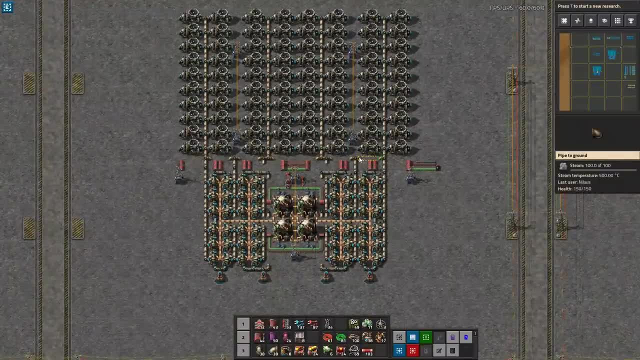 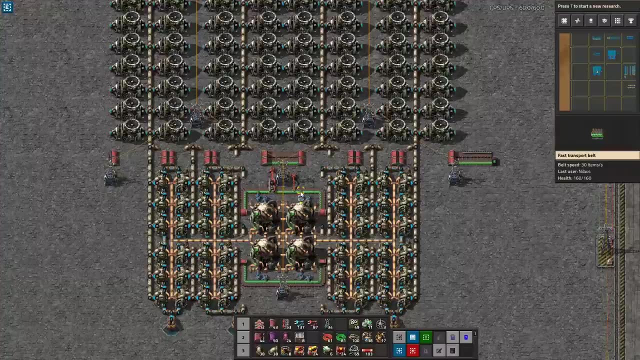 something. so you store the steam. steam doesn't lose any temperature when it's stored. for some reason, that's just the way it is. so if you build steam storage, you do that to save on the uranium, and my argument is: you don't need to save uranium because it is so ridiculously abundant, even. 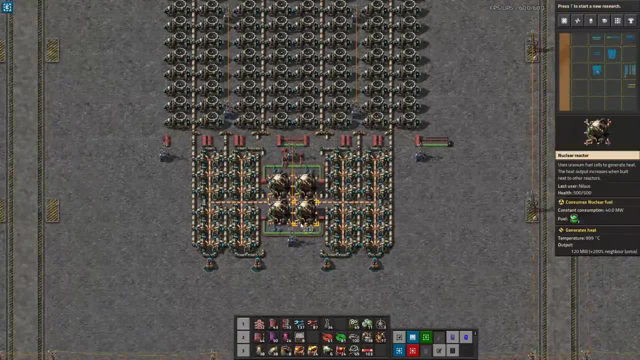 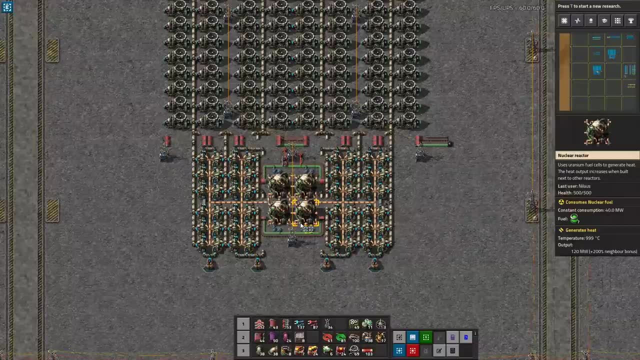 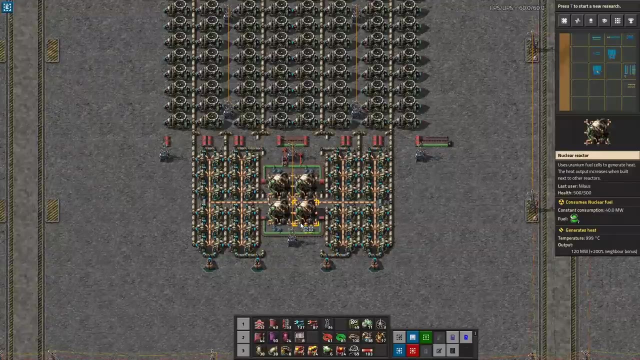 without coverx, that you don't need to go into the hassle of putting up advanced circuit networks. you don't need to tax your your setup with steam storage, because fluid mechanic fluid calculations are some of the heavier ones, so you really don't want to just have a lot of tanks balancing liquids. 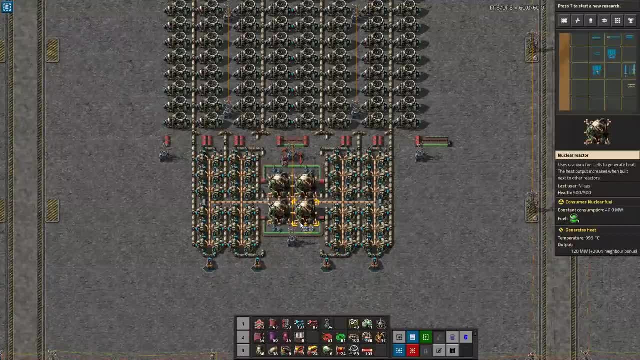 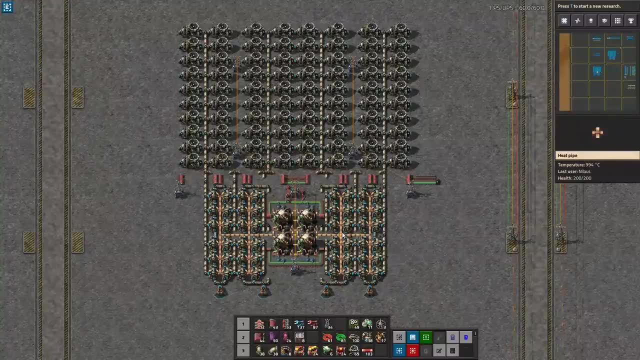 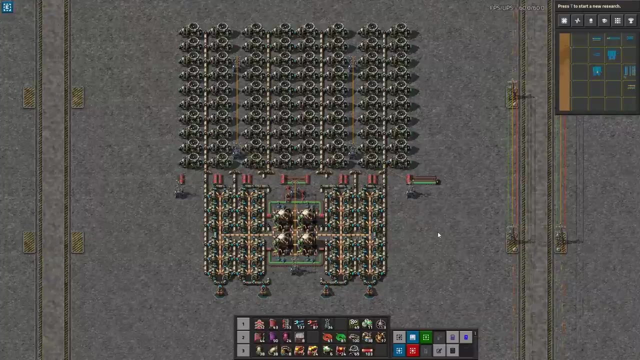 all the time doing that calculation all the time, in order to save a resource that is so abundant as uranium is. so that's, that's why scrap all ideas about steam stores. you can do it if you feel you really want it or if you happen to be on a location that has very, very, very little uranium. 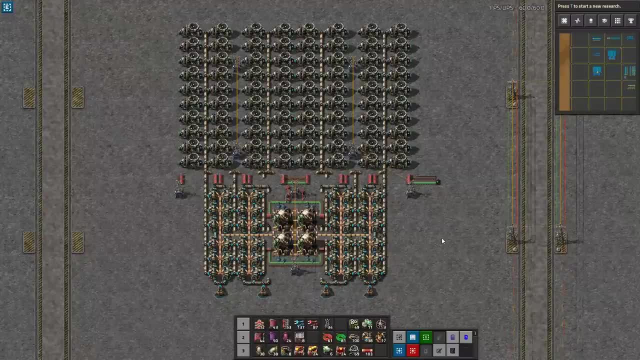 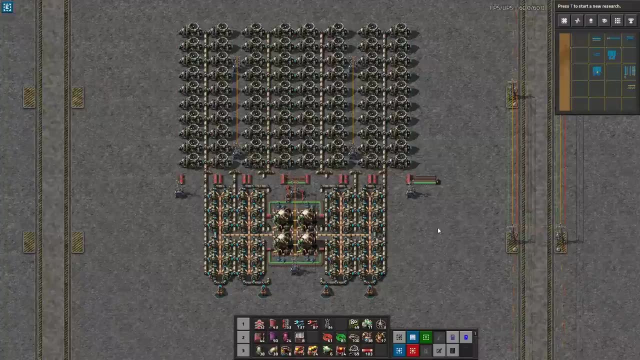 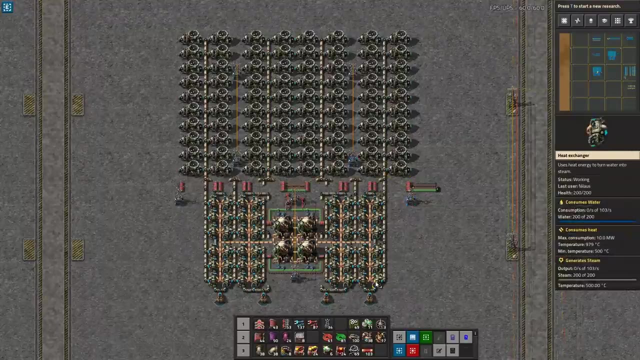 but if you have a normal world with a uranium patch, if the first uranium patch is a million, don't worry about it, don't even bother with steam storage. it is completely wasteful. and the other argument, or the other part that i wanted to talk about was was whether it's better to build. 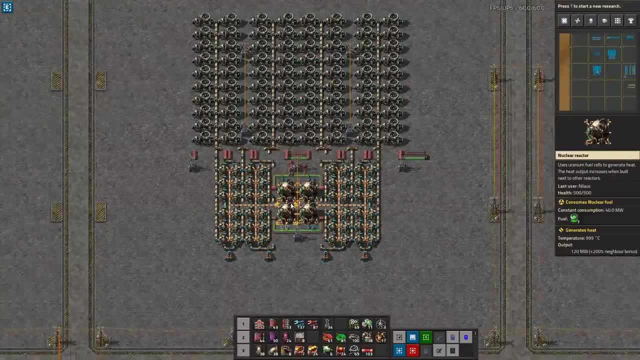 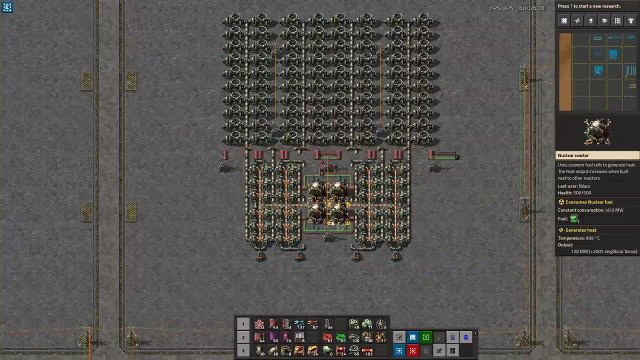 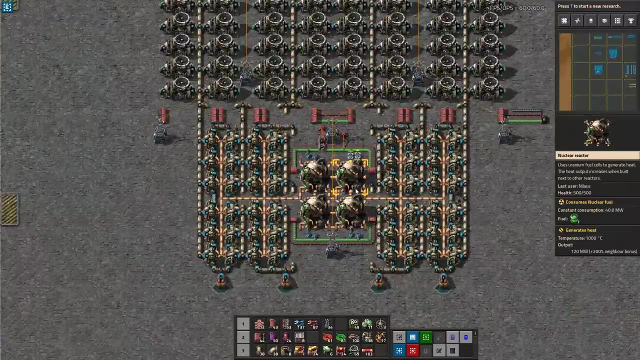 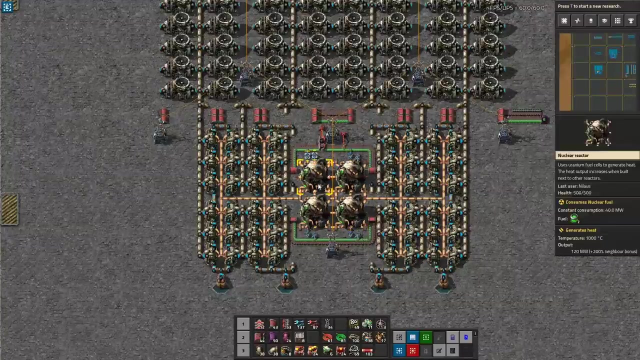 a bigger setup than this. now, my argument is no, and i'm gonna try to explain it. if you look at the power, if you look at this one, the neighborhood bonus is basically what? what are you getting for the neighborhood bonus you're getting? what is the point of using, let's say, a two by three power instead? well, you're going to. 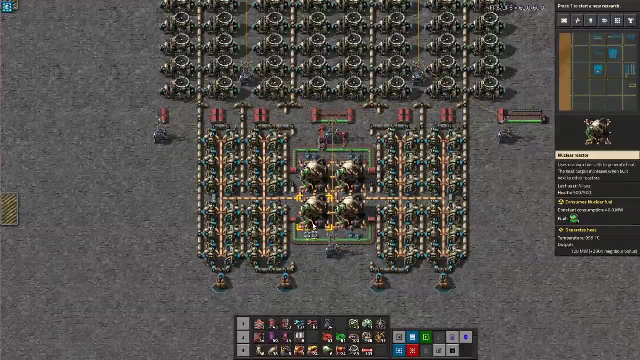 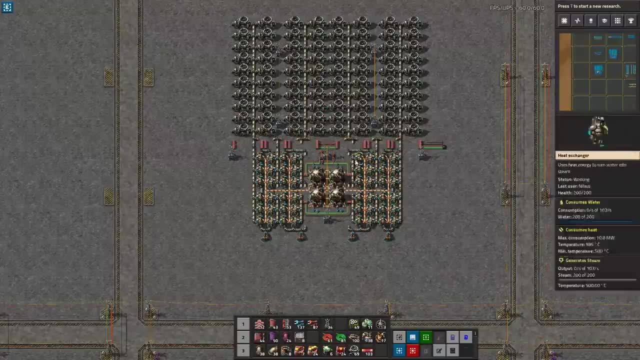 consume 50 more fuel, but you're going to get more power out of it than the 50 extra fuel that you're consuming. so building a bigger nuclear power plant and like a two by three or two by four is going to be a lot of work, but you're going to get more power out of it than the 50 extra fuel. 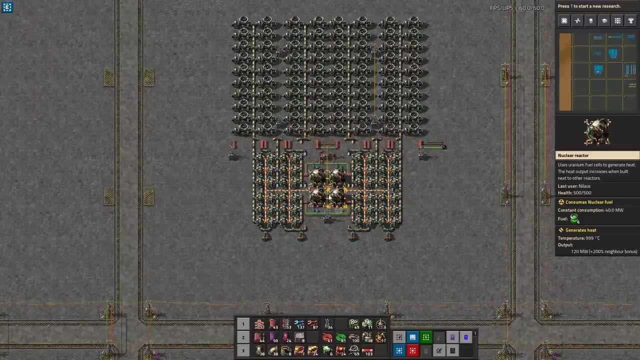 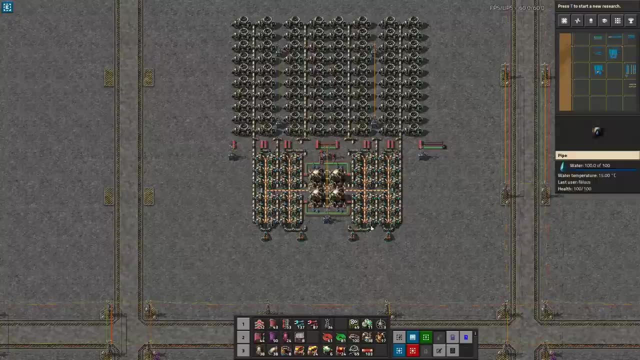 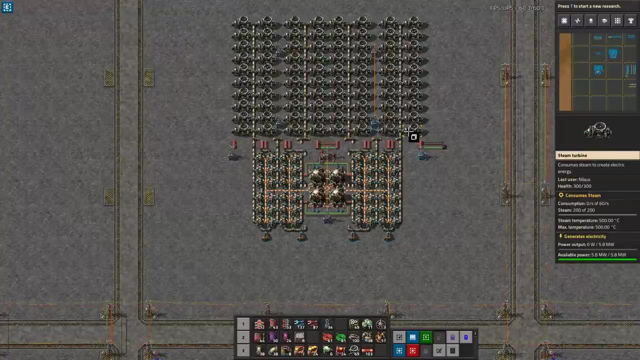 is going to your. the only purpose of that is saving nuclear fuel, because the size of it scales with the power output, because the majority of the space i'm using here is base is on this part. so you're not going to save any space by making it bigger, quite contrary, because you will have all 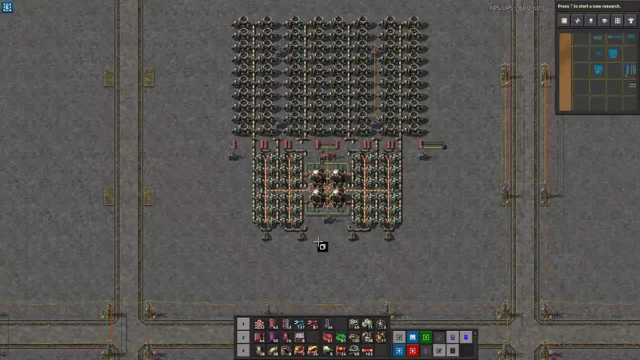 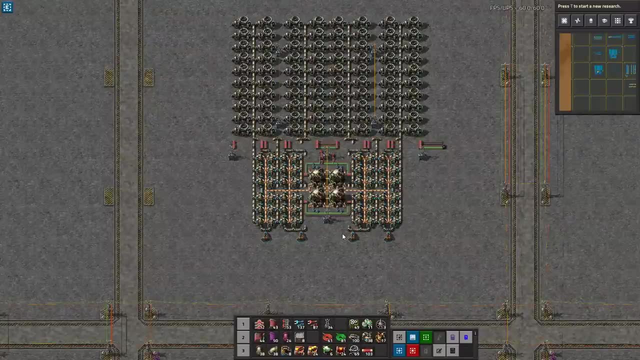 sorts of issues with getting the water in and making sure that the flow is correct, and it's way more difficult to design a two by eight or a two by two by two by four or two by five design, and i see a lot of designs being touted as great. 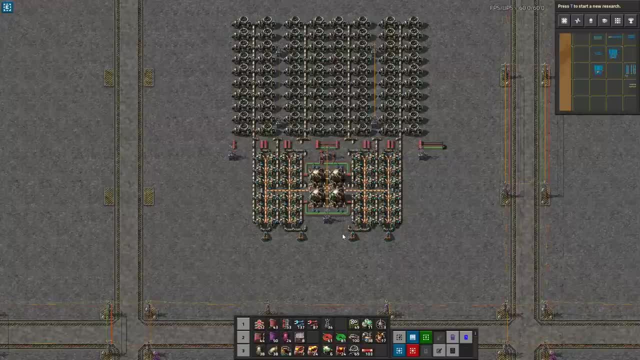 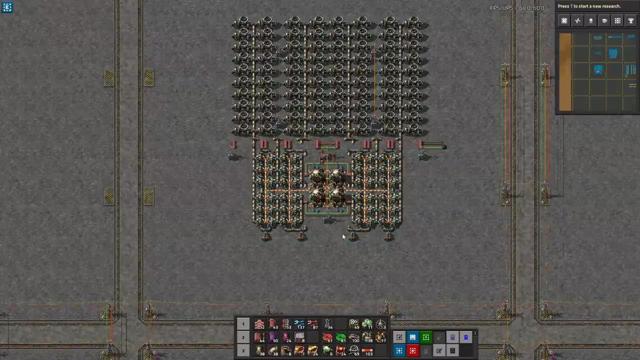 and i can just look at them immediately, like there's problem with water flow, there's problem with steam flow, there's problem with heat flow. it is not easy to assign those big ones so that they work at peak capacity. that's really important if you build something that that only works at 60. 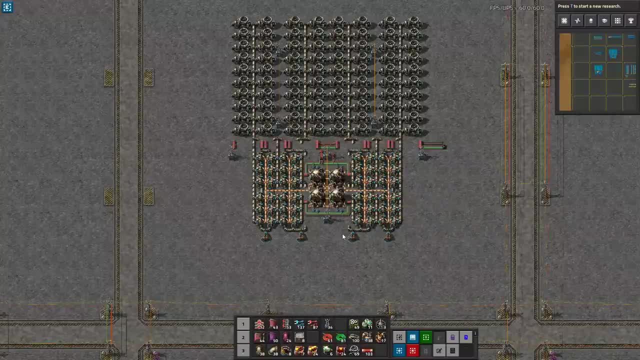 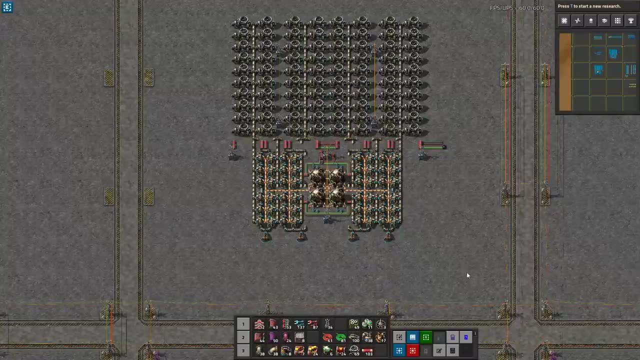 capacity, you are fooling yourself. i would highly recommend: if you are not an absolute master on designing these, don't do it. if you're not an absolute master on designing these, don't do it. it's just not worth it. so i'm adhering to this design because it does all i need to do and the 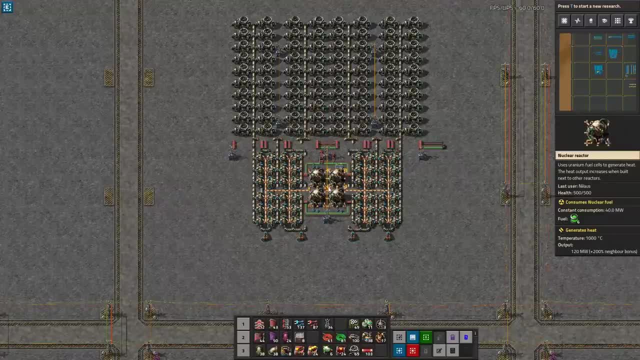 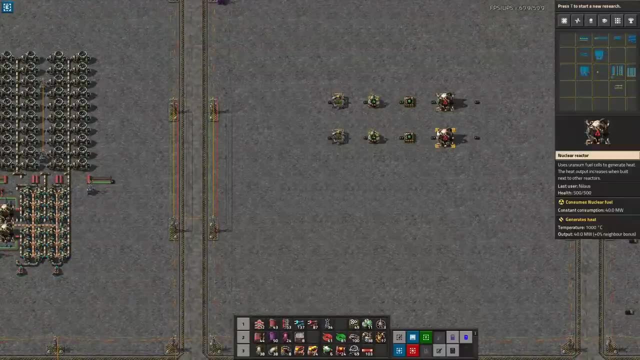 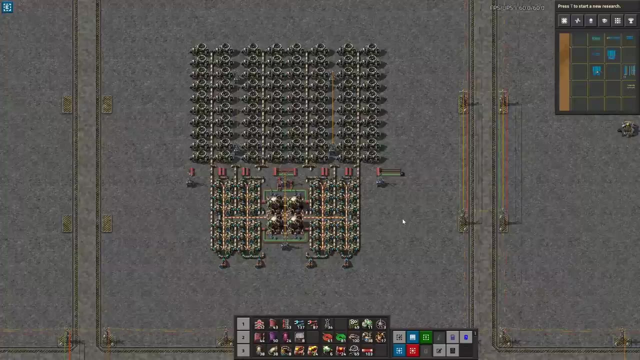 only reason to build it in a bigger configuration here would be saving nuclear fuel, and i've just shown to you that nuclear fuel, even without cover x available, is a non-issue. it really is a non-issue. and as soon as you have the cover x refinement process, you will have all of the nuclear fuel, all. 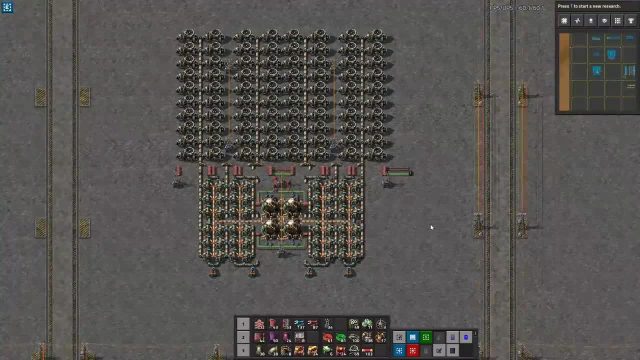 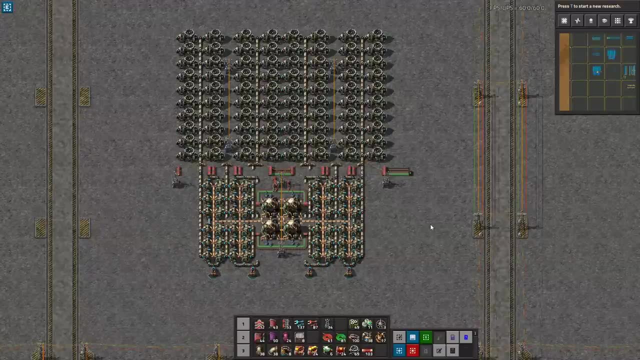 of the uranium 235, just to make sure that you have all of the nuclear fuel, all of the uranium 235 you could ever dream of having. so that's a bit of a controversial opinion. that do not bother with steam storage and do not bother with nuclear power plants larger than two by two, they're fine, rather. 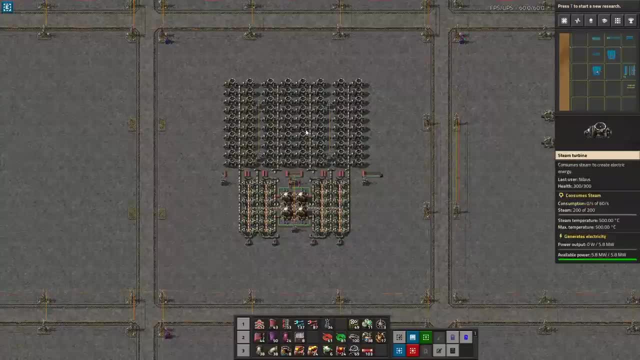 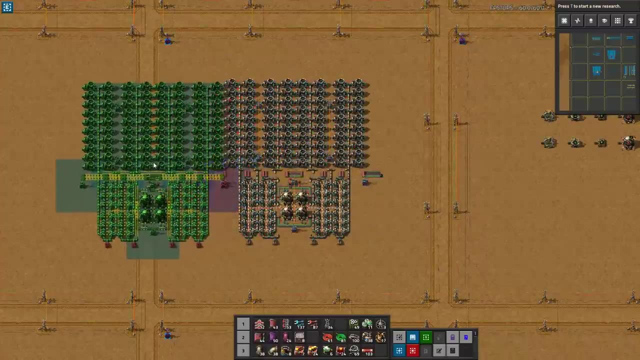 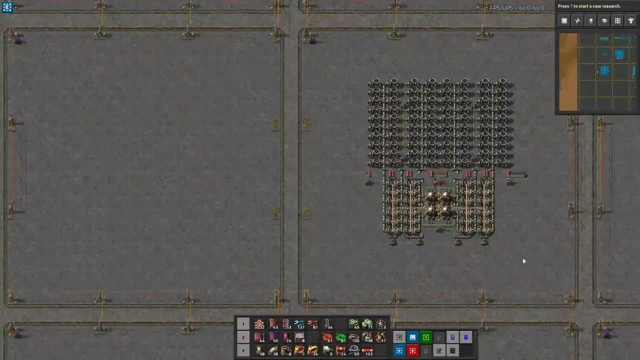 build a nice design and then stamp it down next to each other. this one is fairly quadratic if you look at it, so it has a tiles. really well, go out here. if you have landfill area, you can just make it like an l or something where you can drive, drag the water from, and yeah, it's going to be just just. 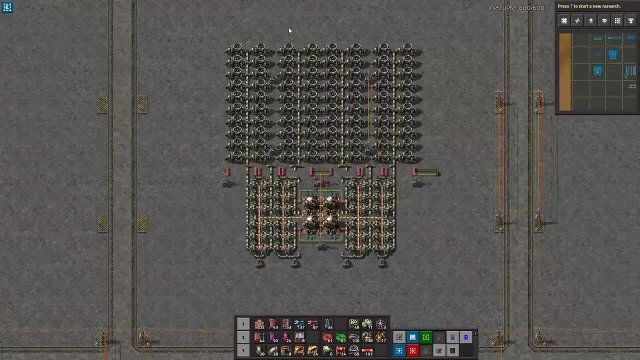 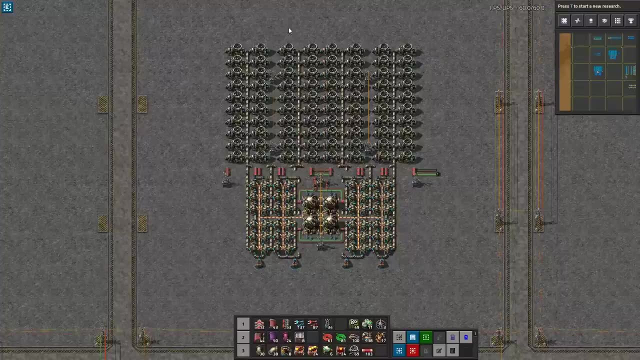 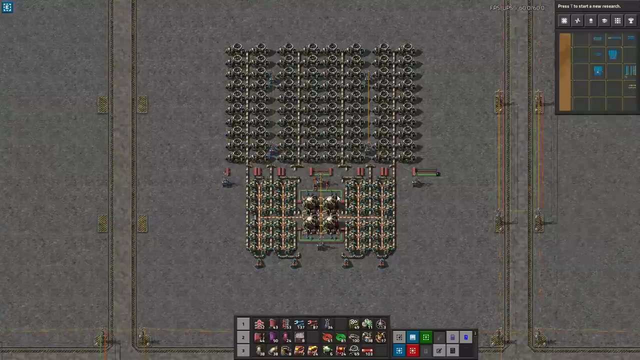 fine, and there you have it. you have a nice, clean, four by two by two nuclear setup, easily tileable, easy to build. you have the arguments why you don't need steam storage, why don't need bigger ones, even though they are slightly controversial. i hope that i have persuaded you to uh, to see the 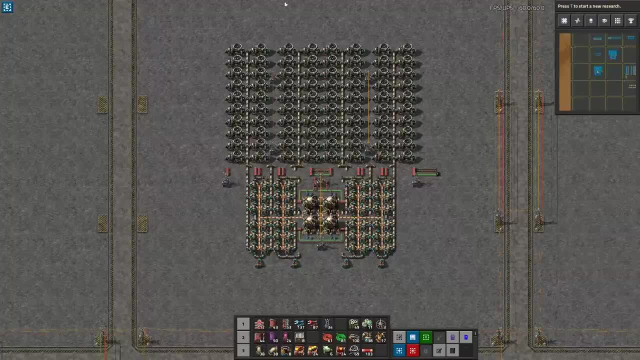 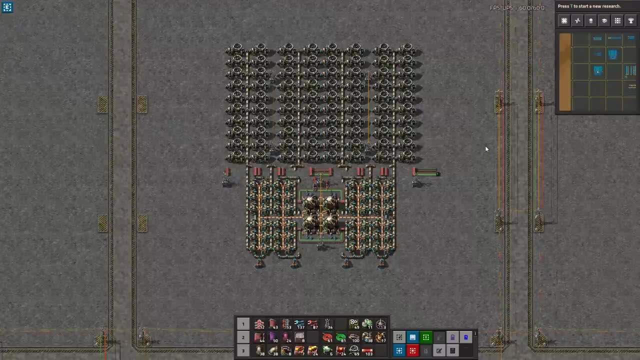 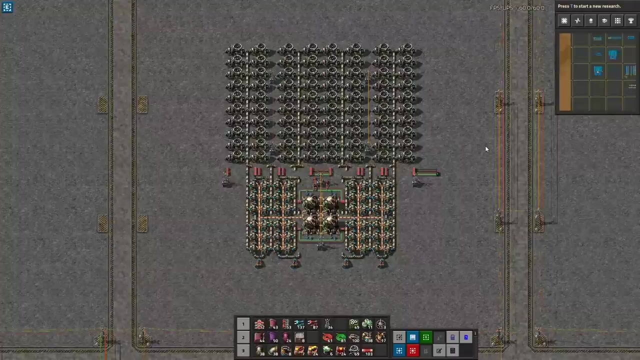 light of why this is the case. this has been double checked. all the math has been double checked by about 200 people when we were designing and building this over on my twitch chat. so if you want to be part of the design process and debugging, and then i'm, i have these factorial 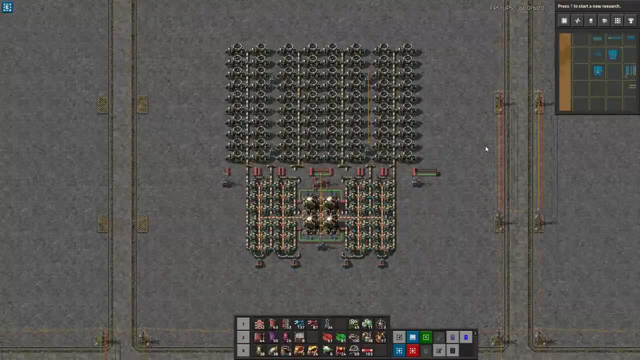 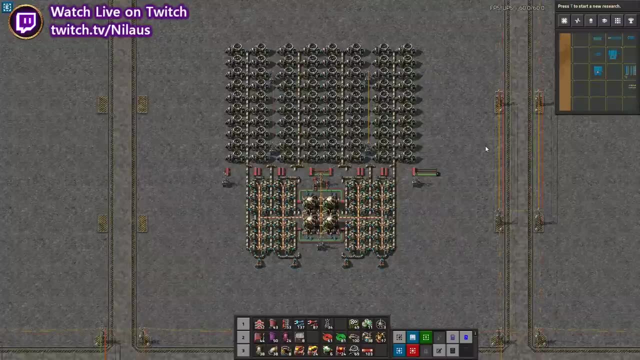 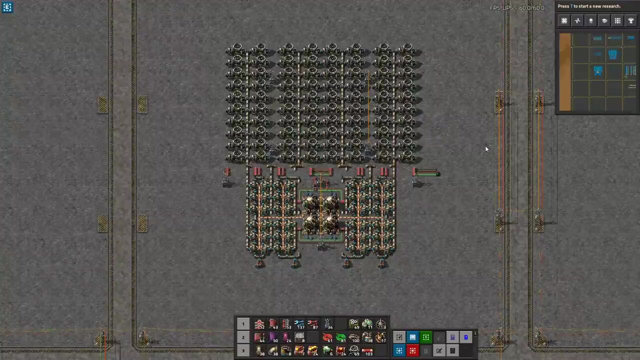 workshop sessions that i'm conducting usually on mondays over on my twitch channel. this is twitch tv, slash nilaus, and it happens usually at 8 pm. i'm also streaming other let's plays- it's tuesday, thursdays and sundays on my twitch channels- and just come on over, hang out. it's really cool. 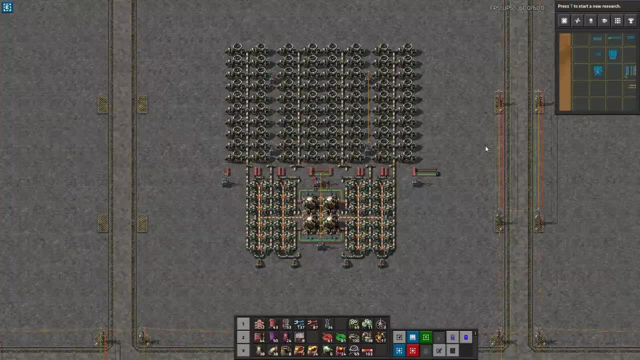 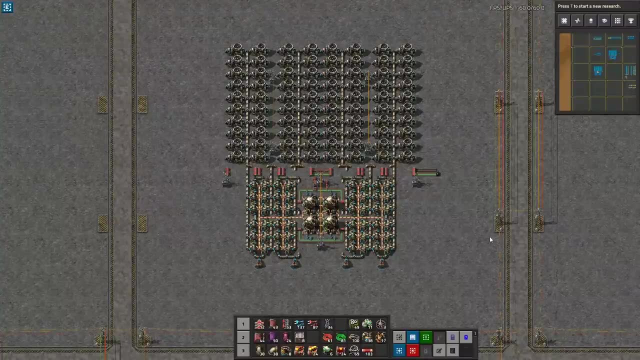 and we do some really nice designs and i'm always learning new stuff when we are, when we are designing, designing these builds. if you like this series here on youtube, this master class series, then consider liking it. that shows me and the youtube algorithm that it is a worthwhile video. 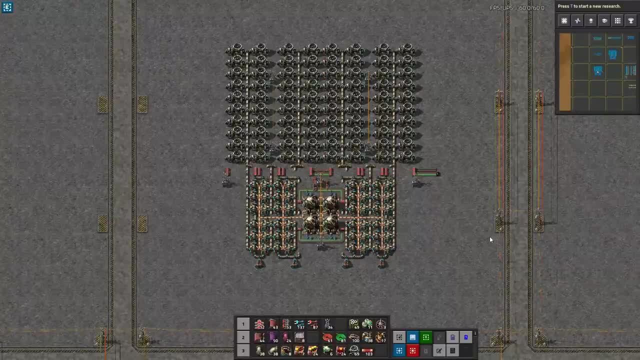 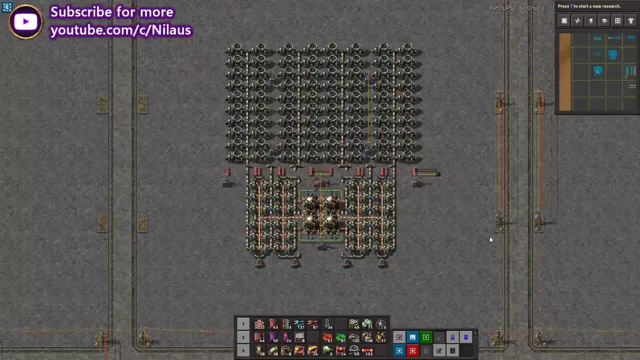 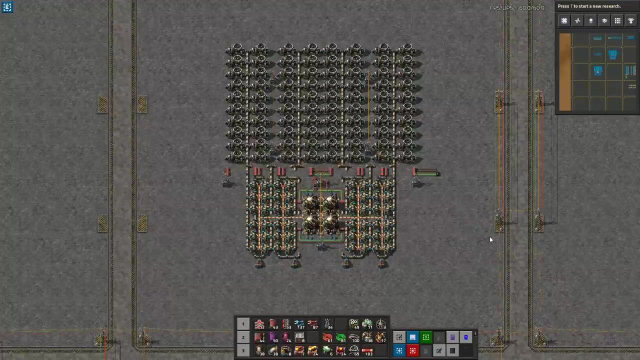 to watch. also, if you haven't already and you like the content produced, then consider subscribing. i hope that i have earned your subscription. we are close to the 50k mark and maybe even over by the time this one goes out, and but there is a. there's still room to grow, and i see that it's only. it's less than 50 of the. 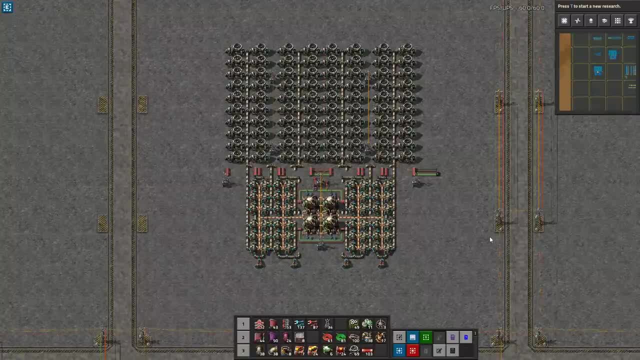 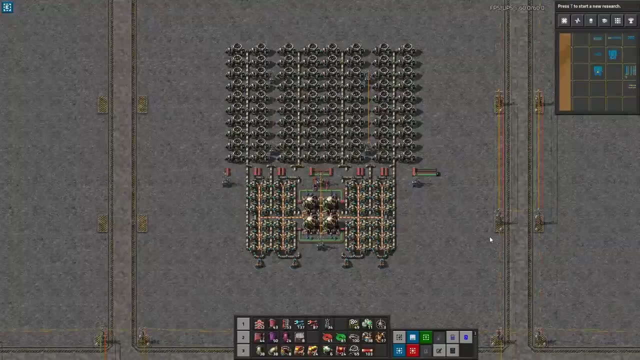 viewers on the channel who actually subscribed, which is a bit puzzling, but so be it. so that's why i have to earn your subscription. thank you very much for watching. it's been a pleasure doing these for you. i hope you have been entertained and educated and i'll see you guys around until. 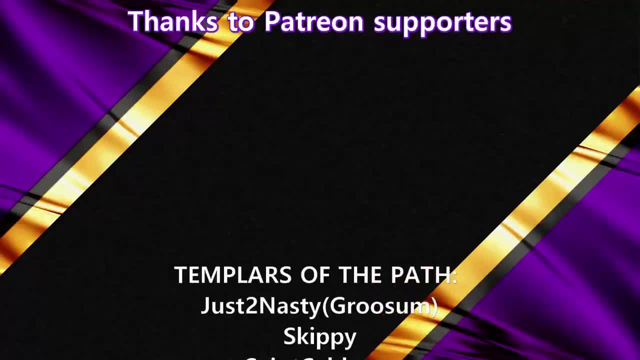 next time stay effective, you. 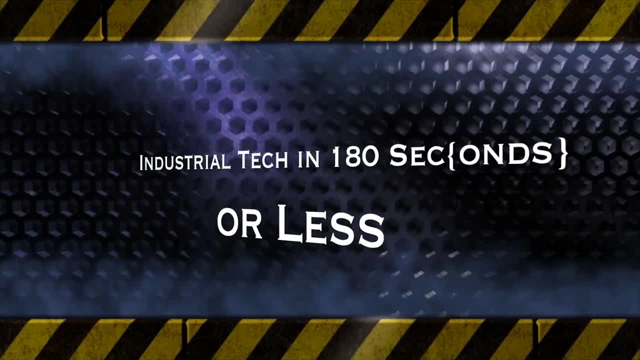 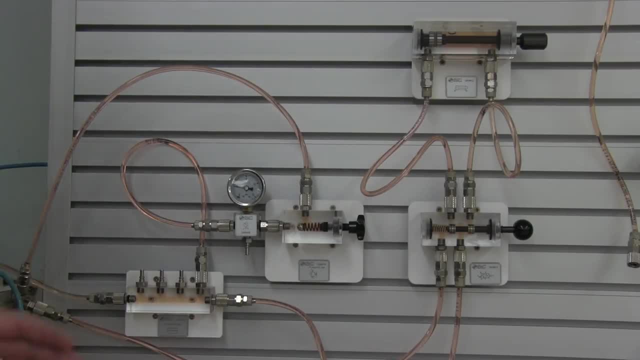 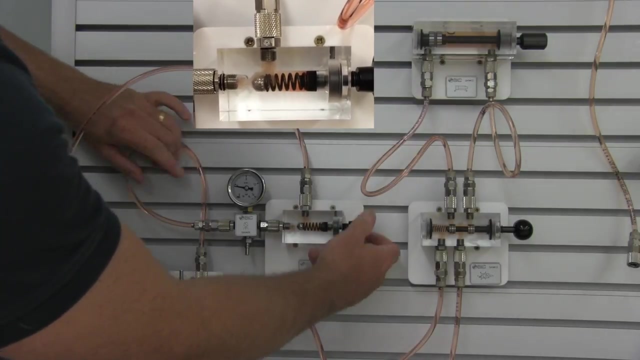 Okay, in this video I want to talk about a very basic hydraulic system. So I have, from my pump I'm running to a manifold with a number of quick disconnects on there. One of the connections from the manifold is being used to go to this very basic pressure relief valve, which I can adjust.